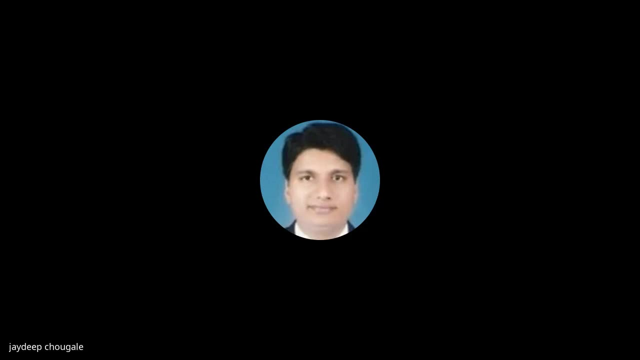 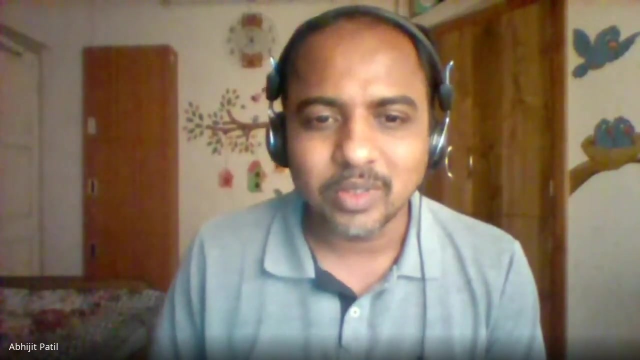 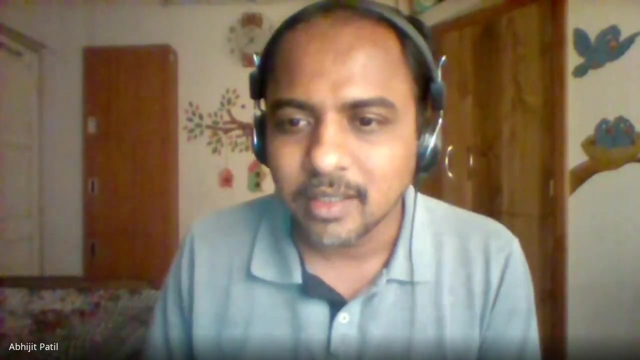 etc. So welcome, sir, and guide to our students, Thank you. thank you very much, Jaydeep sir. So, without wasting more time, we will directly start with the topic. I will share my screen. just let me know if it is visible. 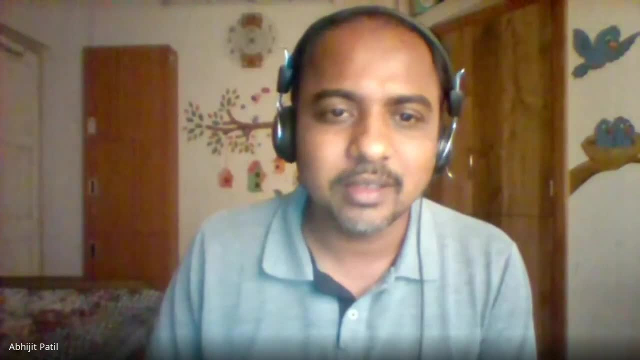 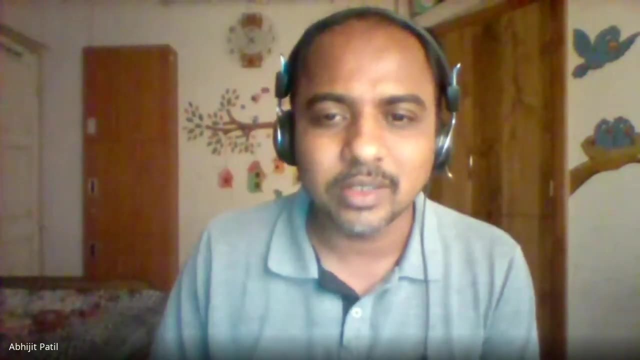 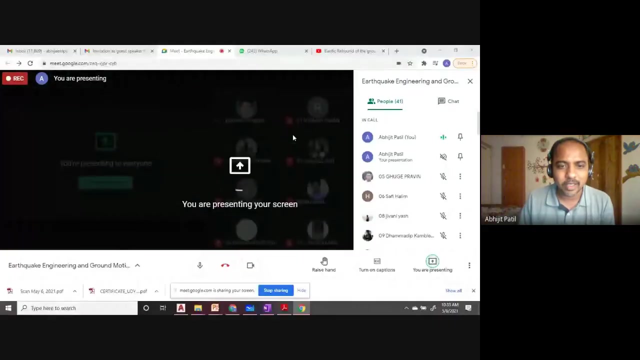 For students. it can be interactive session. So if you feel to ask something or if you feel that it need to be any point need to be elaborated more, you can interrupt me and we can discuss that. Yes, sir, the screen is visible. 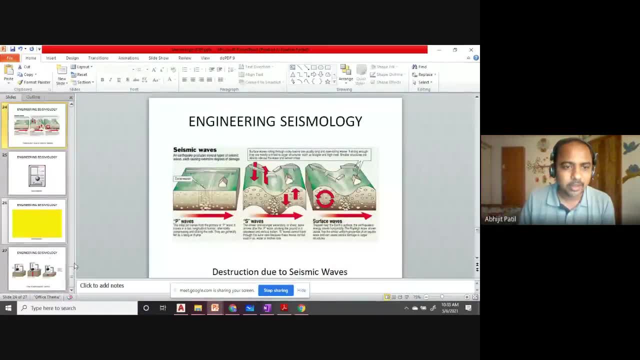 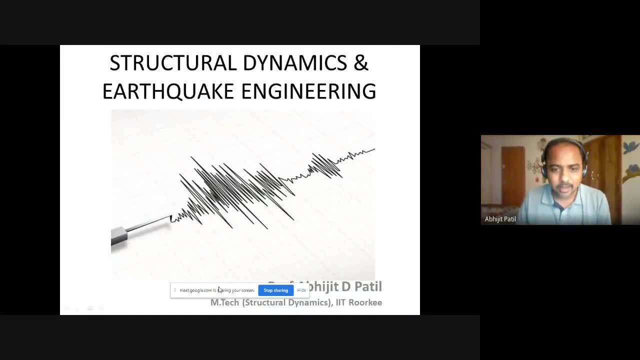 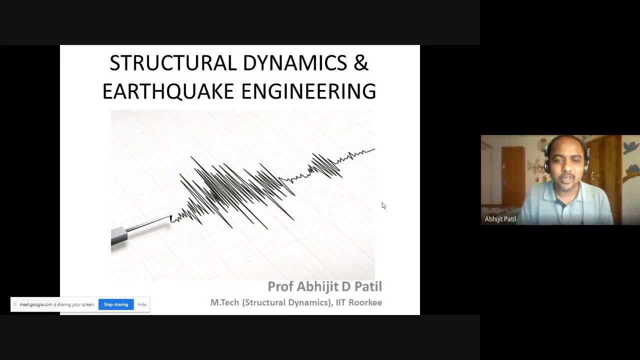 you will be able to understand what exactly is this image. So we will. basically, I have decided a flow, I have gone through your syllabus. So we are given the Phone, then we are given the data. Okay, we will discuss seismology. that that will why we need to discuss seismology. we need to discuss 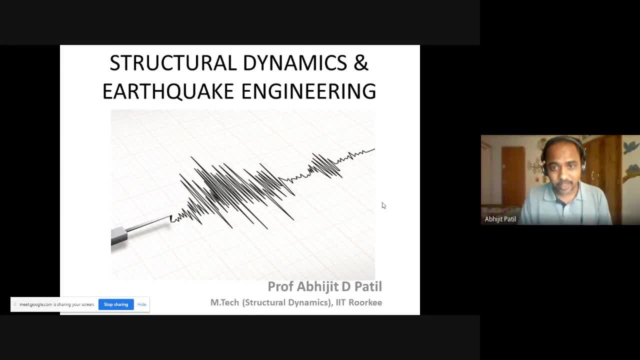 the exact reason or cause of earthquake and what are it, its effects inside the earth, and then we will see what is it, what is its effect on structures. so, once we understand this- although there is no structural dynamics part in your syllabus, but quickly through one or two short- 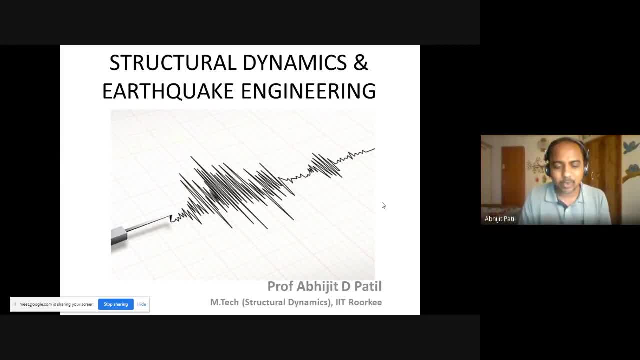 videos i will try to explain the concept of structural dynamics and once you understand that, then the numerical part. that is, how the- or you can say, the application part of what, whatever we will be discussing how the earthquake force on a building is calculated with the help of numerical. 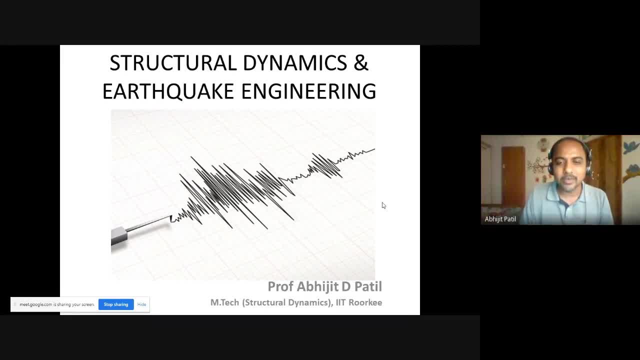 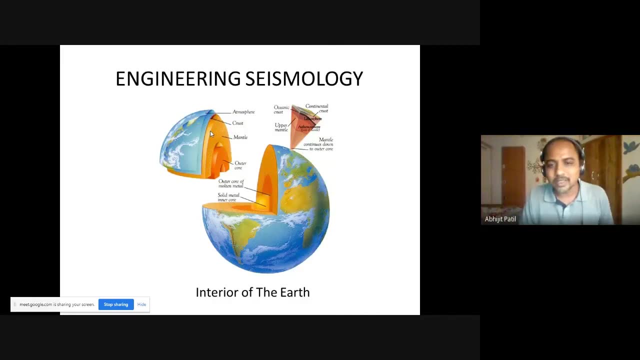 we will discuss that and, if time permits, i will shortly cover the ductility provisions. okay, so this will be a general flow of the lecture. so we will start with seismology. so most of you in school physics must have seen this image, okay, so basically, this is a section through interior of the earth, so you can see. 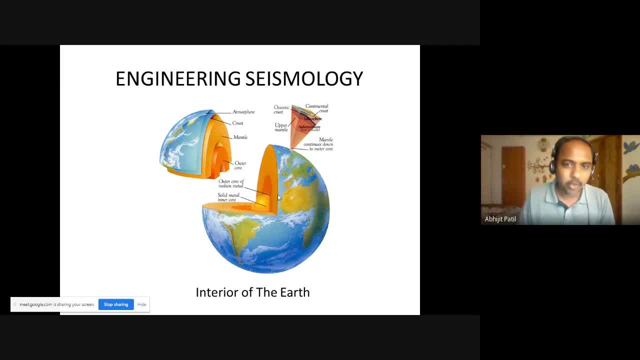 this. can you see my mouse pointer moving? yes, sir, okay, okay, yes, sir. so starting from the top, if you see. so, this is the atmospheric layer. so we know that earth is surrounded by atmosphere and because of which we live, we are in this atmosphere. oxygen is present, so that is why. 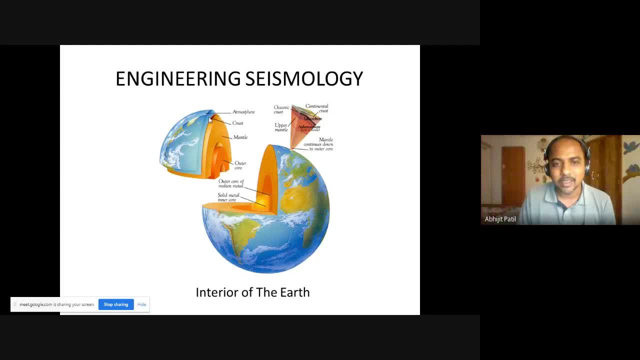 we are able to breathe and the living organisms are present. so beyond this atmosphere, there is void space. no air is present, right? so this is a small layer, then you have a thin crust, okay, so here you can see that thing. we will see the image in detail. 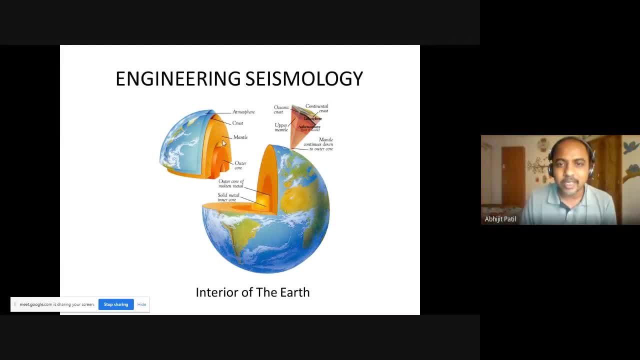 here you have that thin crust. below that there is mantle. again. that mantle is divided in upper and lower mantle. then you have outer core and inner core. okay, so this is a typical interior of the earth. now, why are we discussing this? because we are moving towards what causes. 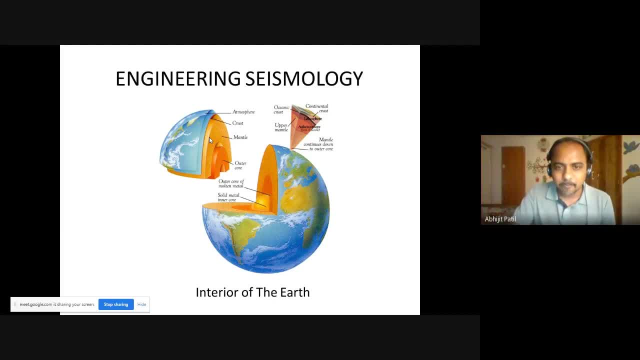 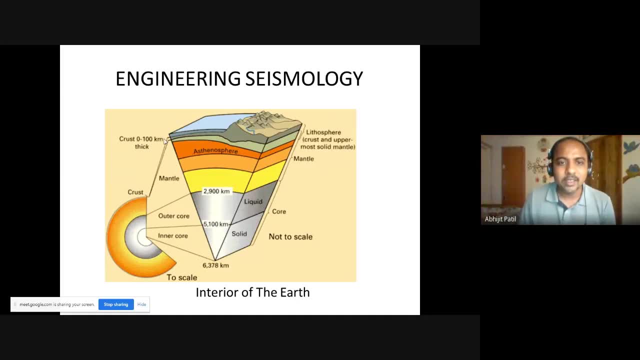 earthquake. so for that we need to understand the structures. so this is a zoomed part and it has many light sources, it has several volumes, like our sun, oh, apple trees, great illuminations, comes in different colors, and this entire rude area where we want to live and yet we keep finding some interesting defter κiler, the more we могут чувствовать. 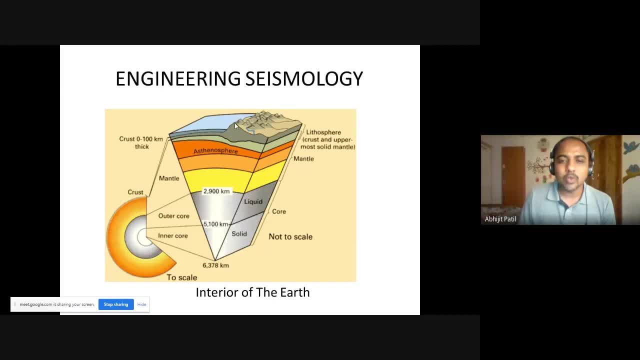 don't worry, I will not put this too deep. there is a lot more facilitate. well, there may be that particular. so we get to try and Fit policy modelici n werner, 10 words. there is another personality and few more details. so you can see, this is the cre. 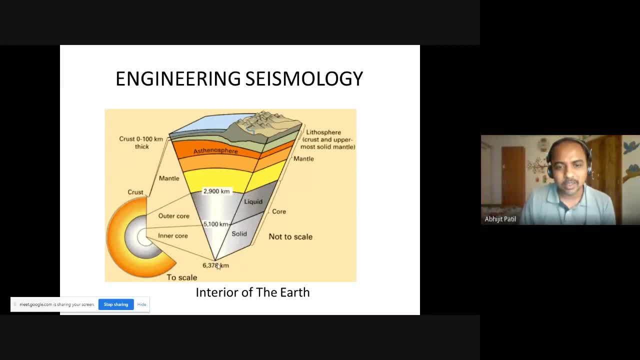 so the thickness of the crust is around zero to 100k of the earth. it is around 6400 kilometers. okay, so as compared to that, hundred kilometers is nothing. it is just like peel on the orange, so it is as thin as that. then you have asthenosphere here. so crust is typically- we know it is- a. 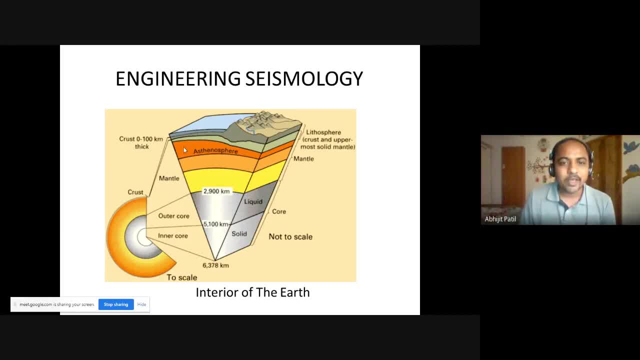 solid part. okay, then you have asthenosphere. it is a part between. it is a transition part between mantle and crust. so crust is solid, mantle is semi solid. so partly liquid, partly solid, basically whatever you may have seen in movies or if you just google the volcanoes. so during volcanic eruption, 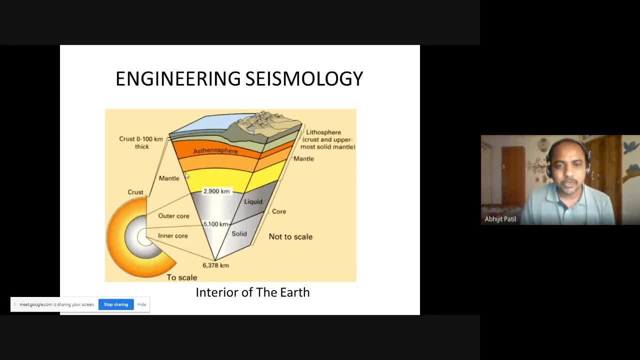 whatever comes out that we call as lava, so that lava is in molten stage here. okay, and in between, this asthenosphere contains viscous matter. so if you try to understand the way, you must have studied fluid mechanics. but we discuss it just like fluid or viscosity. it is a property of fluid which 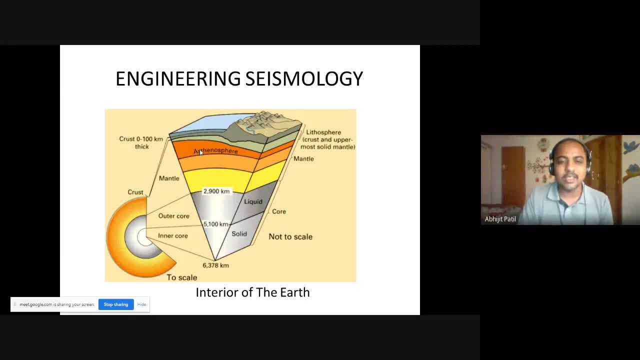 resists the flow. so water is not viscous at all. if you just drop the water, it will just flow away. wherever it gets the lower direction, okay. but if you take an example of oil, okay, lubricating oil. so if you pour that, of course it will flow, but it will not flow as easily as 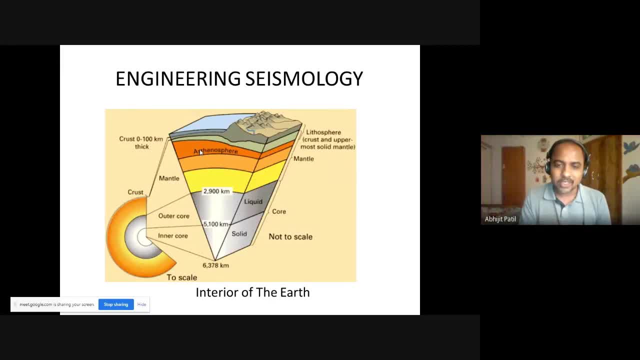 water. okay, so this is called as viscous fluid. so asthenosphere contains the molten rocks. okay, so these crust contains rock, asthenosphere contains molten rocks, but these are not in liquid form. these are in viscous form, semi solid, you can say, or semi liquid. and mantle contains the liquid form, again you. 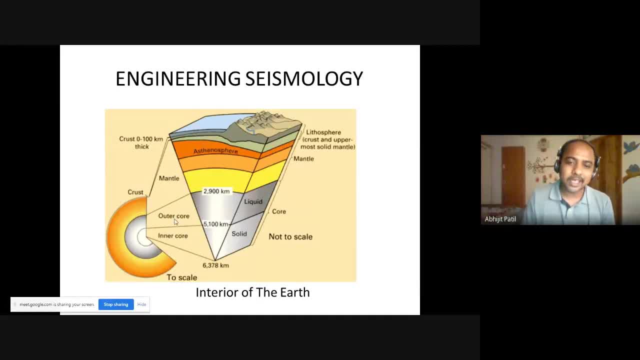 have outer core and inner core. so outer core is again at a distance of 2900 kilometer to 5100 kilometer. so this is in liquid form, the outer core, and inside we have so around 5100 to 6400. so if you calculate the radius is. 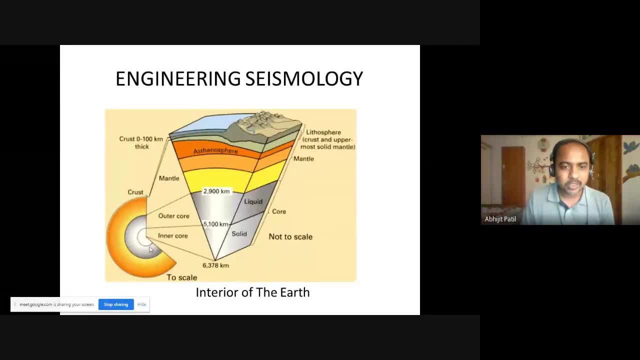 around 1300 kilometers. so this 1300 kilometer radius. we have inner core which is very solid for, say, let's say, Lagoon upstream, this happens and reach only св при and it contains mostly iron. that is why this magnetic field of earth is present. 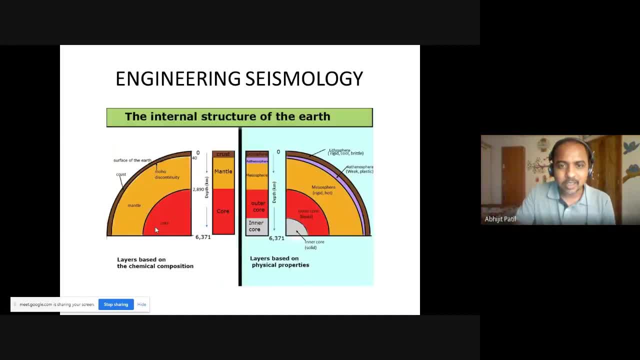 north-south poles, etc. okay, so this is the internal structure of the earth. so these are few more details like this lithosphere- it is again another name for crust lithosphere and asthenosphere. okay, so this is very rigid, cool and brittle. so what do you mean by cool if you compare the temperature at the core? 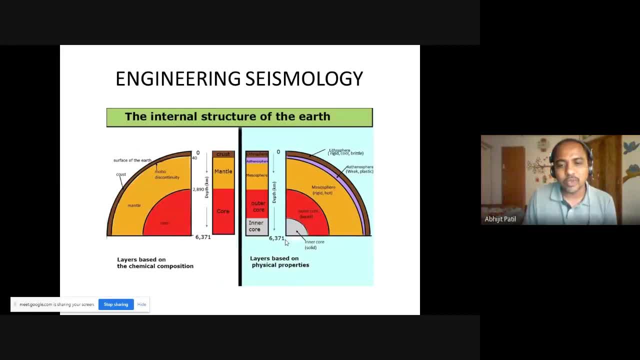 it is around 2400 degree centigrade and at this crust that is where we live. so this temperature ranges from minus 30 degrees somewhere to minus 30 degrees- and this is the temperature at which we live so- and or up to minus 50 degrees near the pole to, if you compare, the hottest. 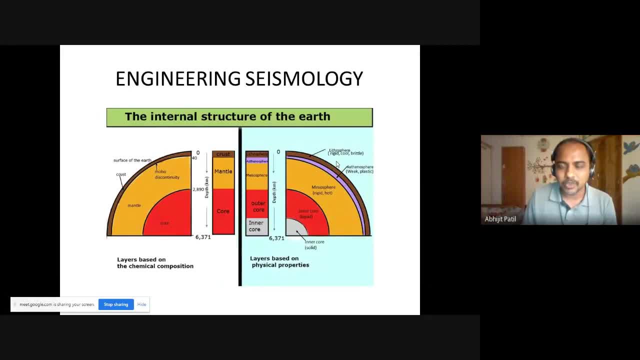 region it's plus 50 degree centigrade somewhere near the Sahara Desert. okay, so it is in the range of minus 50 to plus 50 roughly. so averagely you can see the atmosphere 25 to 30 degrees average and here 2400 degree centigrade. so the 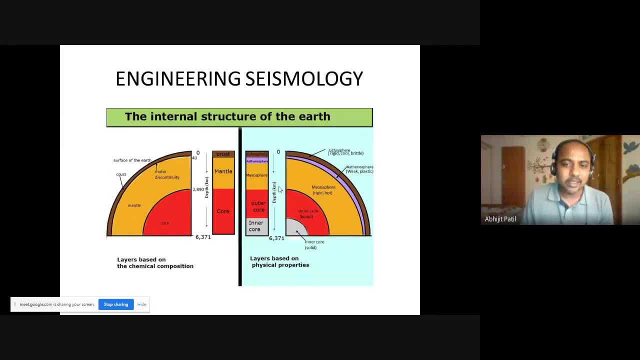 temperature goes on increasing, as you appreciate, from one end of Bonus, continue to take each of what a thermostat edge, your primary system to learn and what we want to show you, which is very important. um, I am going to give you another example. so this is the collection of tropical energy, fromrak and i, yeah, veryām, this is by I sandy. 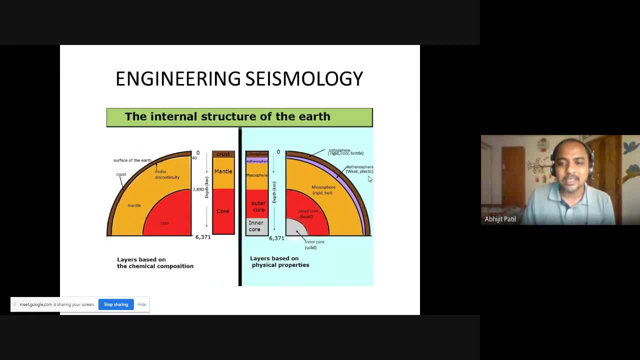 zza right, so that the main thing of the system right is they do not have with zero. you can see that the number ofθ so on each value, and when they are, Psalm 17 a, 0s. here this is EXCELTER거�2 and highest value, that the other Twins are certain, the. 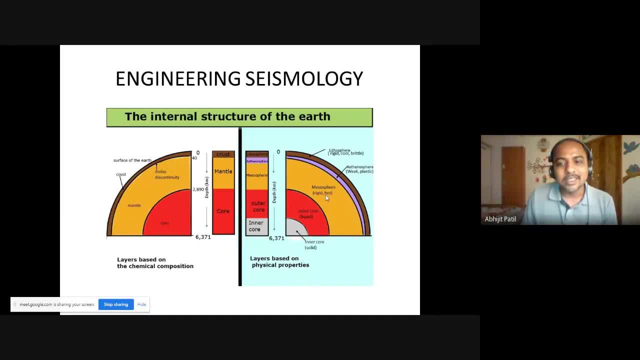 this is nothing but rock. this is molten rock. this is very, very hot, again in liquid stage. this outer core is again in liquid state and this is solid state. so you may wonder that at 2400 degree centigrade this internal core, inner core, because we know iron will melt, because here the temperature. 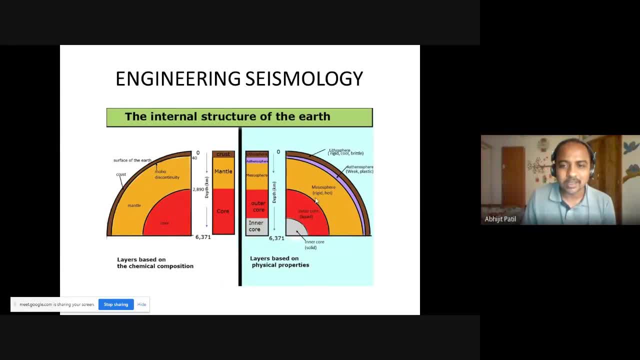 is less as compared to this, but here it is in molten stage. then why this stage is in solid stage? it is not only temperature, it is also pressure. so if you just try to recall that, well, physics, so pressure and temperature are related. so whatever we see by naked eyes, this is at. 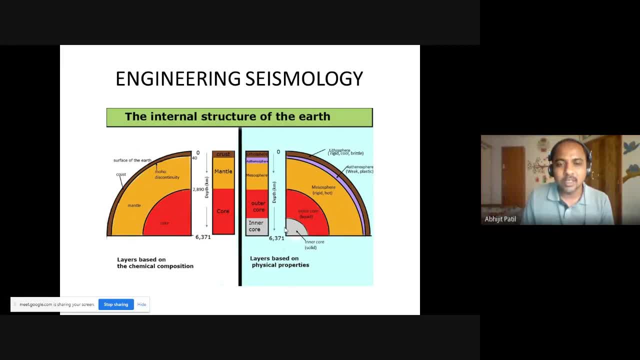 atmospheric pressure. but if you go on increasing the pressure, obviously the, what we call the temperature, where one state changes to another, that is melting point. okay, so the melting point of iron, the temperature increases because imagine huge mass of earth, it is rotating continuously and at the center we have this inner core. so there, the 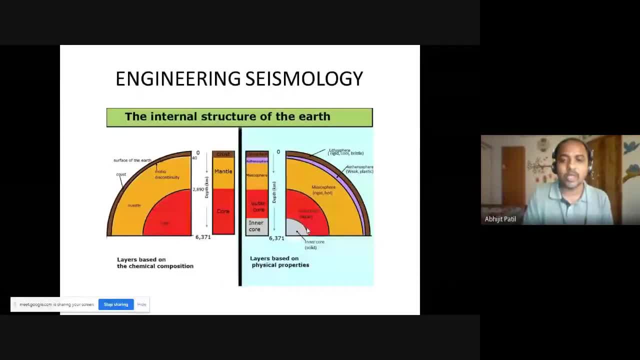 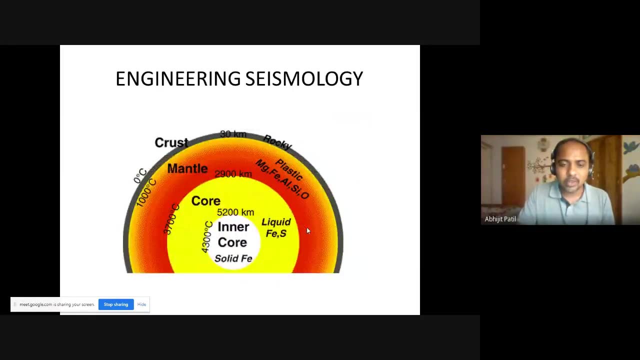 temperature is obviously high, but pressure is also high. that is why the iron, nickel, etc. whatever metals we have there in the inner core, those are not in molten form, those are in solid state. so yes, sorry, it is not 2500, it is 4300 degrees centigrade. okay, so this is just to see. 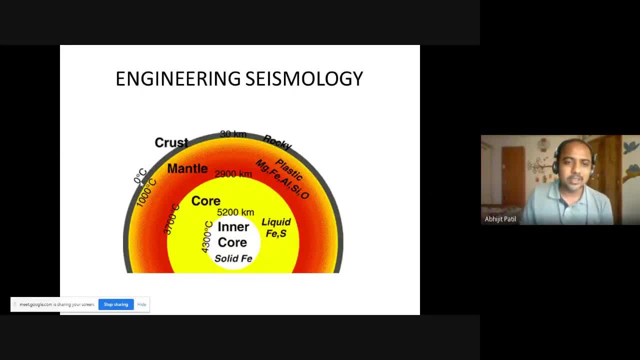 the temperature variation. so just above the crust is, you can say, atmospheric temperature, approximately 30 kilometers. so this is average. then in the mantle just below the crust it is 1000 degrees centigrade, here it is 3700 degrees centigrade and at the inner core you have 4300 degrees centigrade. 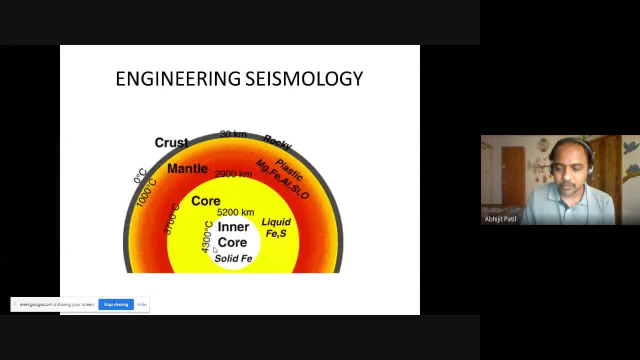 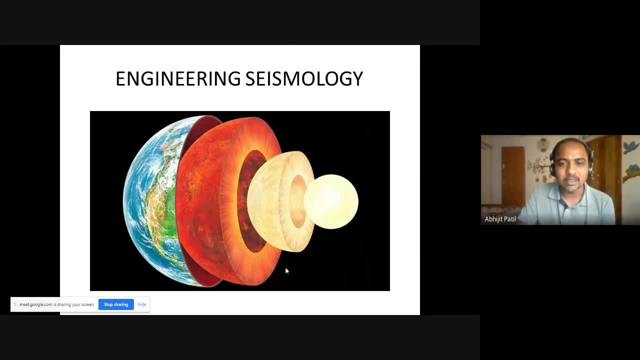 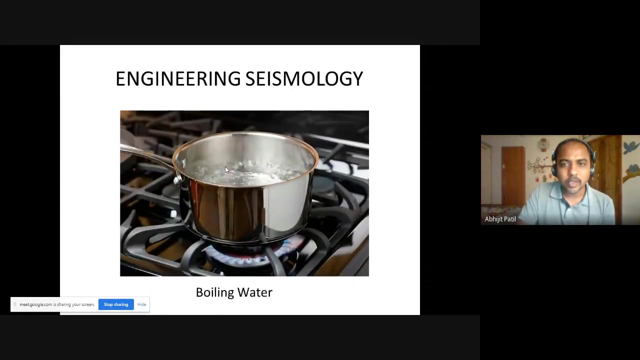 okay, so this is a beautiful imaginary, artistic view of what we have inside the earth's crust. so, whatever lava, etc. we see that that comes from this mantle part. so before- yes, we should discuss this also. so let us try to understand this phenomena. boiling water: can anybody tell me if in this image there is a pan room temperature water? 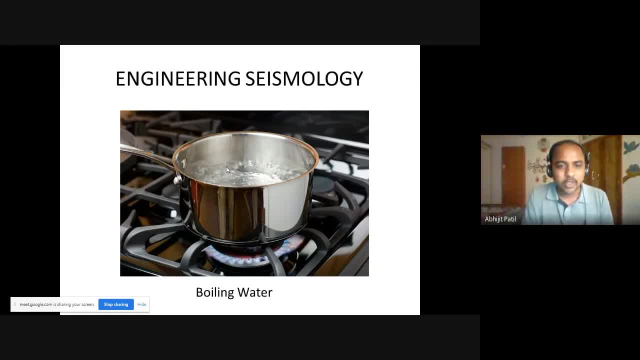 is poured and we are giving heat from bottom. so will the temperature of water rise uniformly from bottom to top, or a little bit? will it be something different story? can somebody share his or her views? so yes, so first, the water at the lower level, that is, in close contact to the pan, will get heated up. 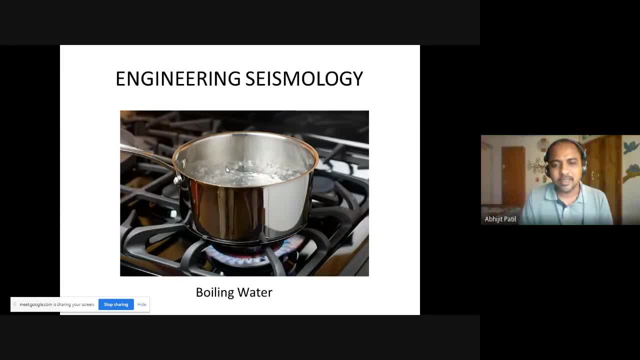 then slowly the water at the top, right right, exactly, exactly that will happen. so this makes sense that I don't know because I don't see the participants list when I share the window. can you tell me your name please? Pritesh Pritesh, Pritesh Pritesh. so this proves that Pritesh makes tea for his family members. so 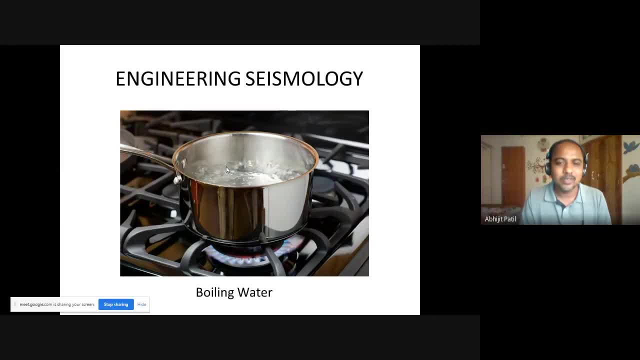 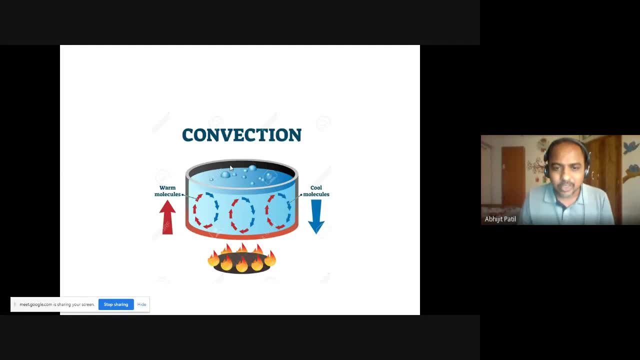 that is why he has observed it carefully and he could answer this. thank you, Pritesh. so that exact answer, so you can see. so this is the cross section of that pan. so what is happening in this pan? the water below this is in contact with the source of heat. okay, so it gets heated, the molecules get warmer and 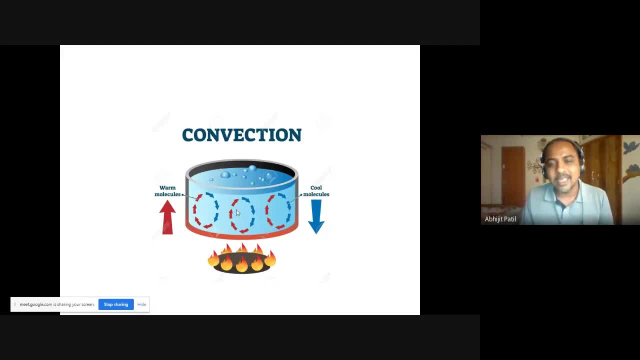 the density of warmer molecules is less as compared to density of colder molecules. so what will happen? this warmer molecules, okay. and another thing: the temperature difference. in technical words we call it as temperature gradient. so here the suppose the room temperature is 25 degrees centigrade. so at the top, these, these. 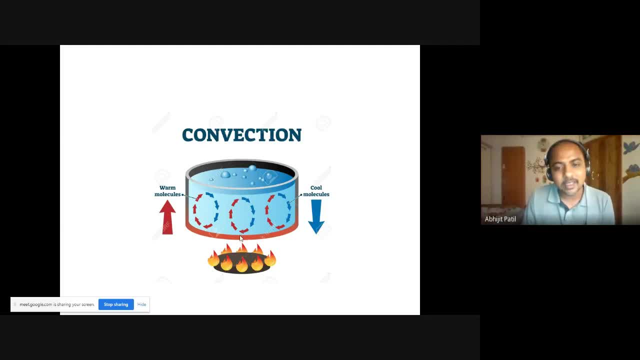 molecules are having temperature of 24 degrees centigrade and here from 25. when the source of heat is given, heat is given, it will start 25, 30, 35, 40. slowly it will increase. so at roughly around 45, 50, 55 or 60 degrees. what will happen? there will be temperature difference. so here it is 25, here it is 60. let us disolve this 온. 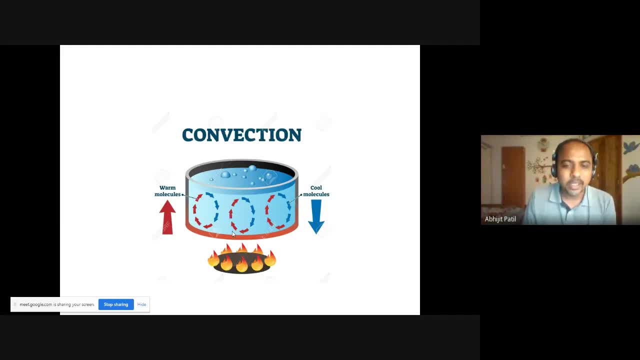 be temperature difference. so here it is 25, here it is 60, let's say so. these warm molecules will start moving upwards, okay, and these colder molecules will. these warm molecules will push these cool molecules downwards and again they will receive heat. and what will happen to these? 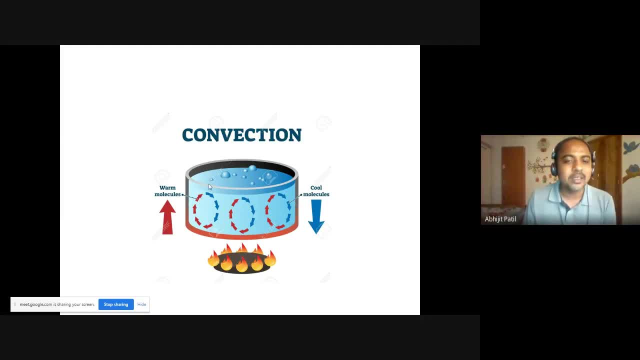 warm molecules. these warm molecules will release the heat to the atmosphere because there is temperature difference here it is 60 degrees and it is 25, so obviously the heat will be lost in the atmosphere. okay, but the heat is continuously being given at the bottom. so again, these cool molecules. 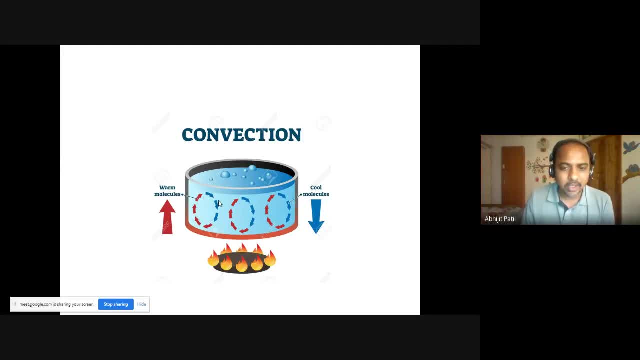 will become hotter. these warm molecules will become cooler again. this cycle will go on, but if you. but you will see, if this goes on then how the water will get heated, because after some time we see that bubbles are going to come out of the water and the water is going to come out of the water. 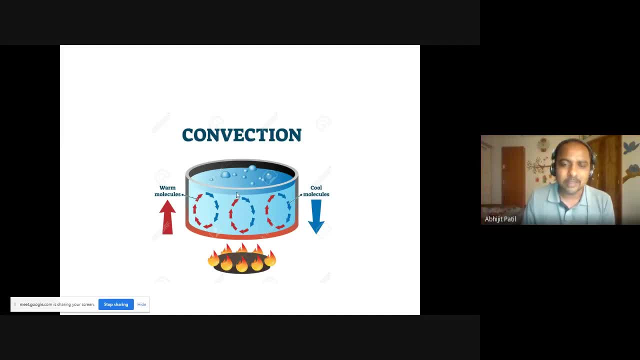 coming up the water. its total water is heated, so this rate of loss of heat is less, very, very less as compared to the rate of gain of heat. okay, but if you, the main point is there is this circle: always the molecules are moving, they are not stationary. so if you, 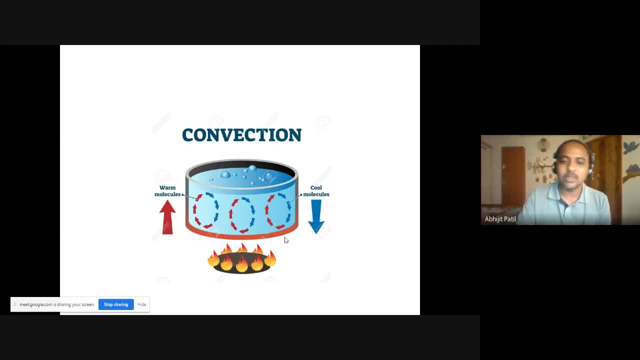 have not observed. just put a pan and observe it by yourself, because you will understand these things not just by listening, but just by doing so. this is very simple thing which you can do at your home or if you are staying at hostel and you have access to gas, you can easily observe this. so 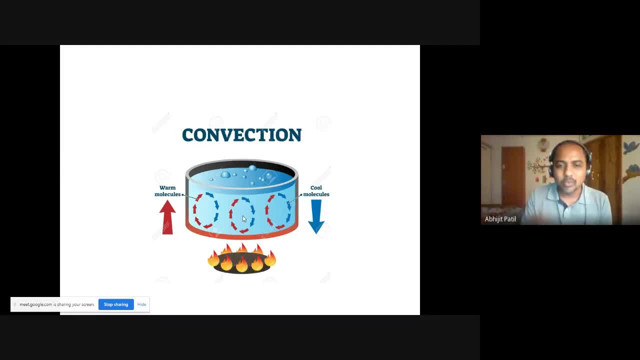 this is the thing happening: the molecules are moving, so these moving molecules are called as convection and these are called as convection currents. now why are we discussing this again? this is from school physics or school rhythm playing, which is: you get into the Redробlinrettik. 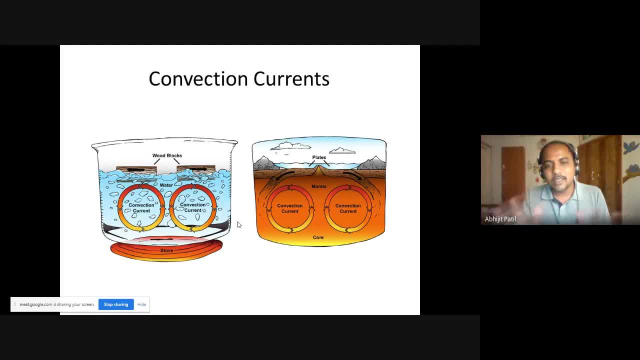 science. so this is the relation of what we have discussed. okay, so same pan, just put two small wooden blocks. okay, this also you can do and observe what will happen because of this convection of currents. okay, so these two currents are moving in opposite directions: anti-clockwise and clockwise. 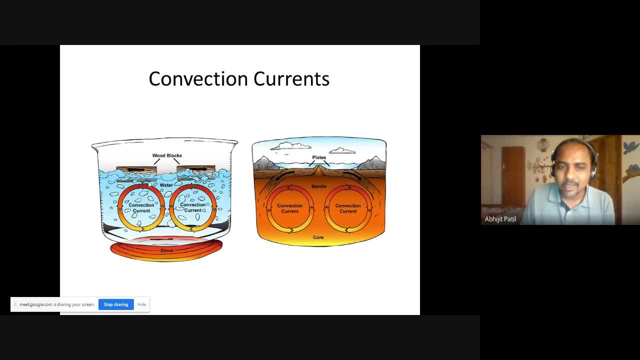 and if you put wooden blocks here which are floating on the water, these wooden blocks will move away from each other, agreed. because of this, we understood why this convection of current? because there is temperature difference: here it was 60- 70 degree, here it was 25- 30 degree. so water is moving in this fashion. 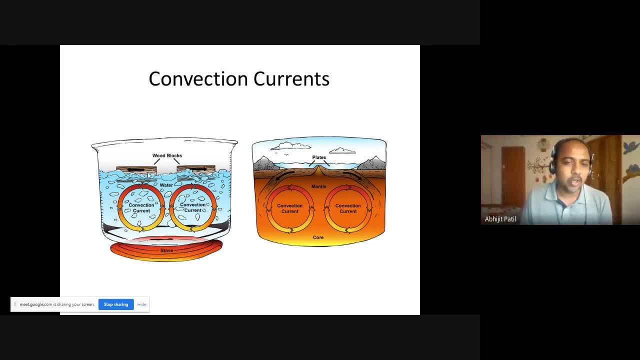 and if i observe, put some floating objects at the top of the water surface, it will start moving. sometimes they will move towards each other, sometimes they will move away from each other. okay, so this phenomena is directly applicable to our earth. so, instead of pan, imagine that this is our earth. instead of water, what we have at the core, the 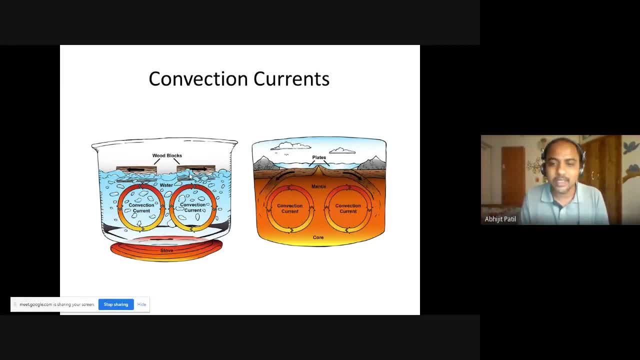 temperature of, i don't remember, 4 300 degree centigrade approximately, and here, at the top, where the plates are present, the temperature is 25 to 30 degrees celsius centigrade. okay, and this crust, if you recall just know what, what we discussed, that this mantle. 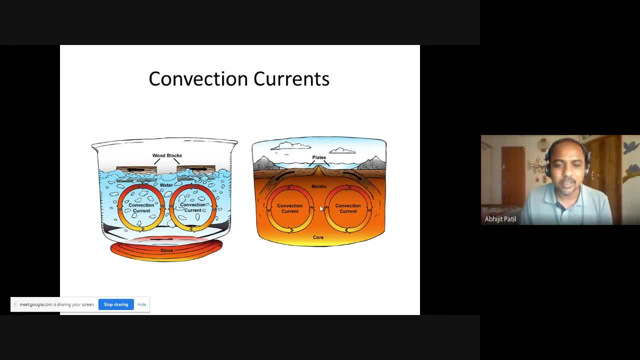 is in molten form, so this is acting as a liquid, so water mantle. just trying to give you the analogy, similarity: these plates are just like these wooden blocks. okay, so this earth's crust is not a unique, only one single piece. so if you play cricket with leather ball, so leather ball is just not a single piece. 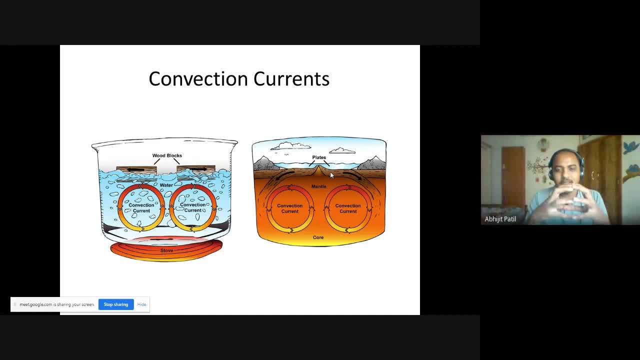 it is actually two pieces stitched together. okay, so, just like that. our Earth's crust is not a single piece. okay, it is different, different parts. so these are called as plates and they are just attached together. okay so, because these are different, different parts, and below the Earth's crust, what is happening? the 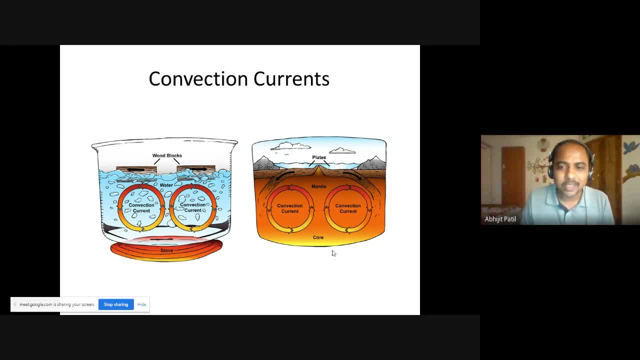 temperature is very high here, very low here, so the magma is continuously moving. there are different, different convection currents present- clockwise, anti clockwise- okay, and the plates above that magma, they start moving along with that convective currents, okay. so this is happening inside the Earth's crust, so, or? 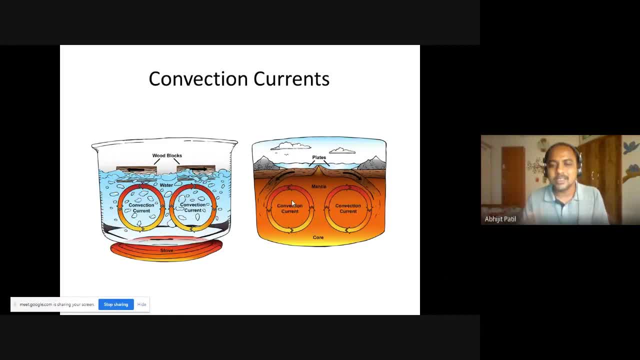 inside the interior of the Earth's crust. so these are different, different parts that matter to each other on Earth. so it is not a stationary object. I will just quickly sum up, before going to next point, what we discussed: the Earth's crust, Earth's interior consists of crust, then mantle, then core, outer and inner core. 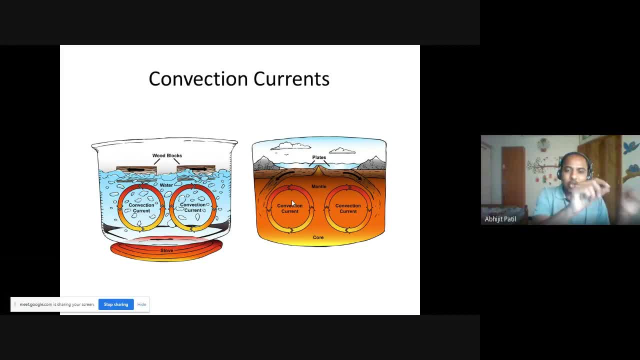 then earth's crust is rock, solid, rigid, it is basically rock. then below that mantle is a molten rock stage, so it is in plastic stage of the surface that in stage or semi-solid stage. Then below that you have core. And another thing we learned that the core is obviously. 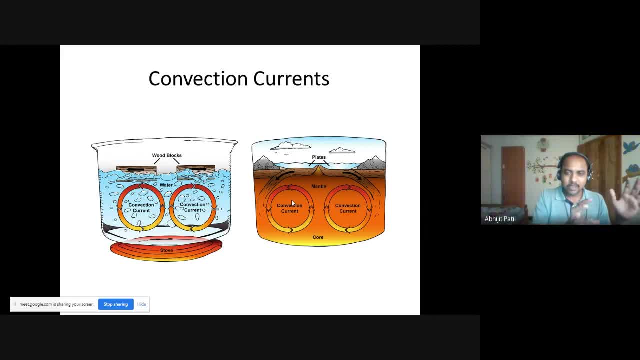 solid, but the temperature difference, so temperature at the core is tremendously higher than the temperature at the crust. Another thing we learned: because of this temperature difference, there is convection of currents. The magma is not stationary, It is a moving entity. 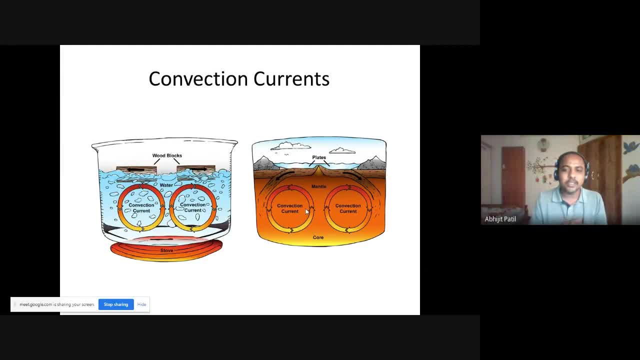 So it is continuously moving because of the temperature difference. So magma below gets heated, Then warm magma goes up, The cooler, relatively cooler- magma goes down And because of this there are continuous activity happening below the crust And the crust is not a uniform entity. 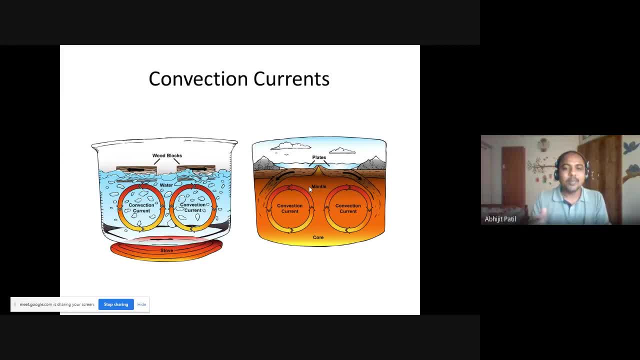 It consists of different parts. We call it as plates, And these are called as tectonic plates, And these plates are literally floating on the magma, And the magma is not stationary, It is always moving. So this is the thing: Everything is moving. 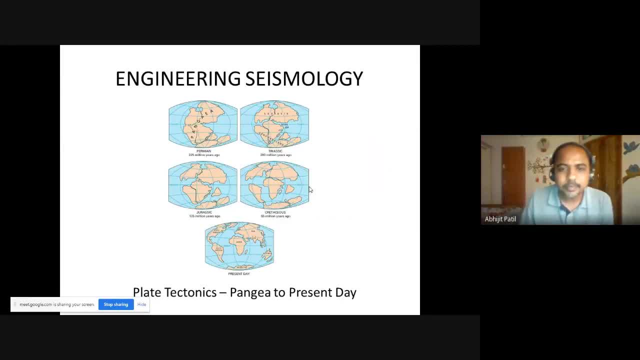 So what has happened because of this? So around 2,000, sorry, 225 million years ago, the continents- OK, I hope everybody understands continents. So we have continents and seas, So there are around seven to eight continents. So all those continents were attached together like this: 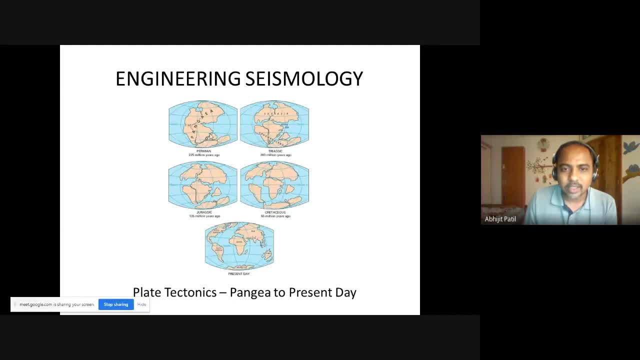 So if you see, slowly this started moving, If you concentrate on this plate, so this is an African plate, So each plate has a name, generally by the Continent's name. So this African plate, if you see it was below this equator and almost near to the South Pole. 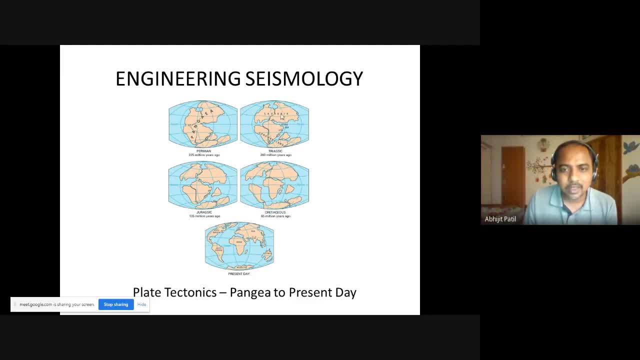 Then, slowly, it started moving towards- you can say 30 degree towards north, And this is east, so northeast, Slowly. here it has touched the equator, Here it has started crossing the equator here almost at the middle. 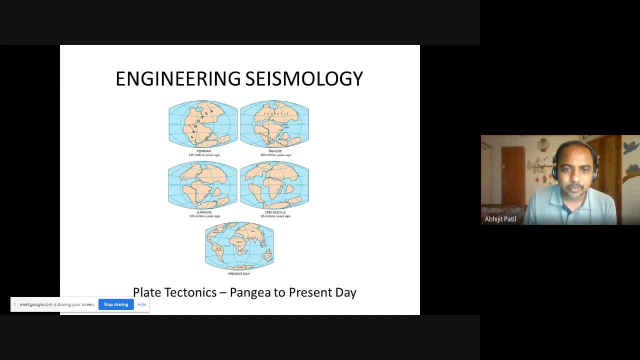 And here you can see the present-day Africa. OK, So why this plate started moving? Because below this the magma is moving in this direction: from southwest to northeast, southwest to northeast. Then if you see the Australian plate, so it was around near the South Pole. 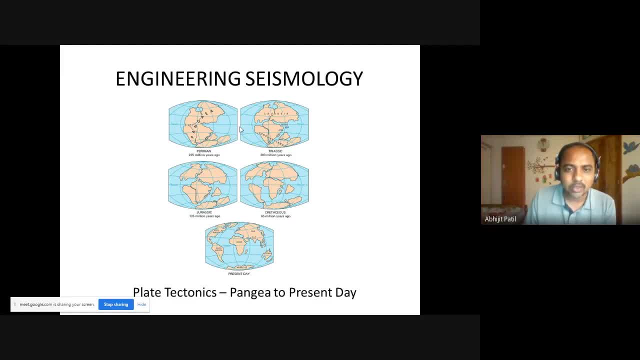 It has also started moving towards northeast. so, like this And present-day, you have Australia here, so from here to here. Similarly, see the South American plate. So South American plate, here it was present, attached to the African plate. 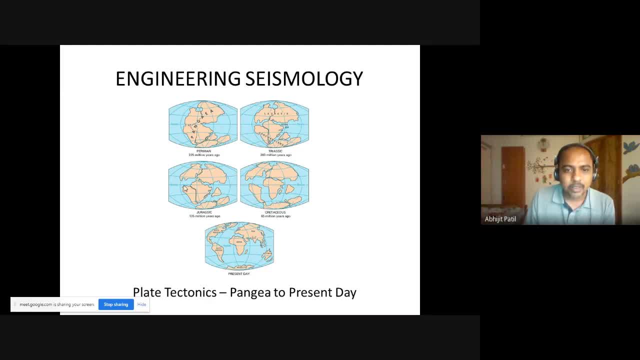 Then it has started moving towards west, west west And currently it is at this location. Now see the Indian plate. It was again attached to the South Pole and African plate. Then here it has started detaching from African plate. 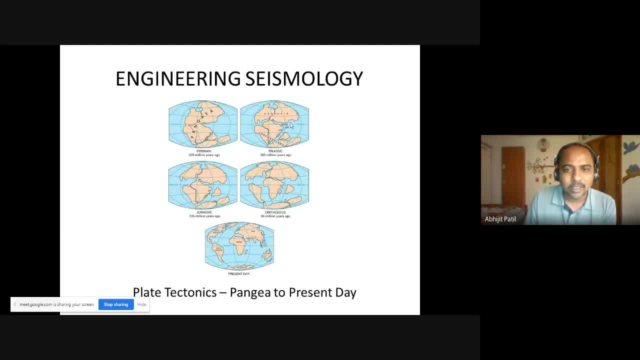 and started moving Like, OK, Australian plate. But then it has started journey from southwest to northeast and then towards north, OK, And here with the Eurasian plate. so this is Europe and this is Asia, so this is called as Eurasian plate. 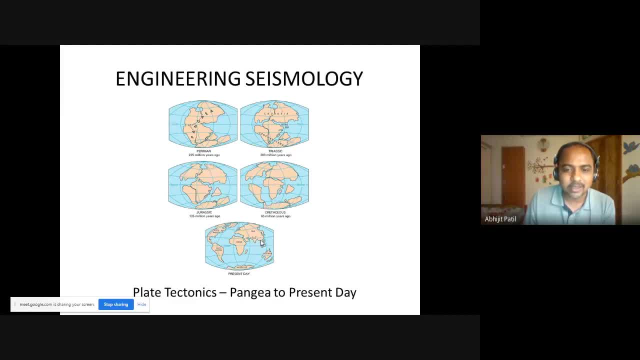 The Indian plate has attached And here, at this location, the formation of Himalayas is there. OK, So this is the thing. Because of all these happenings inside the Earth, the continents or the plates are continuously moving And they are changing its position. 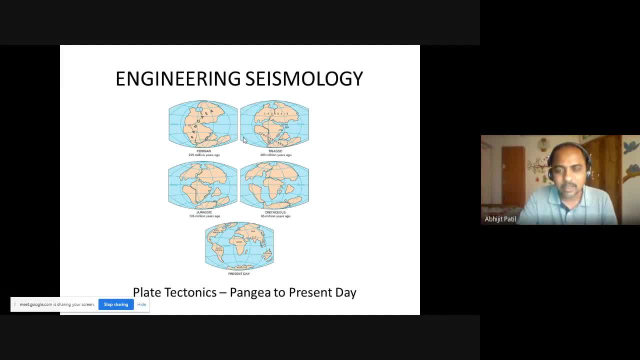 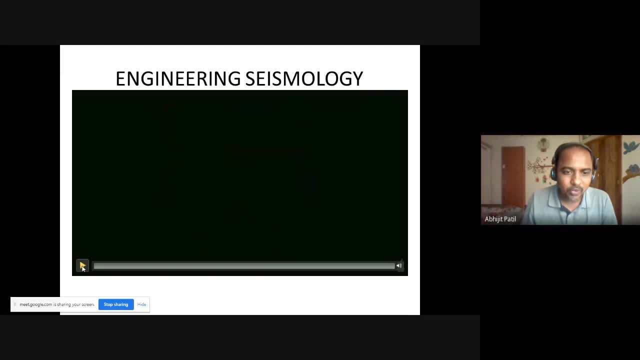 And because of that, the geology of Earth is continuously changing. So, with the help of a small video- of course this is not a technical video, But you will be- You will be just able to understand what exactly, or how exactly, the Earth's plates have been moved. 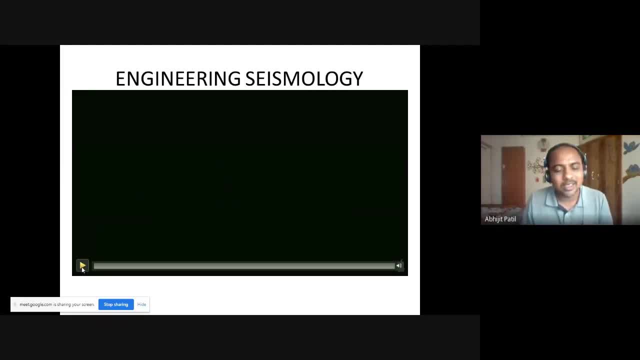 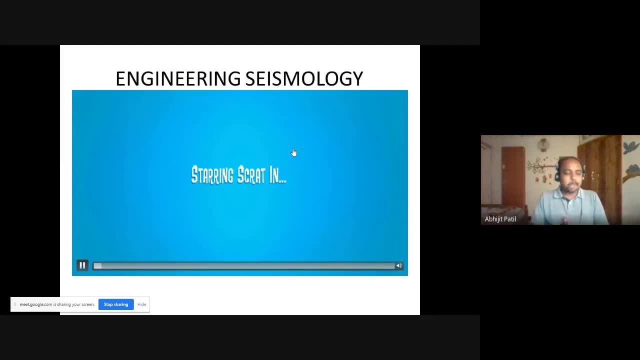 Of course, this is a clip from a movie, So take it lightly, Don't take it seriously. You'll uhhh, Oh, Oh, Oh, No, no, not that, Please, Don't take it seriously, Please. Ah, is it audible? 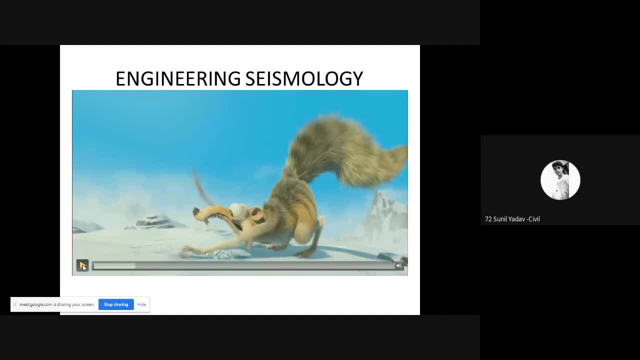 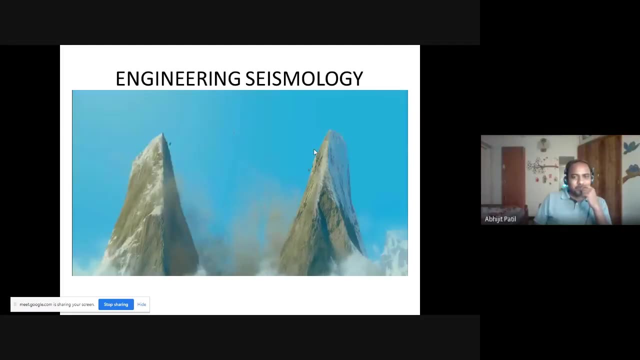 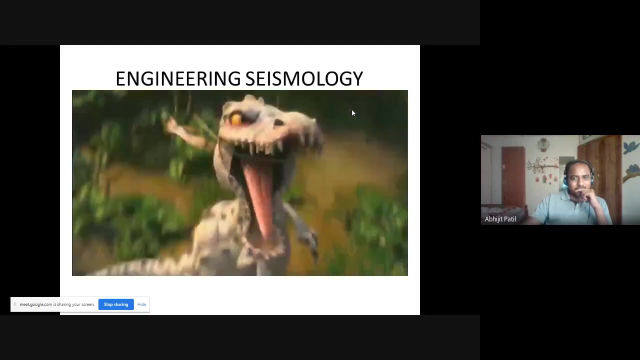 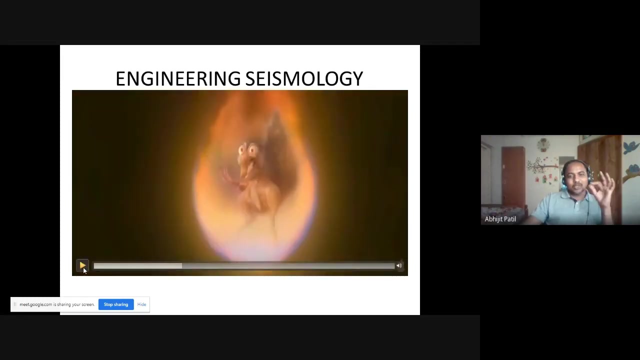 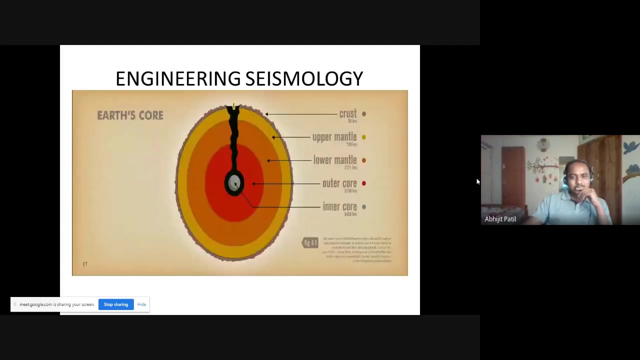 Yes, OK, Yes, sir, OK, thank you. so just the thing is, this squirrel is going inside the earth's crust, so that is why this temperature. it is feeling the increase or heat in the temperature. so this is what just now we discussed: the crust, the upper mantle, this yellow. 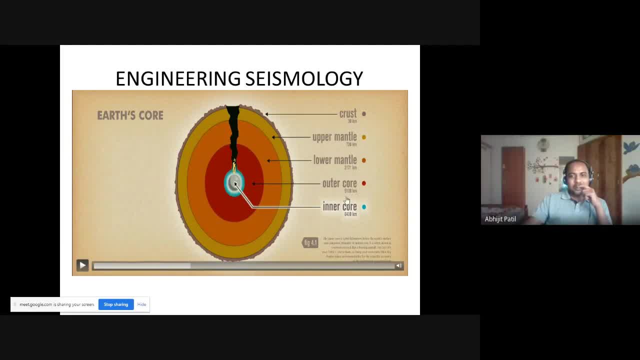 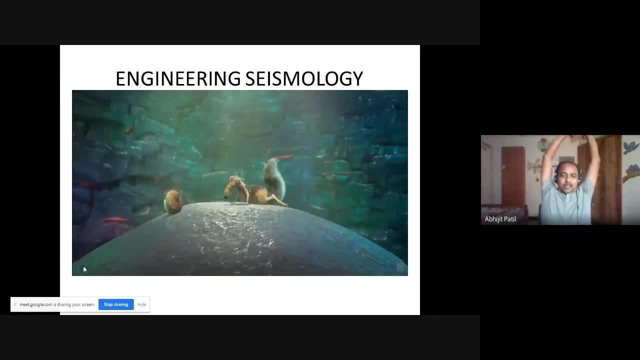 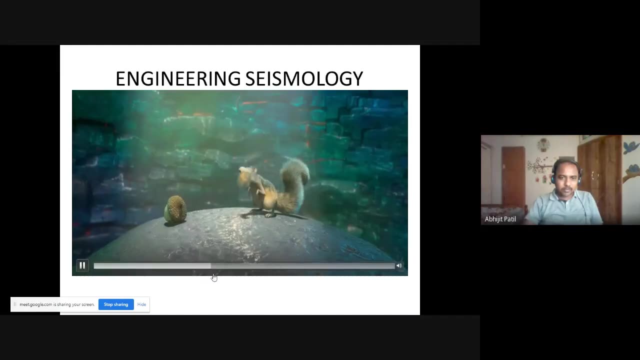 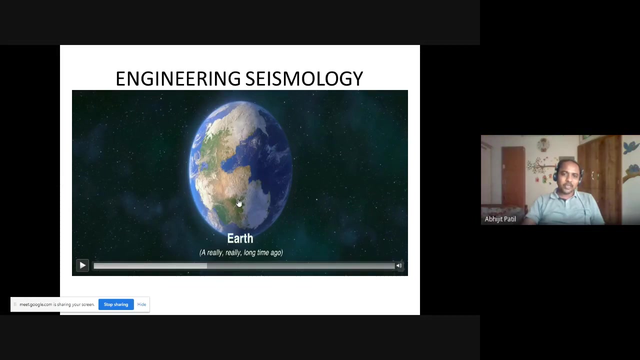 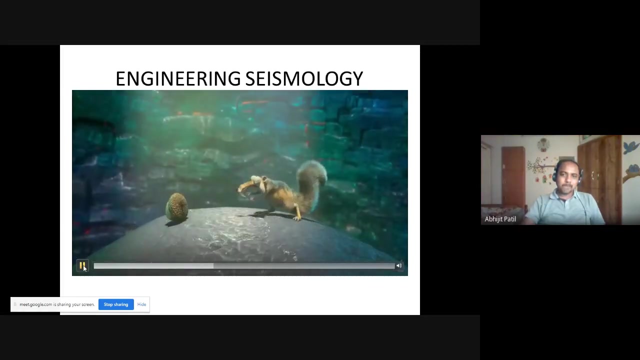 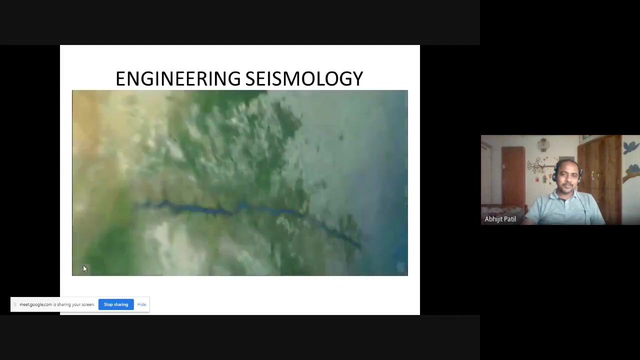 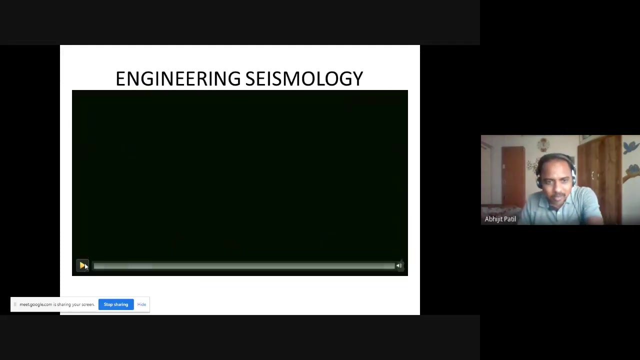 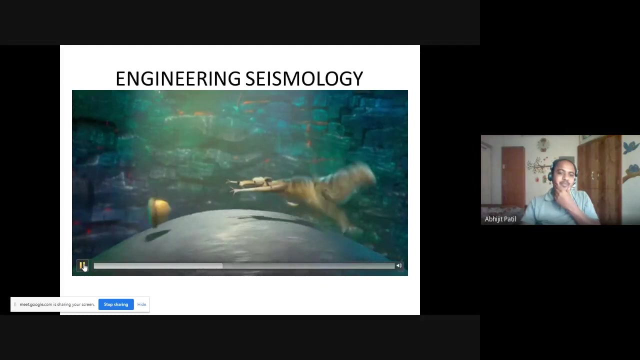 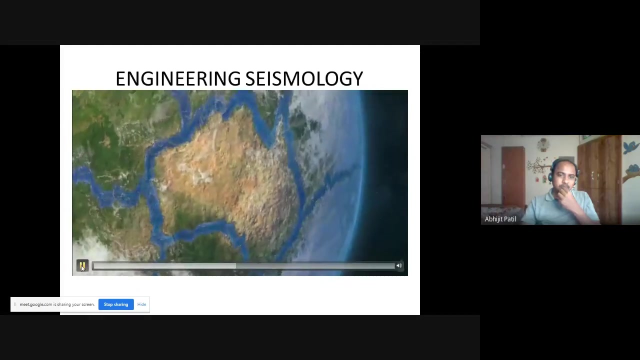 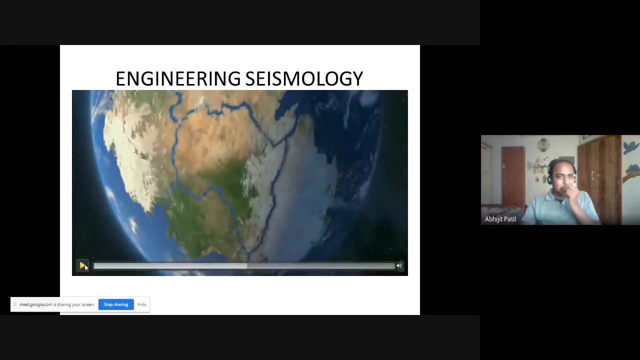 part, this orange part, lower mantle, the outer core and the rock solid inner core. so this is where all the continents were attached to you. sorry, so you can see these plates. okay, this cracking up started, so you can see. this is African plate, this is UE, this is actually the Indian. 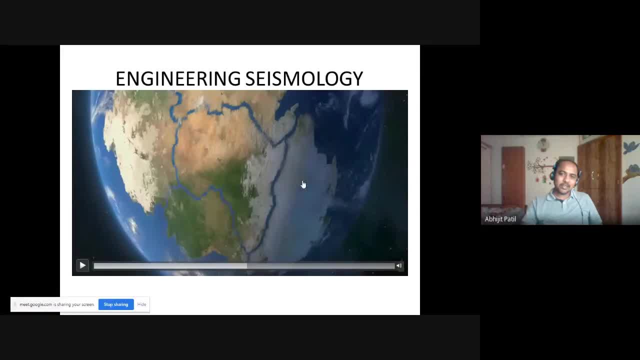 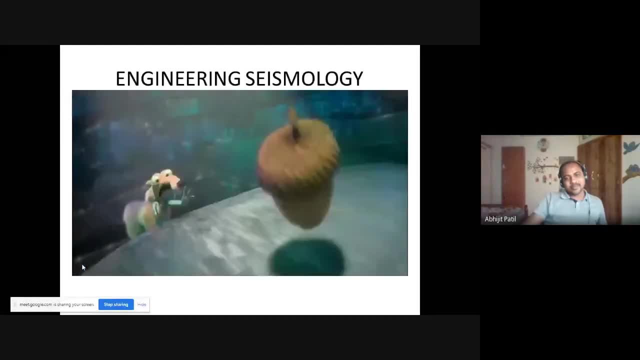 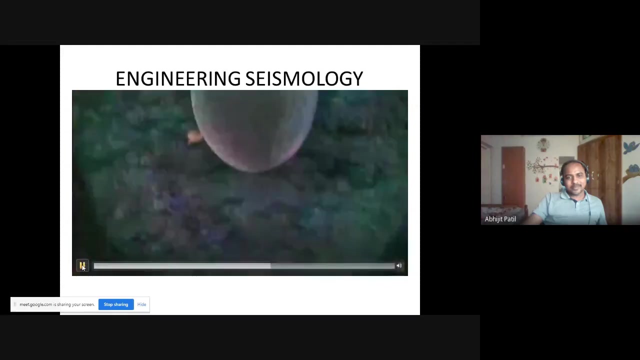 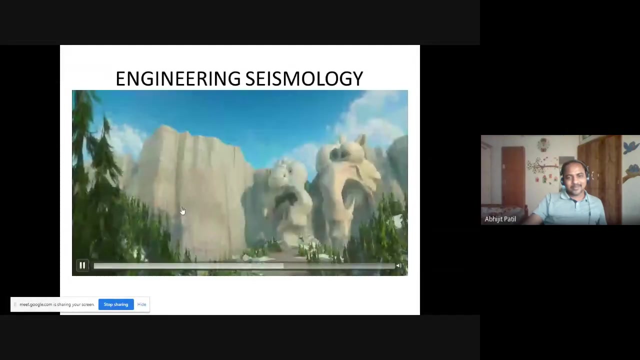 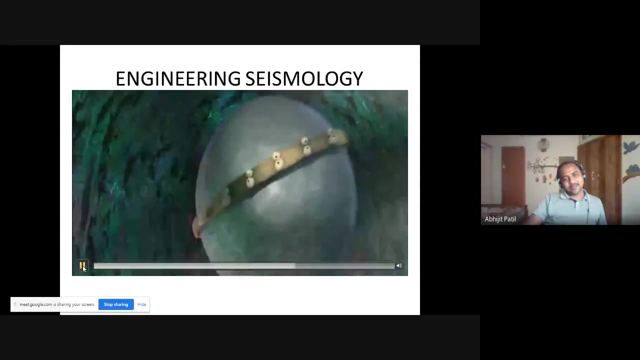 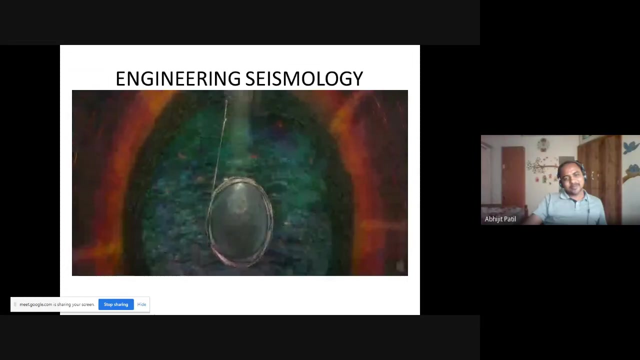 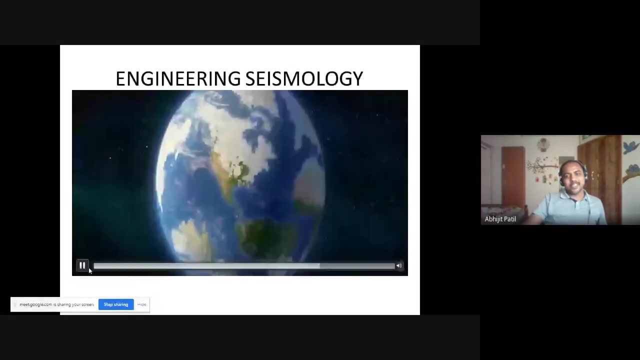 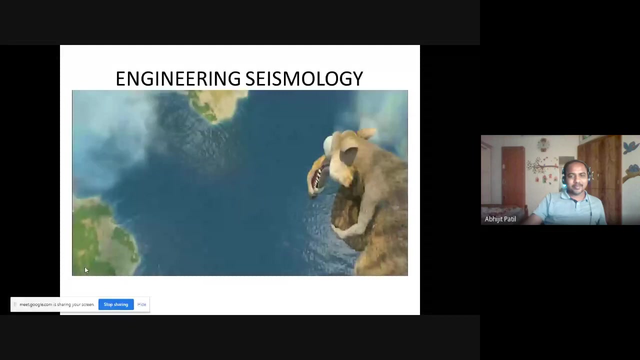 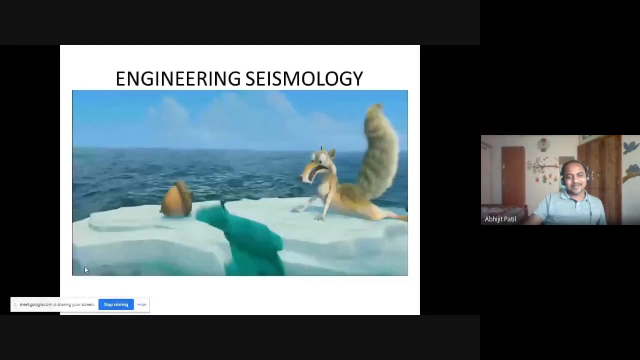 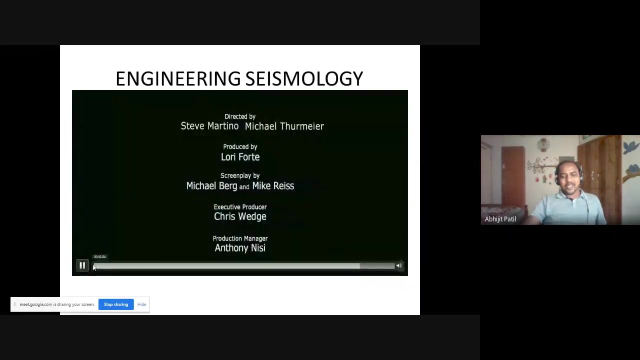 plate attached with the Australian plate. so this is the present-day map of the. so this is the present-day map of the world, okay. so apart from non-technical part, this, okay. so apart from non-technical part, this okay. so apart from non-technical part, this takes. 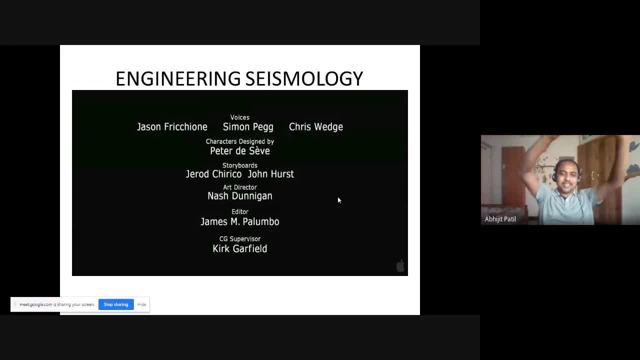 takes the technical part, that how the this is the technical part, that how the this is the technical part, that how the this is obviously. this is just for fun. this is obviously. this is just for fun. this is obviously. this is just for fun. this is not the actual reason of continental 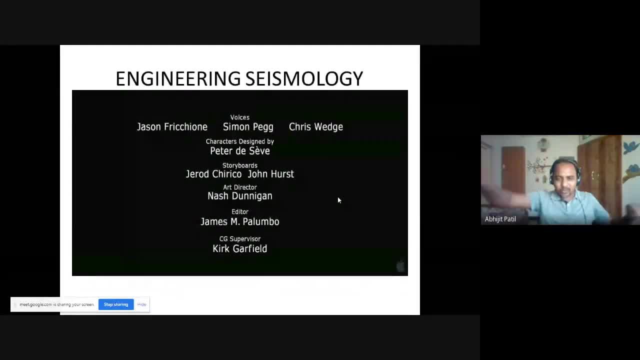 not the actual reason of continental, not the actual reason of continental drift. okay, so this is called as drift. okay, so this is called as drift. okay, so this is called as continental drift: the movement of plates, continental drift, the movement of plates, continental drift, the movement of plates. so we know the obvious, or technical, or 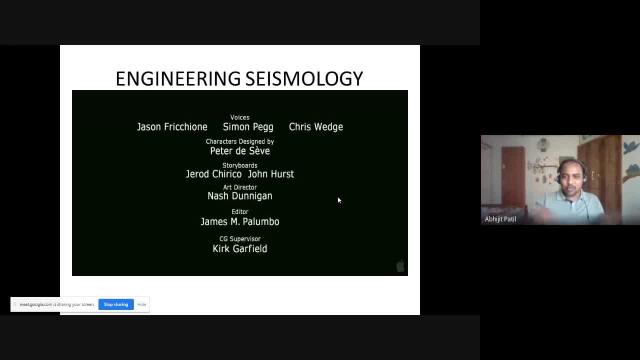 so we know the obvious or technical, or so we know the obvious or technical or real reason. this is because of the real reason. this is because of the real reason. this is because of the temperature difference: the moving magma temperature difference. the moving magma temperature difference, the moving magma, the convection of currents in the magma. 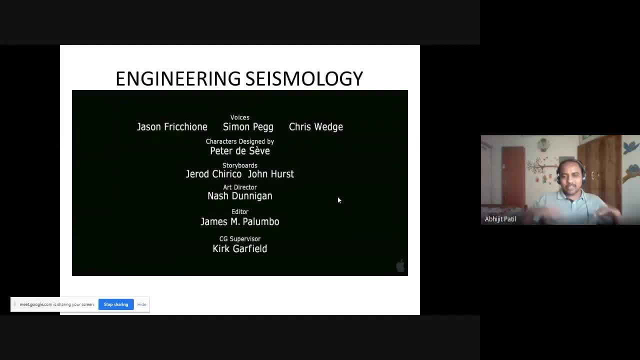 the convection of currents in the magma. the convection of currents in the magma and the nature of the Earth's crust which and the nature of the Earth's crust which and the nature of the Earth's crust which is floating on the magma. so that is the 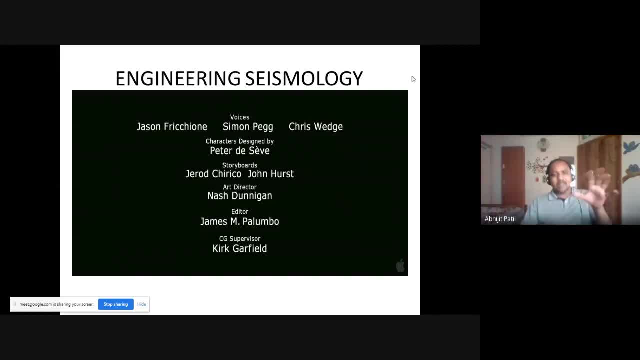 is floating on the magma. so that is the is floating on the magma. so that is the exact reason behind this continental exact reason behind this continental, exact reason behind this continental drift. but what is the takeaway from this drift? but what is the takeaway from this drift? but what is the takeaway from this? how these continents were attached. 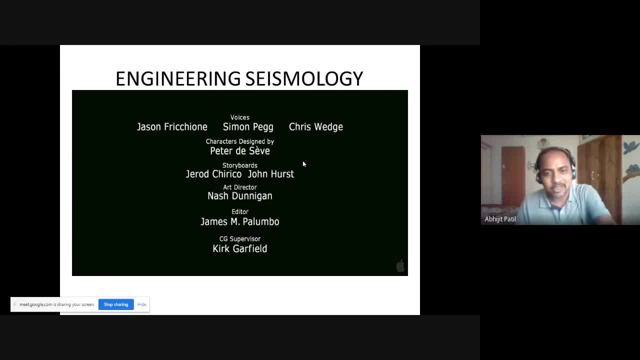 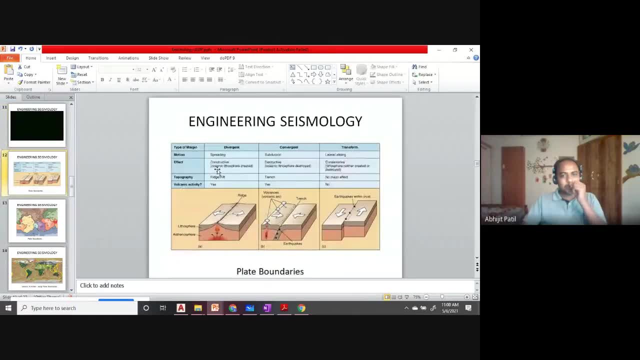 how these continents were attached, how these continents were attached together and how they got departed from together. and how they got departed from together and how they got departed from each other, and this movement is still each other, and this movement is still each other and this movement is still going on. okay, so, before we see this, 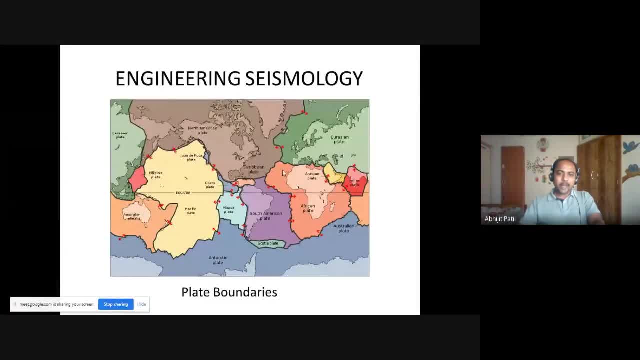 going on. okay, so, before we see this going on, okay, so, before we see this, okay, so this is the present-day map. so okay, so this is the present-day map. so okay, so this is the present-day map. so these are the plates South American. these are the plates South American. 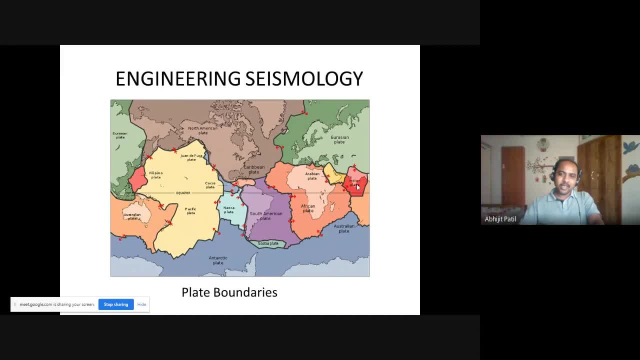 these are the plates. South American plate. so this is the African plate. this plate, so this is the African plate. this plate, so this is the African plate. this is the Indian plate. Eurasian plate. so is the Indian plate. Eurasian plate. so is the Indian plate. Eurasian plate. so this is Arabian plate. Australian plate. 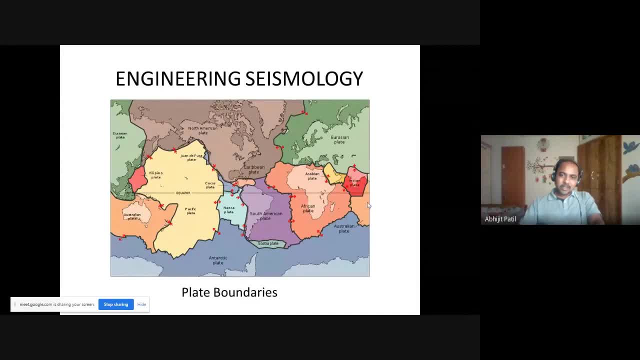 this is Arabian plate, Australian plate. this is Arabian plate, Australian plate. so you see the Australian plate, so you see the Australian plate. so you see the Australian plate continues from here to here. so it is continues from here to here. so it is continues from here to here. so it is only. this continent is small, but 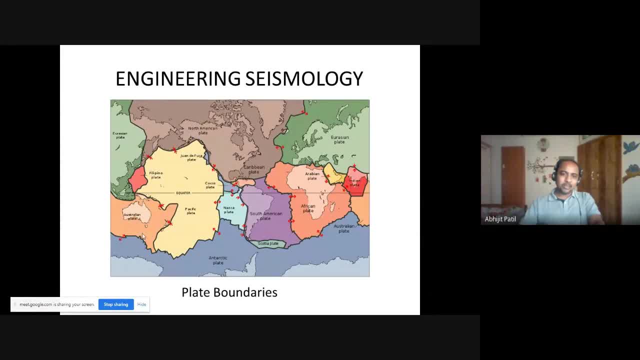 only this continent is small, but only this continent is small. but actually, if you see the size of the, actually, if you see the size of the, actually, if you see the size of the Australian plate is very, very large. Australian plate is very, very large. Australian plate is very, very large. Antarctic plate it is also very large. 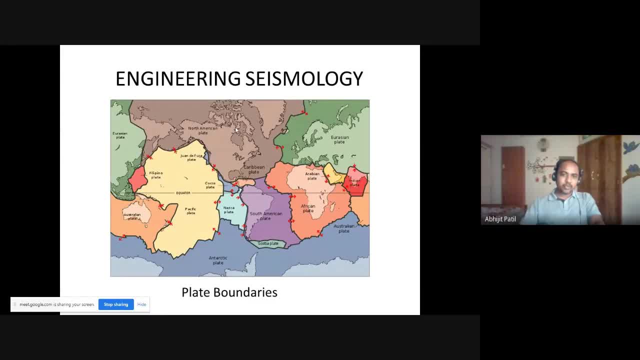 Antarctic plate. it is also very large. Antarctic plate, it is also very large. okay, then you have North American plate. okay, then you have North American plate. okay, then you have North American plate. that is also very large, so the largest. that is also very large, so the largest. 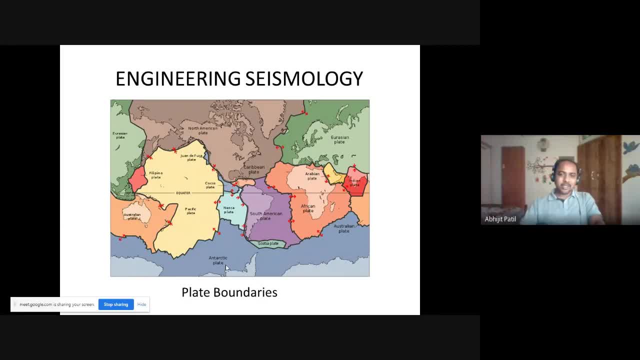 that is also very large. so the largest plate is North American plate, second to plate is North American plate, second to plate is North American plate, second to that is Antarctic plate and most of that is Antarctic plate and most of that is Antarctic plate and most of these two plates is covered with the. 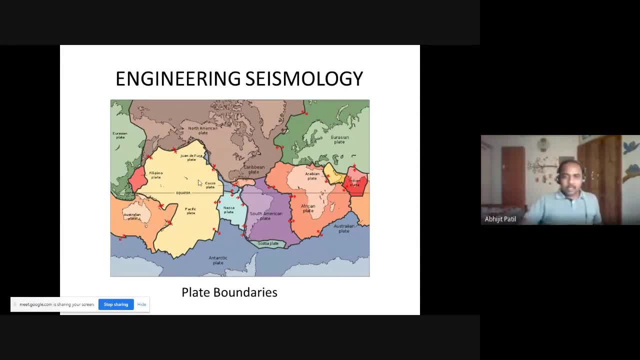 these two plates is covered with the. these two plates is covered with the water seawater. okay, now, just focus on water seawater. okay, now, just focus on water seawater. okay, now, just focus on these arrows. so we had seen that this: these arrows. so we had seen that this. 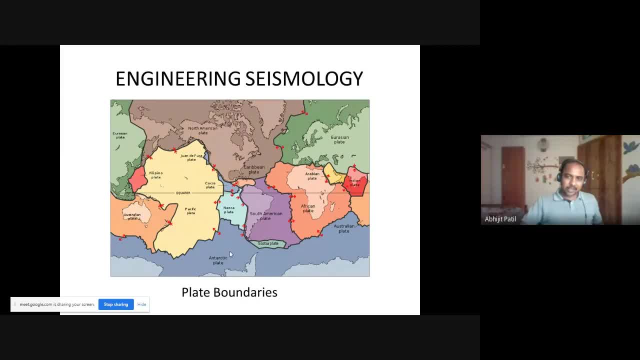 these arrows. so we had seen that this African plate was somewhere here and it African plate was somewhere here, and it African plate was somewhere here and it has started moving in this direction, so has started moving in this direction. so has started moving in this direction. so here now the current direction is like: 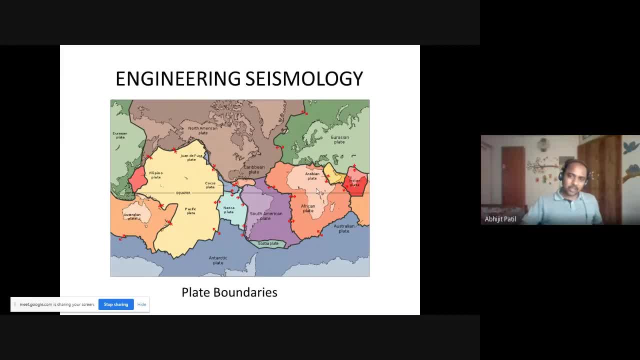 here now the current direction is like here. now the current direction is like this: so here some part of the African this. so here, some part of the African this. so here, some part of the African plate is moving like this, some part of plate is moving like this, some part of. 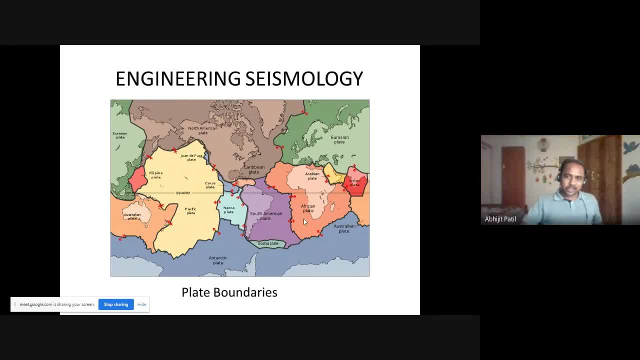 plate is moving like this, some part of the African plate is moving like this. so the African plate is moving like this. so the African plate is moving like this. so, since it is moving in a port direction, since it is moving in a port direction, since it is moving in a port direction, so here also it is moving in a port. 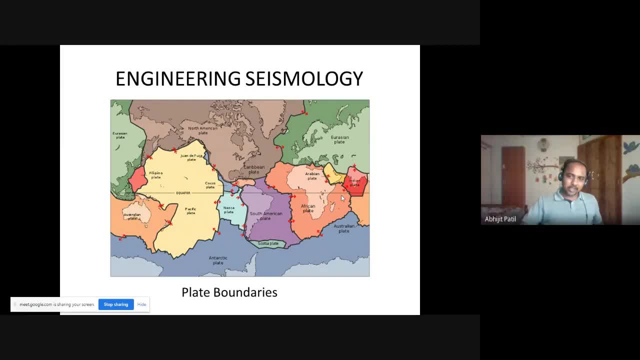 so here also it is moving in a port. so here also it is moving in a port direction. the Australian plate is moving direction. the Australian plate is moving direction. the Australian plate is moving in this direction. the Indian plate is in this direction. the Indian plate is in this direction. the Indian plate is moving in this direction. the Eurasian: 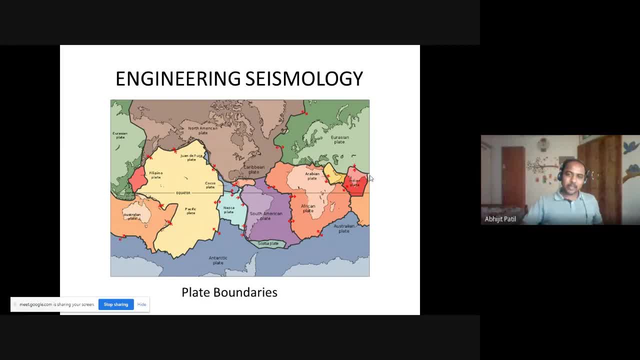 moving in this direction, the Eurasian moving in this direction, the Eurasian plate is exactly opposite to the Indian plate, is exactly opposite to the Indian plate, is exactly opposite to the Indian plate. and this is where the Himalayas plate and this is where the Himalayas. 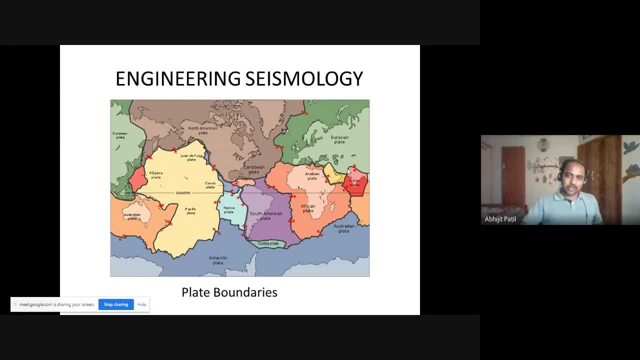 plate, and this is where the Himalayas were formed. after the collision of these were formed. after the collision of these were formed. after the collision of these two plates, the Himalayas were formed. two plates, the Himalayas were formed. two plates, the Himalayas were formed. and still, if you follow the news, the 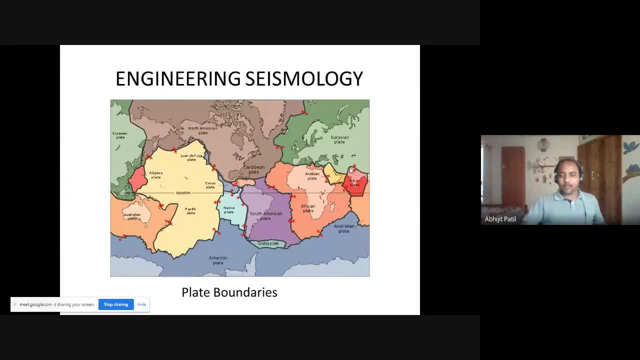 and still, if you follow the news, the, and still, if you follow the news, the, Everest is rising every year by a few. Everest is rising every year by a few. Everest is rising every year by a few centimeters, three or four centimeters. centimeters, three or four centimeters. 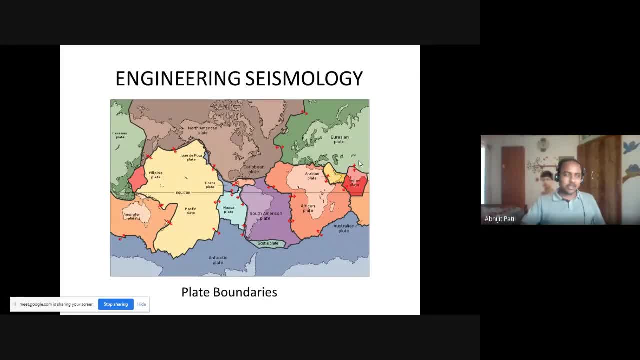 centimeters, three or four centimeters per year, like so, this move, these per year, like so, this move, these per year. like so, this move, these movements are still happening, okay, so, movements are still happening, okay, so, movements are still happening, okay. so why I'm showing this? because we want to. 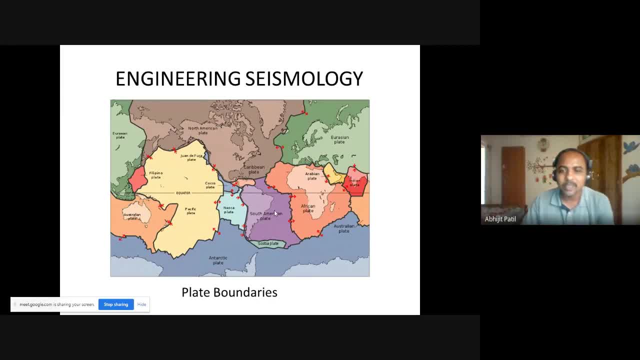 why I'm showing this? because we want to. why I'm showing this? because we want to know the plate boundaries. so wherever know the plate boundaries, so wherever know the plate boundaries, so wherever there these two plates meet, we call it. there these two plates meet, we call it. 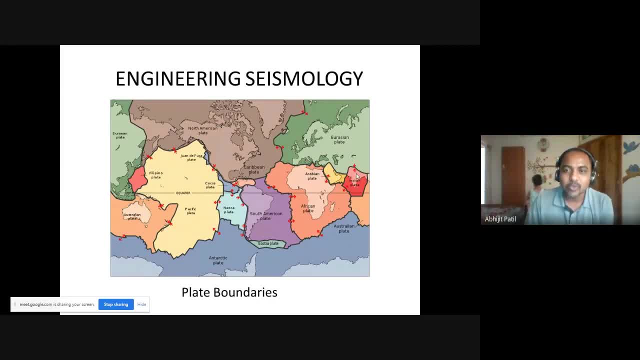 there these two plates meet. we call it as boundaries. so these two plates are as boundaries. so these two plates are as boundaries. so these two plates are moving towards each other. so this is moving towards each other. so this is moving towards each other. so this is called as convergent boundary. these two 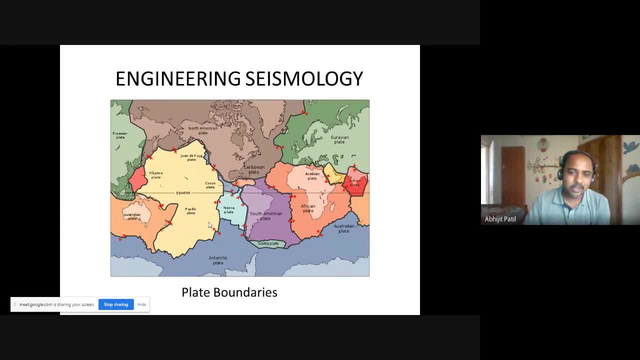 called as convergent boundary. these two called as convergent boundary, these two plates are moving away from each other. plates are moving away from each other. plates are moving away from each other. the South American plates towards West, the South American plates towards West, the South American plates towards West, African plate towards East. so this is: 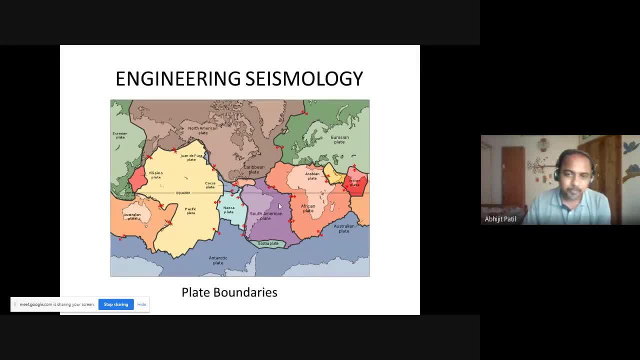 African plate towards East. so this is African plate towards East. so this is called as divergent boundary and these called as divergent boundary and these called as divergent boundary, and these two plates: the Pacific plate, where Pacific two plates. the Pacific plate where Pacific two plates. the Pacific plate where Pacific Sea is present, and the North American. 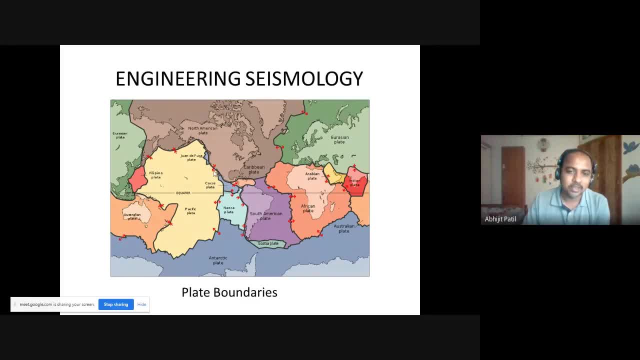 Sea is present and the North American Sea is present and the North American plate. they are moving parallel to each plate. they are moving parallel to each plate. they are moving parallel to each other. so these are called as parallel other. so these are called as parallel other. so these are called as parallel boundaries. okay, so once we understand, 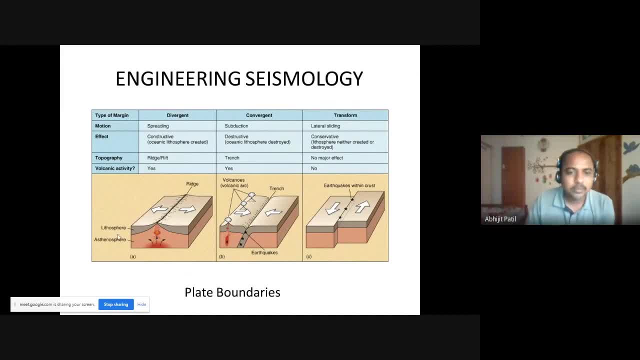 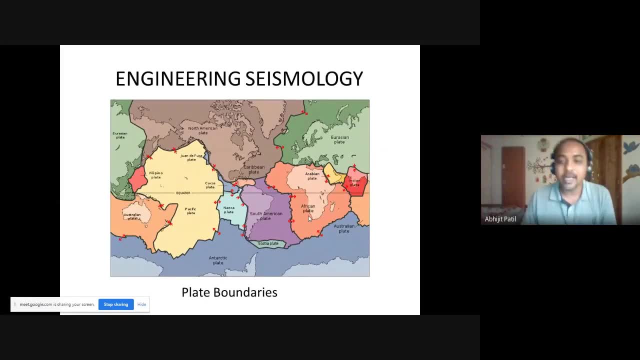 boundaries. okay, so, once we understand boundaries, okay, so once we understand this divergent boundary. the example is this divergent boundary. the example is this divergent boundary. the example is this one: the South American boundary. this one: the South American boundary. this one: the South American boundary, between South American plate and the. 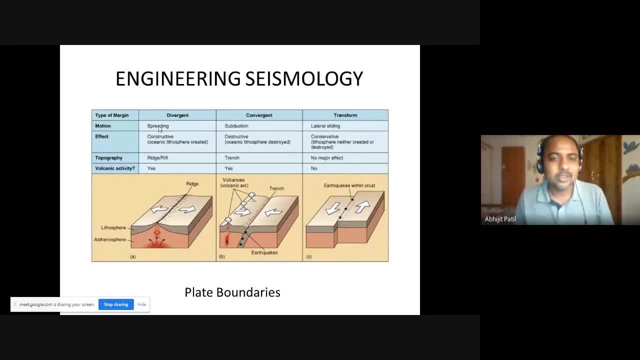 between South American plate and the between South American plate and the African plate. what is happening at the African plate? what is happening at the African plate? what is happening at the divergent boundaries? so the motion is divergent boundaries, so the motion is divergent boundaries. so the motion is spreading. that means they are moving. 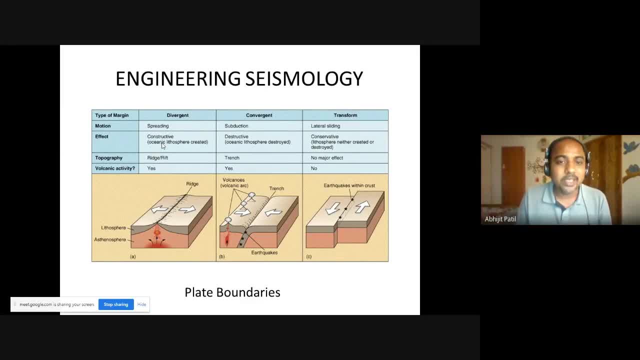 spreading, that means they are moving. spreading, that means they are moving away from each other and the effect is away from each other. and the effect is away from each other and the effect is constructive. so I will explain what is constructive. so I will explain what is constructive. so I will explain what is constructive. so, when these plates move, 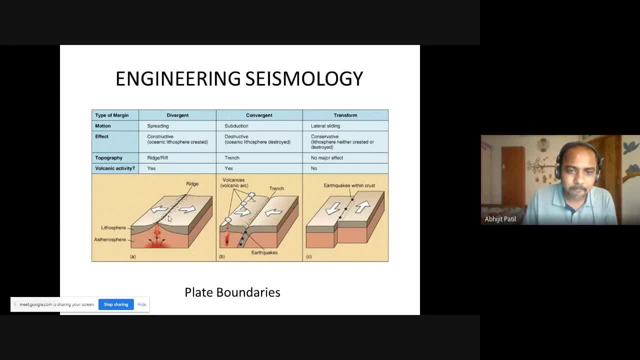 constructive, so when these plates move. constructive so when these plates move away from each other, this is a weaker away from each other. this is a weaker away from each other. this is a weaker section generally. a small ridge is section generally. a small ridge is section generally. a small ridge is present here and the magma tries to come. 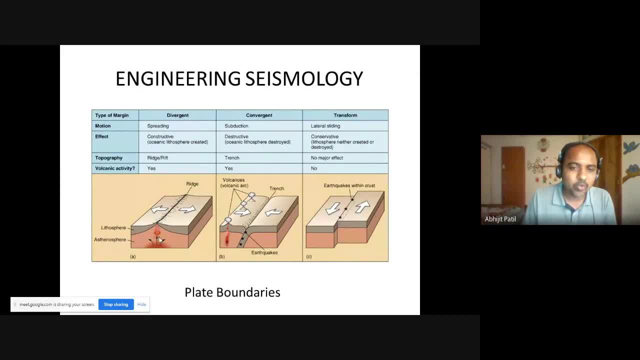 present here and the magma tries to come present here, and the magma tries to come out of this, out of this. so most of the out of this, out of this, so most of the out of this, out of this, out of this, so most of the volcanoes you will find are: 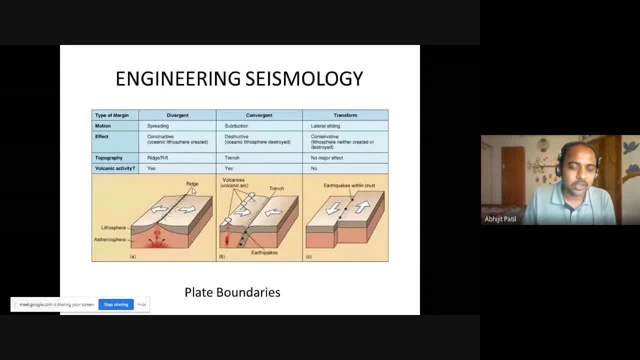 volcanoes you will find are volcanoes you will find are present on this divergent bondage. so you present on this divergent bondage. so you present on this divergent bondage. so you will not find that volcanic eruption is, will not find that volcanic eruption is, will not find that volcanic eruption is happening near Himalayas, because that is. 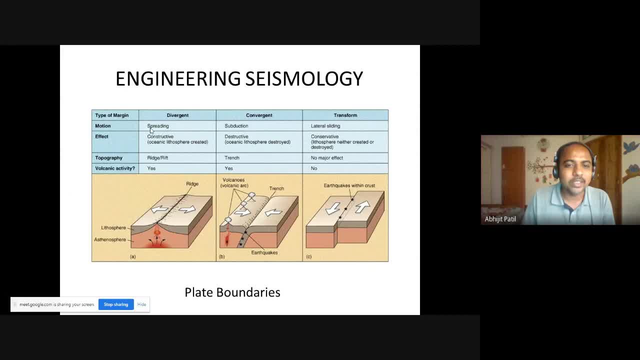 happening near Himalayas because that is happening near Himalayas, because that is is not a divergent boundary. that is, the is not a divergent boundary. that is, the is not a divergent boundary. that is the conversion: one leader: two boundaries are conversion: one leader: two boundaries are. 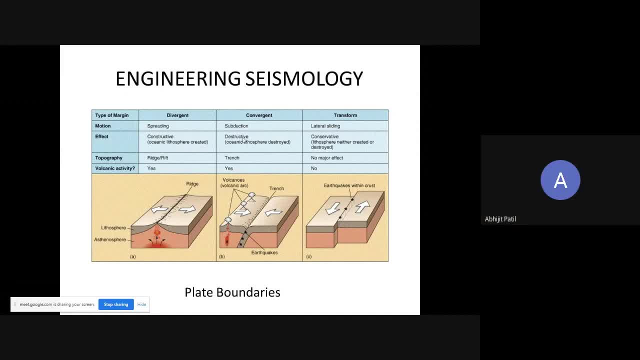 conversion. one leader, two boundaries are moving towards each other. okay, so this moving towards each other? okay, so this moving towards each other? okay, so this is destructive. why destructive one plate is destructive? why destructive one plate is destructive? why destructive one plate is going down and this obviously 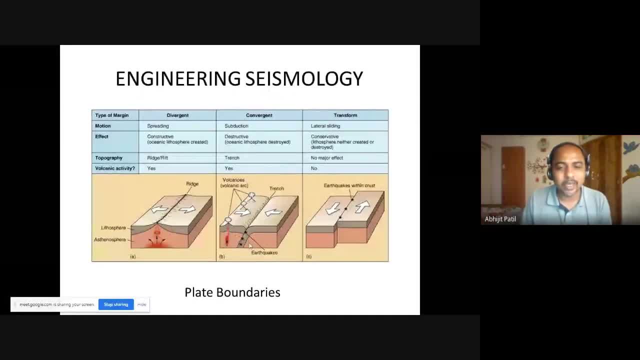 is going down and this obviously is going down, and this obviously because of the rising temperature, this because of the rising temperature, this because of the rising temperature. this gets melted and it becomes part of the gets melted and it becomes part of the gets melted and it becomes part of the magma. so here a destruction is happening. 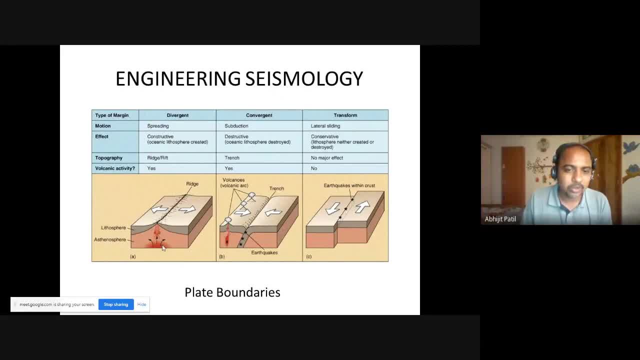 magma, so here a destruction is happening. magma, so here a destruction is happening here. construction is happening by here. construction is happening by here. construction is happening by construction. the volcanoes through construction, the volcanoes through construction, the volcanoes through volcanic eruption: the magma will come. volcanic eruption, the magma will come. 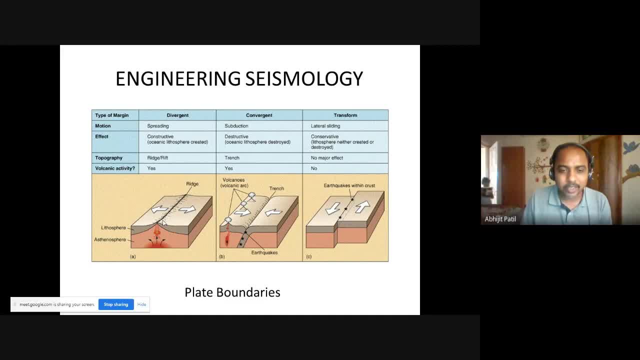 volcanic eruption, the magma will come out. and when it reaches the atmospheric out, and when it reaches the atmospheric out, and when it reaches the atmospheric temperature, it cools down and it becomes temperature, it cools down and it becomes temperature, it cools down and it becomes a part of the plate. so here it is. 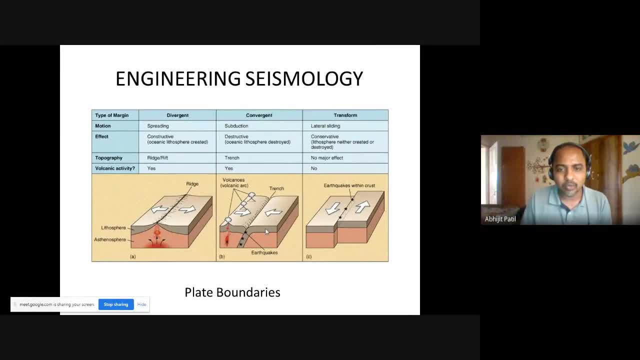 a part of the plate. so here it is a part of the plate. so here it is divergent, constructive. here it is divergent, constructive, here it is divergent, constructive, here it is convergent, so exactly at the boundaries. convergent, so exactly at the boundaries. convergent, so exactly at the boundaries. there will be trench, but nearby the 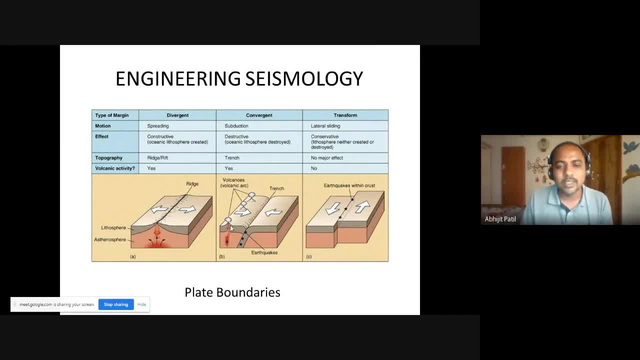 there will be trench, but nearby the there will be trench, but nearby the boundaries, there will be for formation of boundaries, there will be for formation of boundaries. there will be for formation of high ridges, so the Himalayas is good, high ridges, so the Himalayas is good. 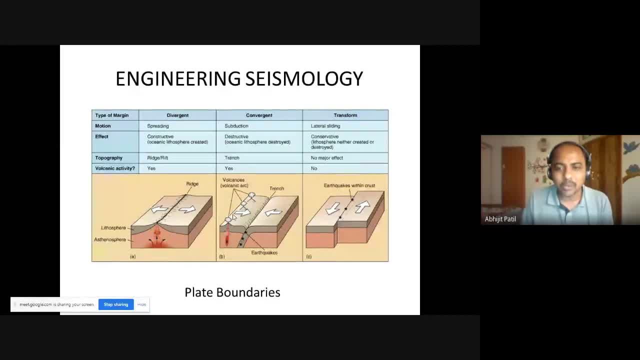 high ridges. so the Himalayas is good example of this. then you have transform example of this. then you have transform example of this. then you have transform boundaries or parallel bonds. so here the boundaries, or parallel bonds. so here the boundaries, or parallel bonds. so here the boundaries are moving parallel to each. 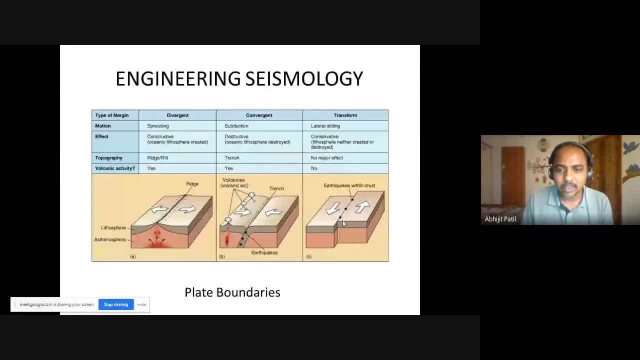 boundaries are moving parallel to each. boundaries are moving parallel to each other, okay, and there will be movement other okay, and there will be movement other okay, and there will be movement like this. so what are these stars marked like this: so what are these stars marked like this: so what are these stars marked? so I will just explain that belt of this. 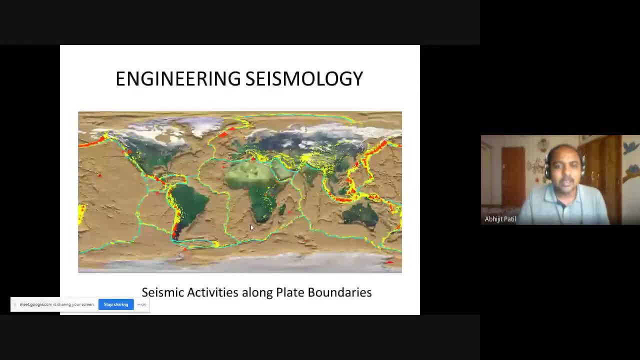 so I will just explain that belt of this. so I will just explain that belt of this. we will come back to this slide in few. we will come back to this slide in few. we will come back to this slide in few moments. so there is another theory called. 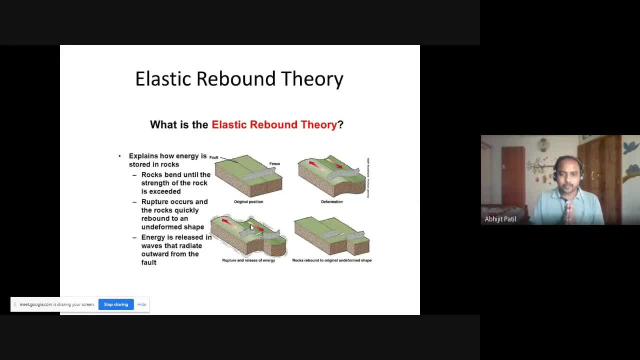 moments. so there is another theory called moments. so there is another theory called as elastic rebound theory. okay, so what as elastic rebound theory? okay, so what as elastic rebound theory? okay, so what is happening? you see now the mass of is happening. you see now the mass of. 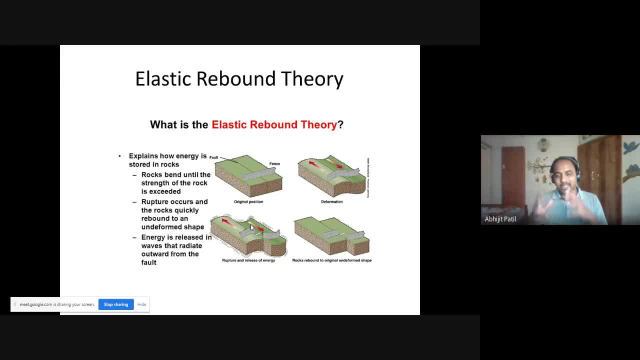 is happening. you see now, the mass of rocks or the plates is very large. if you rocks or the plates is very large. if you rocks or the plates is very large. if you just see the Indian plate, whole India, just see the Indian plate, whole India, just see the Indian plate, whole India, along with some part of Arabian Sea, it's 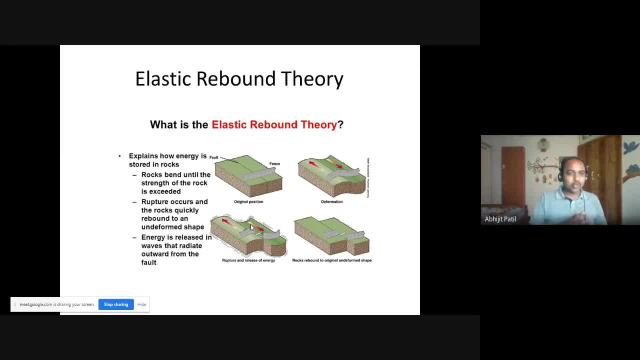 along with some part of Arabian Sea. it's along with some part of Arabian Sea. it's a plate hold the Africa continent is a a plate. hold the Africa continent is a a plate. hold the Africa continent is a plate. so you can imagine how much mass plate. so you can imagine how much mass. 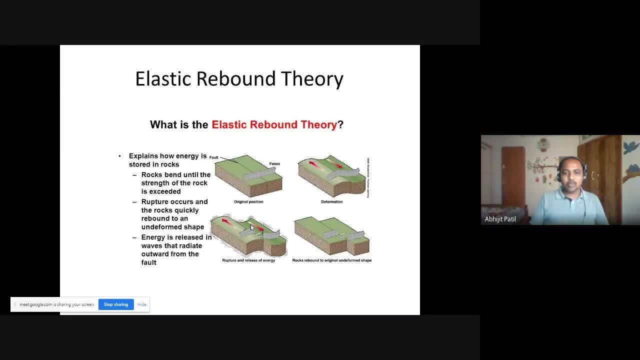 plate so you can imagine how much mass is involved. and this mass is moving, so is involved. and this mass is moving, so is involved, and this mass is moving. so whenever there is movement, it cannot be. whenever there is movement, it cannot be. whenever there is movement, it cannot be very smooth. okay, so add boundaries. what? 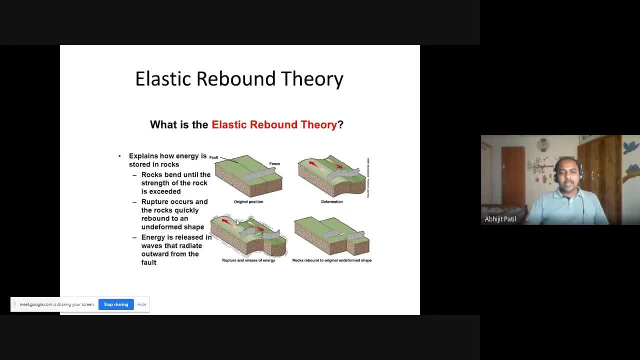 very smooth, okay, so add boundaries. what is happening? the magma is continuously is happening. the magma is continuously is happening. the magma is continuously moving below this plate, okay. so if you moving below this plate, okay. so if you moving below this plate, okay. so if you see, this is a fault line, so fault line. 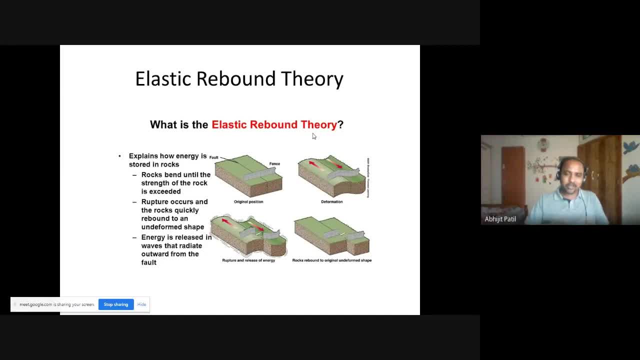 see, this is a fault line, so fault line- see, this is a fault line, so fault line is what it can be. one example of it can is what it can be. one example of it can is what it can be. one example of it can be inside the plate or it can be at the 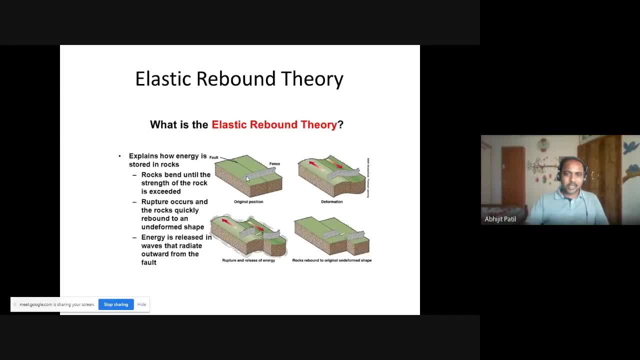 be inside the plate, or it can be at the be inside the plate, or it can be at the boundary of the plate. so, just for our boundary of the plate, so just for our boundary of the plate, so just for our understanding, we are attaching a fence. understanding, we are attaching a fence. 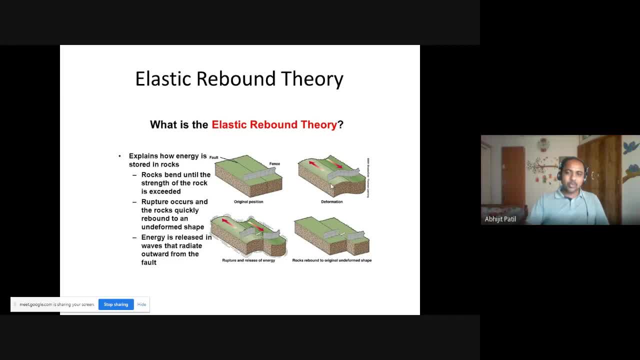 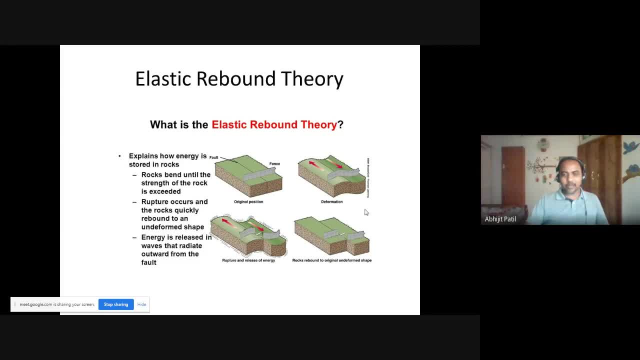 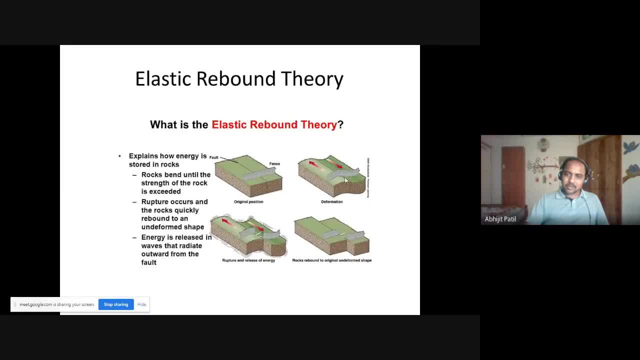 what is happening. this major part of the what is happening, this major part of the plate, is moving in this direction. major plate is moving in this direction. major plate is moving in this direction. major part of the plate is moving in this part of the plate is moving in this. 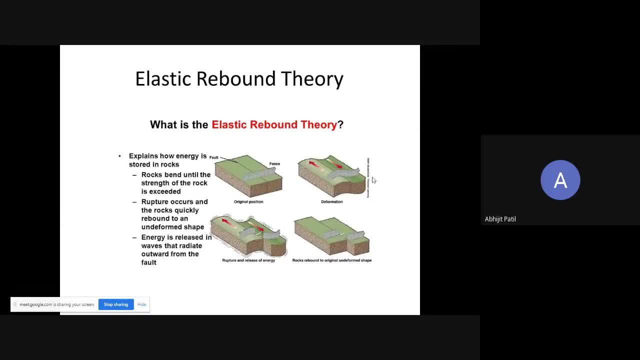 part of the plate is moving in this direction, but here at the junction direction, but here at the junction direction, but here at the junction. there is a connection between these two, there is a connection between these two, there is a connection between these two and push one hand in forward direction. 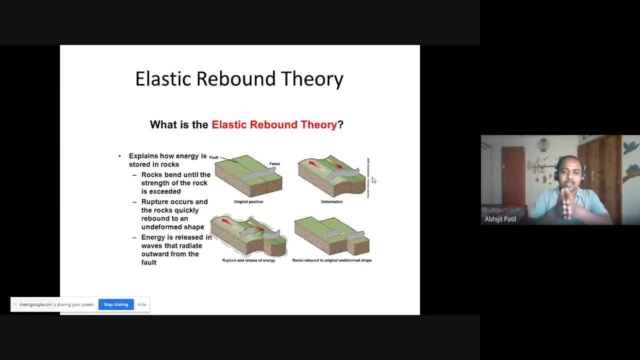 and push one hand in forward direction and push one hand in forward direction and one hand in backward direction, so and one hand in backward direction so and one hand in backward direction, so suddenly it will not. suddenly it will not, suddenly it will not move. why? because there will be friction. 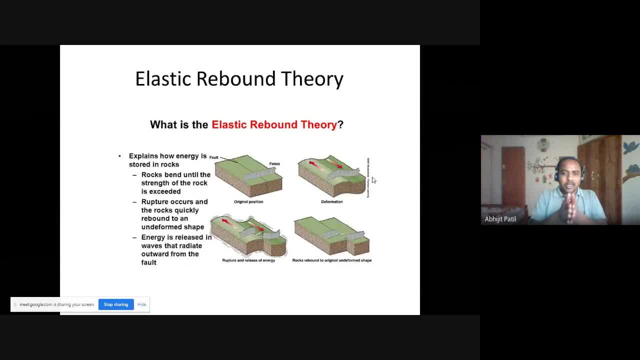 move. why? because there will be friction move. why? because there will be friction: friction between your palms, friction between your palms, friction between your palms, okay, and there will be built up of okay, and there will be built up of okay, and there will be built up of energy. 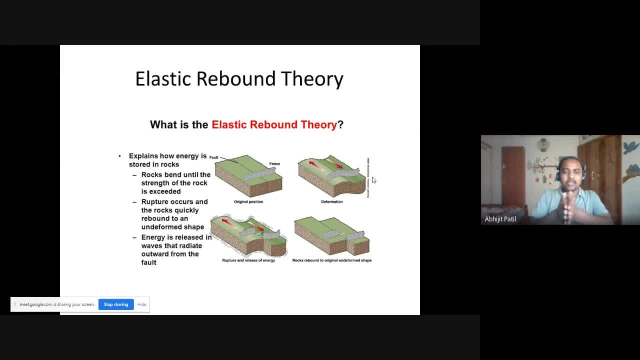 energy, energy. okay, if you continuously go on applying, okay, if you continuously go on applying, okay, if you continuously go on applying the force, go and increase the magnitude, the force. go and increase the magnitude, the force, go and increase the magnitude of the force, of the force. at one point, you will feel that your hands are getting stressed, okay. and at one point, when the 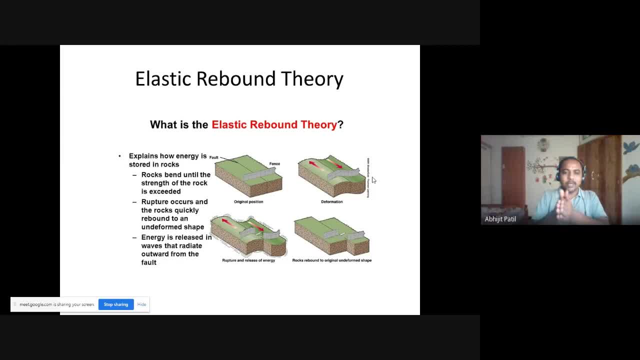 force applied is more than the friction between palms. there will be sudden sleep between your palms. okay, and the release of stress. you will feel that the stress which was induced in the arm of your hand will get released, and this stress gets released in the form of energy. okay, because this 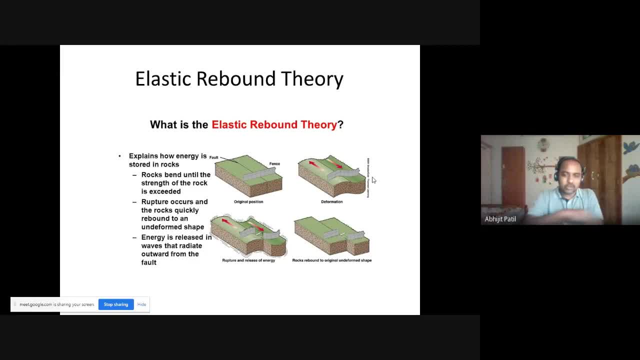 energy. why the stress was there? because the energy, the force which we were applying, that was getting stored in the form of stress in the rock, and when there is sudden displacement, okay, that energy gets released in the form of heat, in case of our rubbing of palms, okay. so imagine: 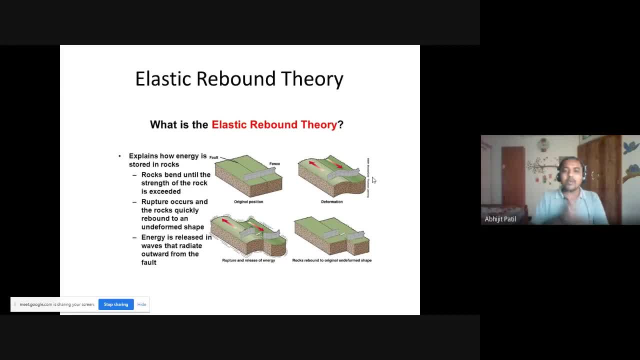 your why we uh rub our palms in case of winter season? because it generates heat. because of friction, it generates heat. so heat is a form of energy. okay, so what happens in case of rocks? so here there is buildup of energy, here there is tremendous buildup of energy. and because 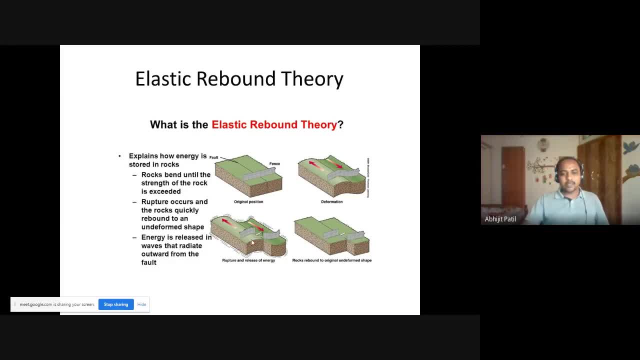 of that. there is sudden movement, okay, at the plate boundary, and that movement causes release of energy, and that release of energy is in the form of, obviously, heat and vibrations. okay, so these rocks, so whatever these lines are shown, these are nothing but vibrations. the rocks start vibrating because of that. 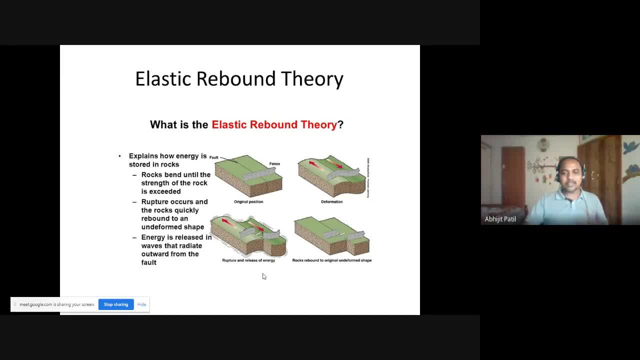 release of energy, okay. and these vibrations we call as earthquakes, okay. okay, try to understand that. and this elastic rebound theory. so again. so once this energy gets released, it doesn't stop again. the movement is. the movement is continuous moment of magma. so this will again start. so this cycle, 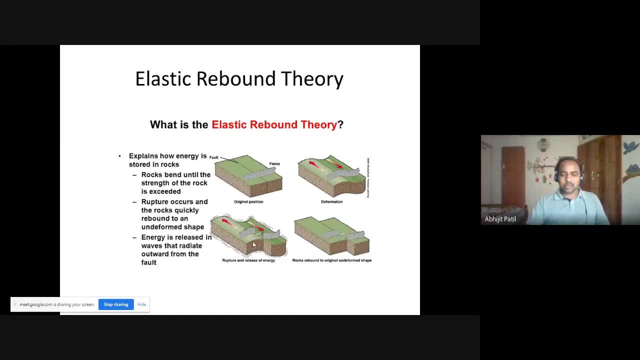 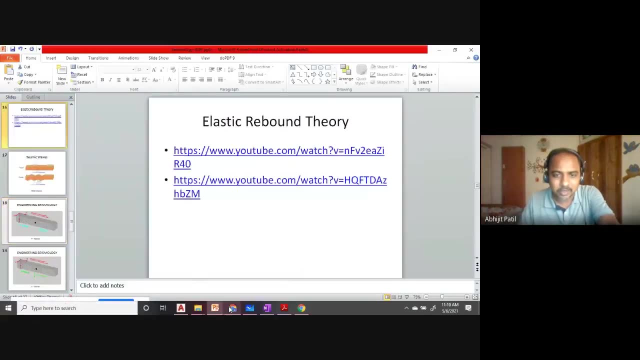 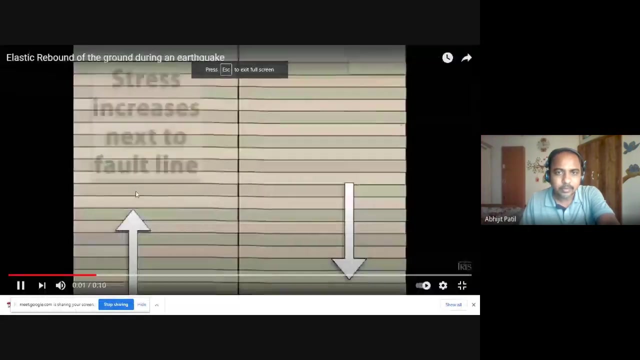 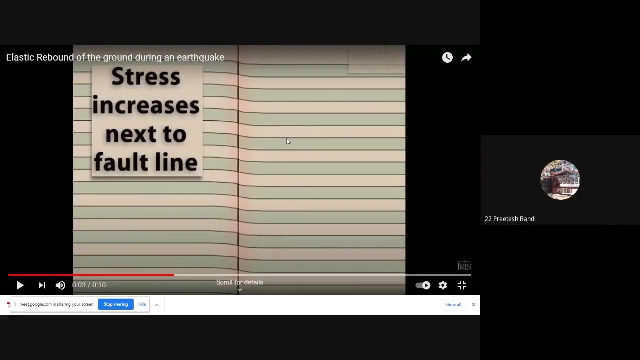 will again be repeated. okay, so this is called as elastic rebound theory. so the rupture of rocks, of the vibrations of rocks, everything is because of this release of, So this is the exact cause of earthquake. So let me just show you one small video. Are you able to see this screen? the video screen. 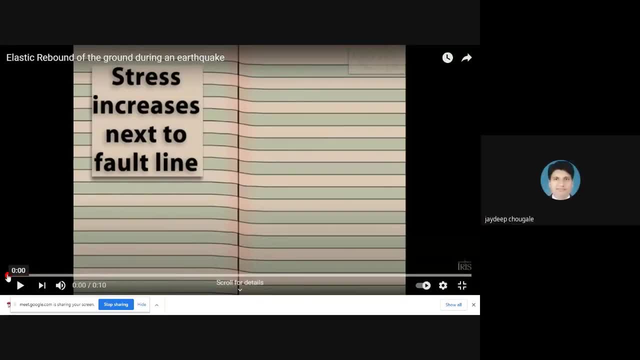 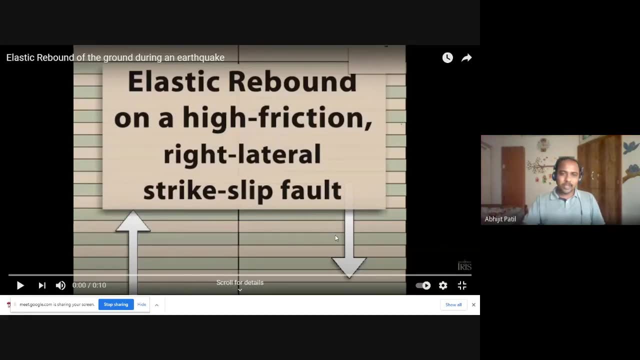 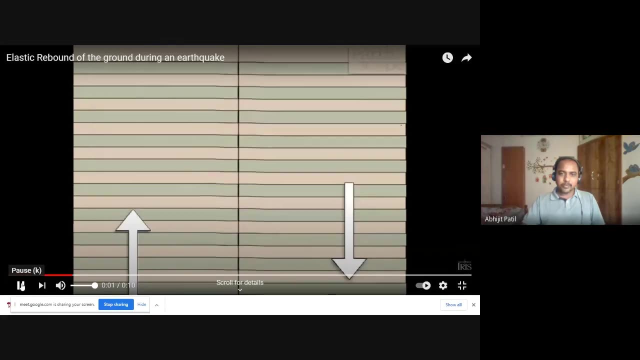 Yes, sir, OK, So I will just So. it is a small 10-second clip. So, whatever, this is one plate and this is another plate. So for reference, these lines are drawn, So just observe what exactly is happening. 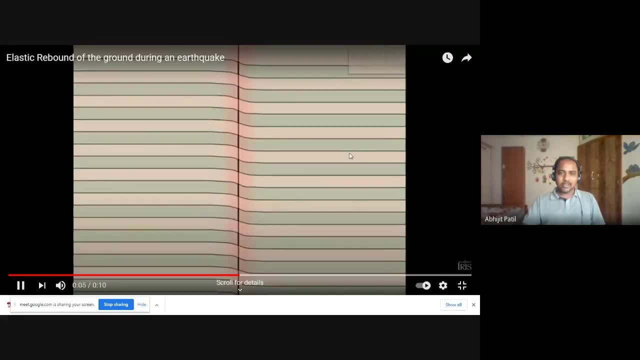 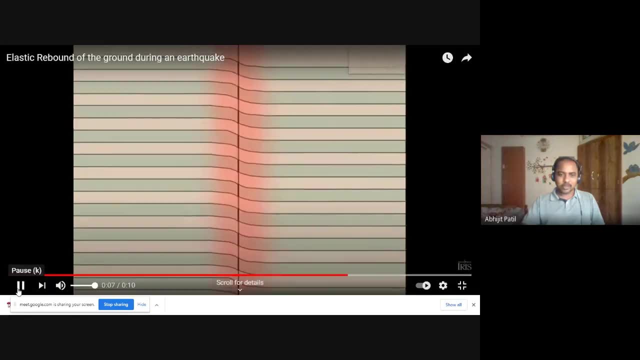 So movement in this direction, movement in this direction, stress concentration here And when this goes off, so at this location. let me just pause this. So at this location, you can see there is deformation of rocks here occurring, But the whole mass. 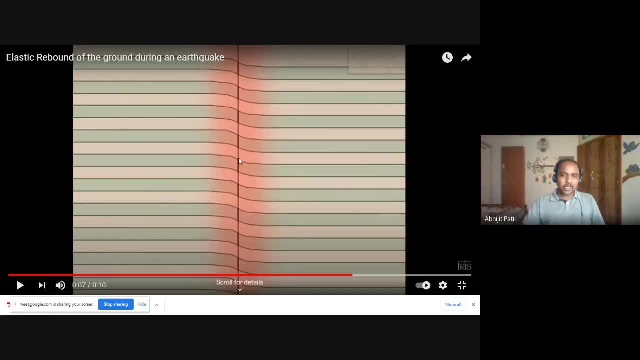 The whole mass has moved forward And this because of this attachment, friction between these two plates. the whole mass is under tremendous stress. So this red color indicates the stress level And at one point the stress is more than the friction between these two plates. 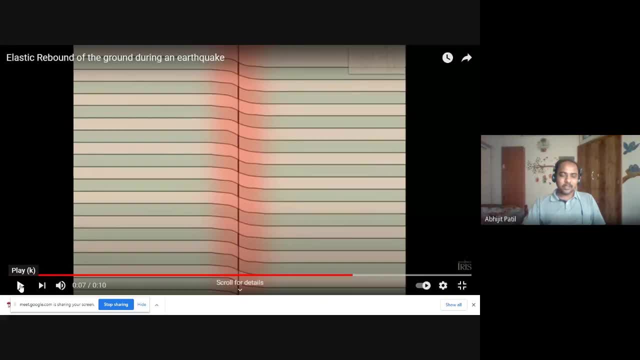 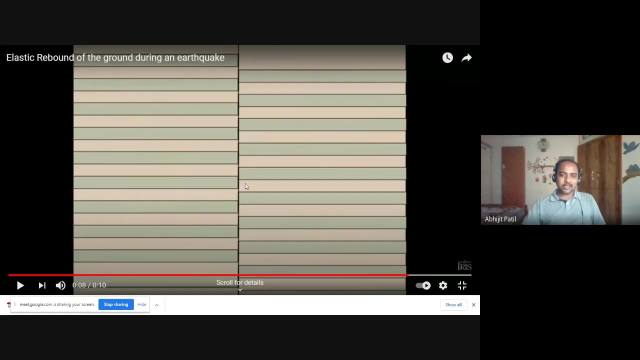 And at that point the energy gets released. But there is sudden slip. We call it a slip. Slip is what? Nothing but Your Displacement of the rock. And after that displacement, now these two were attached And now these are separated. 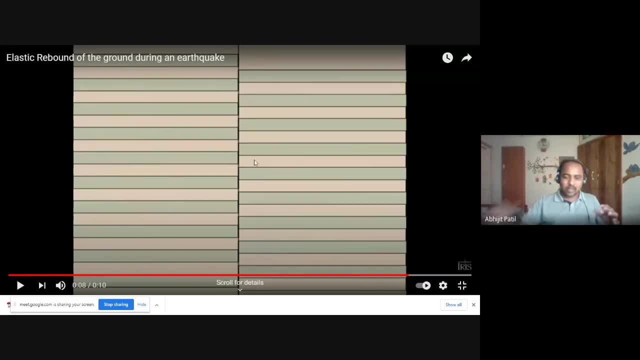 So at that instant you can imagine the South American plate and African plate. So they are under tremendous stress And at one point that stress gets more than the friction between those two plates And there is sudden slippage between these two plates. 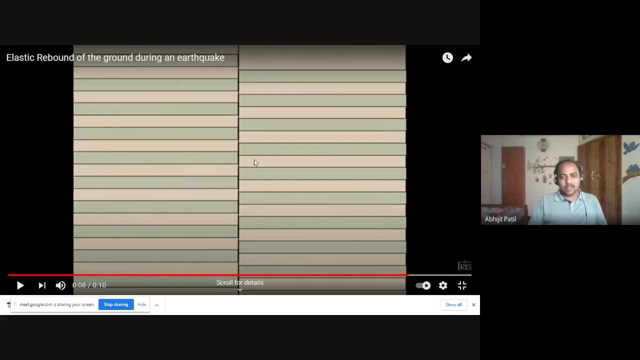 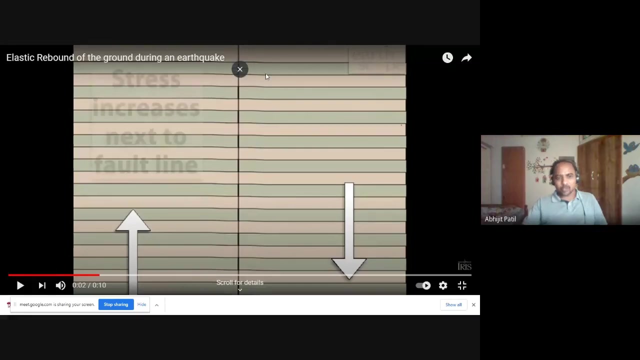 And imagine these two heavy masses involved in these phenomena, And there the energy gets released And the amount of energy is tremendous, And that energy gets transformed into vibrations of the ground And that we call as earthquake. So this is the cause of the exact cause of the earthquake. 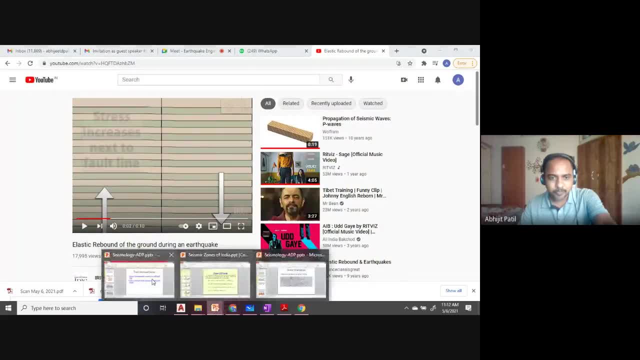 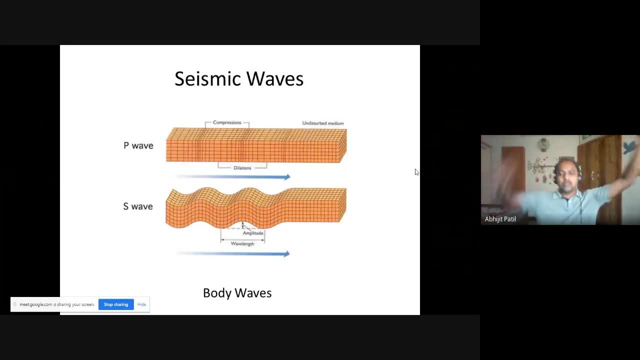 Earthquake, So we'll move further. OK, So we'll see the effects of the earthquake. Now we know the exact cause of the earthquake: Because of the plate tectonics and elastic rebound theory. in short, the earthquakes are generated. 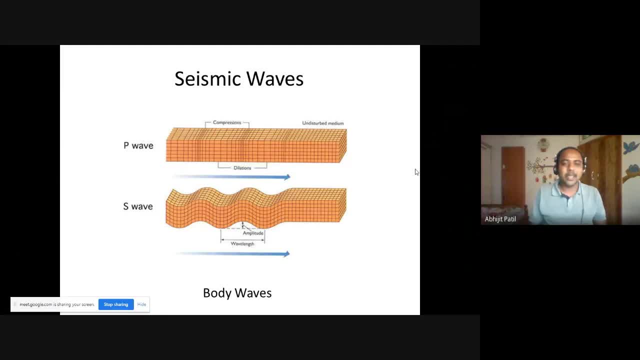 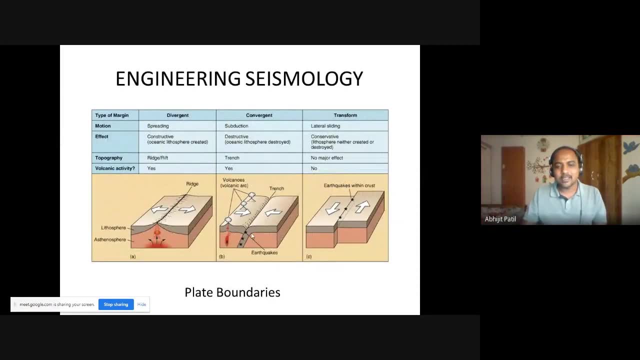 So when the earthquakes are generated, what exactly is happening? So sorry, I had told you to keep it short. OK, Let me try to come back to this. OK, So these are the stars where this slippage is occurring and the release of energy is occurring. 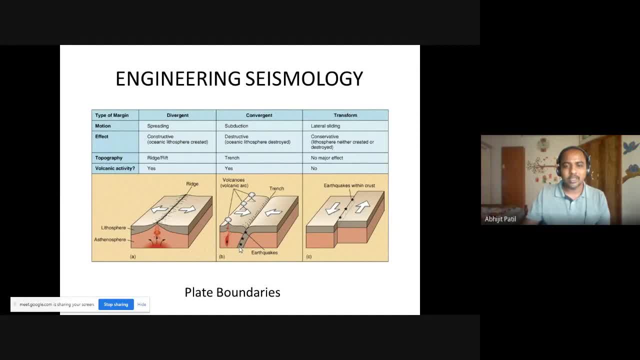 OK, So this star is nothing but location of the earthquakes. So usually this process continues And here the earthquakes will happen. So the Nepal earthquake which was around in 2015,, I guess. So that Nepal earthquake is nothing but example. 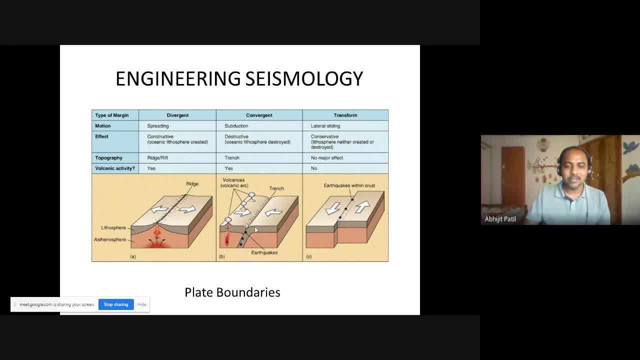 So that Nepal earthquake is nothing but example of this type of boundary and energy release. I will share the video. Of course, this is not the part of syllabus or scope of this lecture, But just out of curiosity. you can see that video. 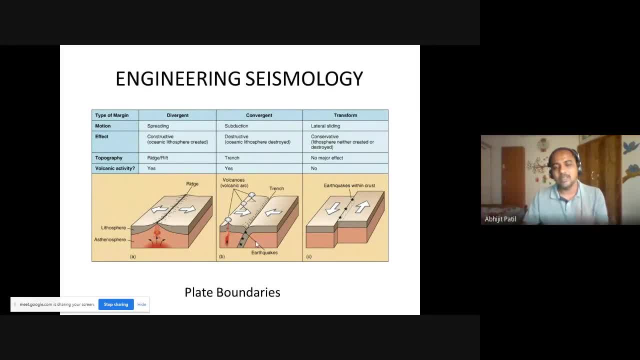 to understand the more details and more analysis of that Nepal earthquake. Now you understood the terms, the plates or plate tectonics, elastic rebound theory. Now you will be able to understand that video. OK, So I will share that later on. 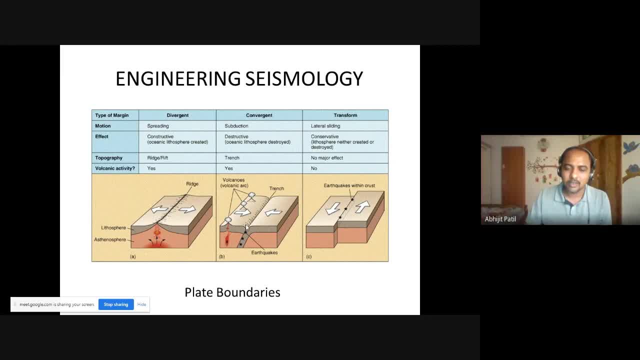 So, just if you are curious enough, you can go through that video. And this is so. you can see, the stars are not there here at the divergent boundary. So this means that earthquakes will happen at convergent boundaries and transform boundaries, And very less earthquake will happen near the divergent boundary. 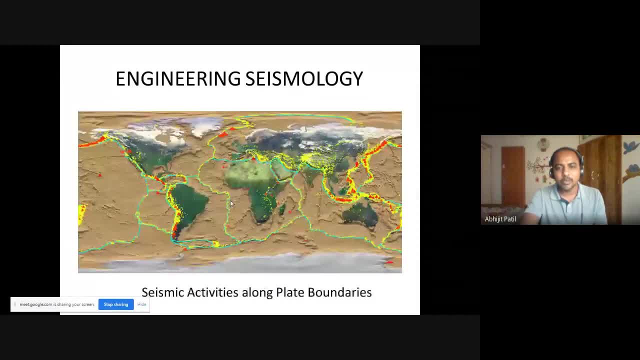 OK, And this is not a theory, This has been proved. So This image, which is again a map of world with plate boundaries marked And the yellow and red dots are nothing but seismic activities. OK, So the orange dots indicate higher magnitude. 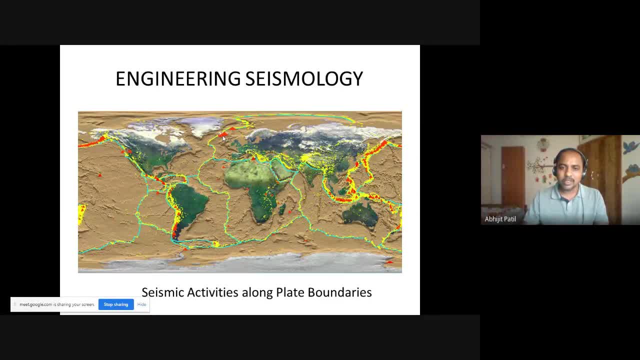 Now this term magnitude. I will explain. So magnitude is nothing, but it indicates the amount of energy released during the earthquake. OK, So this is nothing But magnitude. So if you say two magnitude or three magnitude, So two magnitude earthquake or, sorry, the amount of energy released in magnitude three. 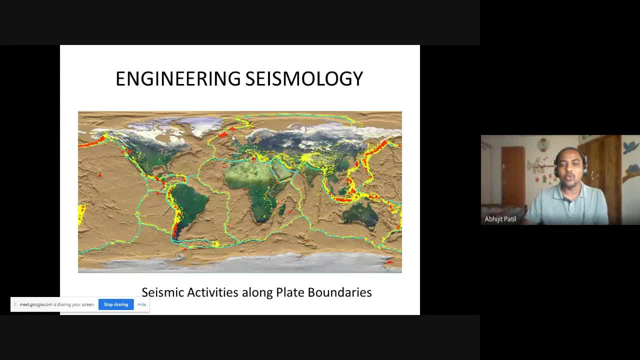 it's ten times more than amount of energy released in magnitude two, because that is a logarithmic scale. OK, So coming to the point, So you can see, we had seen that this is South Africa, South American plate And this is African plate. 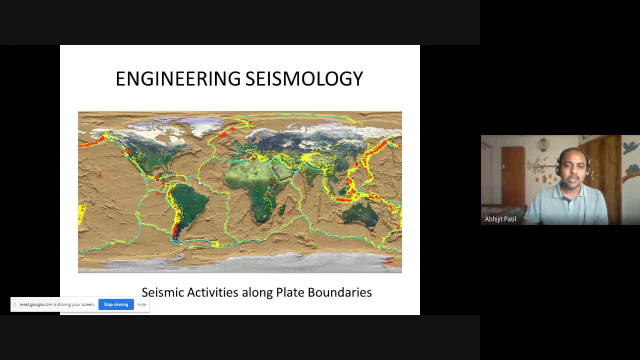 I wasn't boundary. You can see very few seismic activities. You can see Only the small, and that too, of low magnitude. the yellow indicates low. okay, comparatively, if you come here. so this is australian plate and this is eurasian plate, okay, so this is parallel boundary. transform boundary. 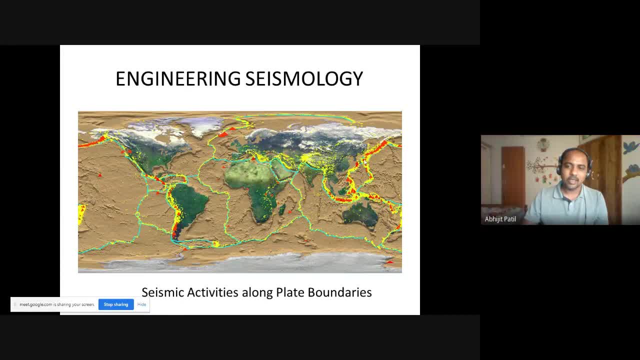 so here you can see, even here in the japan. so this is antarctica, sorry, pacific plate, and this is eurasian plate. so here also this is parallel boundary. so most of the earthquake activities orange or red dots and yellow dots also present, but more number of yellow dots are. 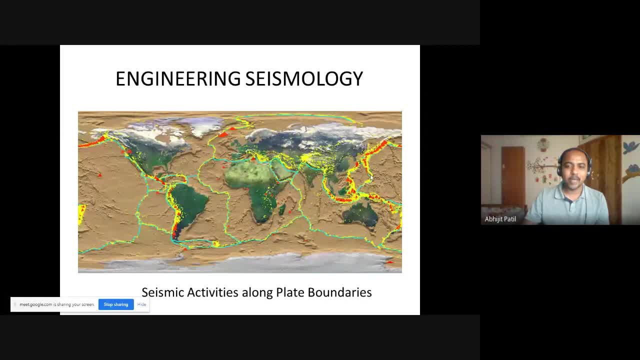 present as compared to this. so seismic activities are happening on this boundary. so the tsunamis in 2007 were because of the earthquake happened near java and sumatra, so that location is somewhere here. okay, so here also nepal earthquake. the yellow dots are more, but 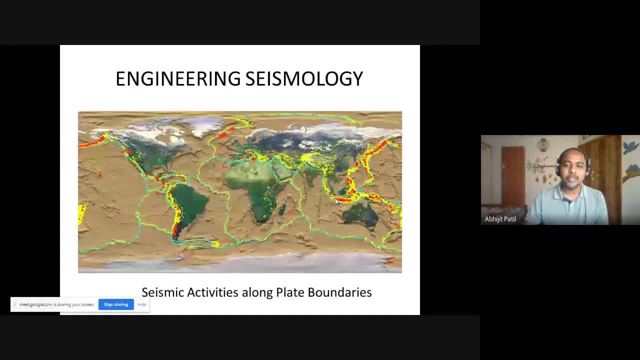 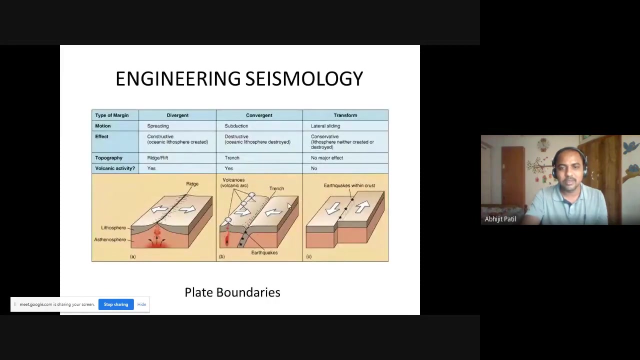 no large seismic activities are happening as compared to this. so, parallel boundary: if you try to arrange in descending order, parallel boundaries are more prone to earthquakes- then below that will be convergent and below that will be divergent. okay, so this is uh practical data. so from this we can prove this theory. this is what exactly is happening. okay, now 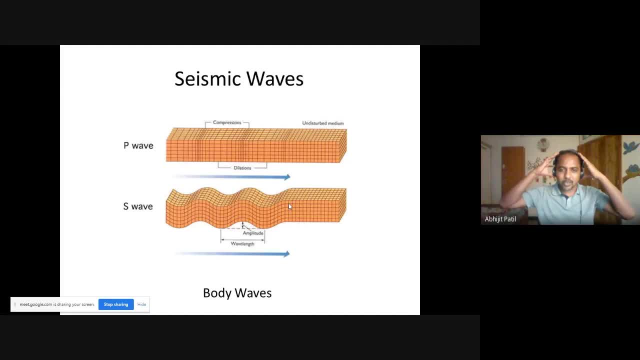 going ahead. uh, if you have any doubts, up to this point, because of time limitation, i'm going too fast. but if you have any doubt, we can discuss that or we can move further. okay, shall we move further? okay, so we will be looking after the effects of earthquakes because, as an engineer, as a 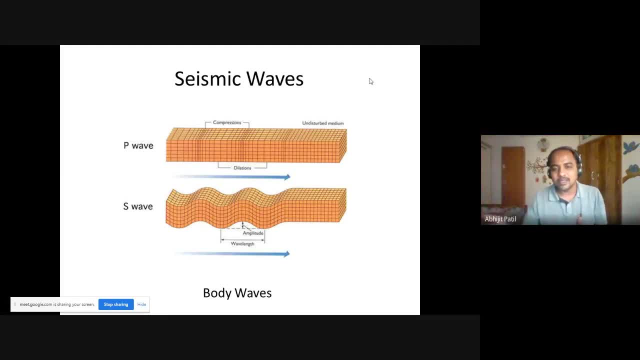 civil engineer or as a structural engineer, these effects are more concerning to us than the causes. of course. we must know the causes, then only we will understand the effect. okay, so when, as we have seen, the earthquake is nothing but release of energy because of the movement of the plates, 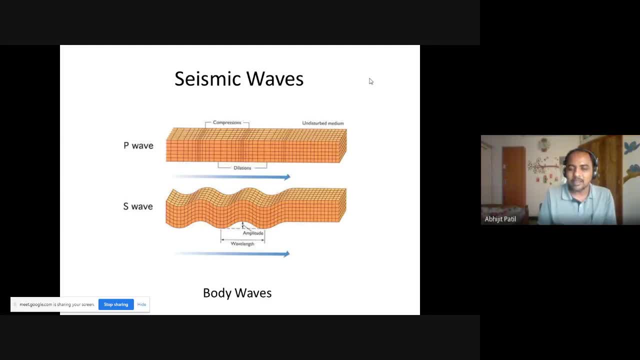 so this energy is getting released in the form of waves, vibrations or waves, and these are called as seismic birds. so seismic is related to earthquakes, it is. it comes from latin world, so sismo means earth, earth. okay. so seismic waves mean the waves which are traveling inside the body of the earth and as well as the surface of the earth. so earth waves you can call it. 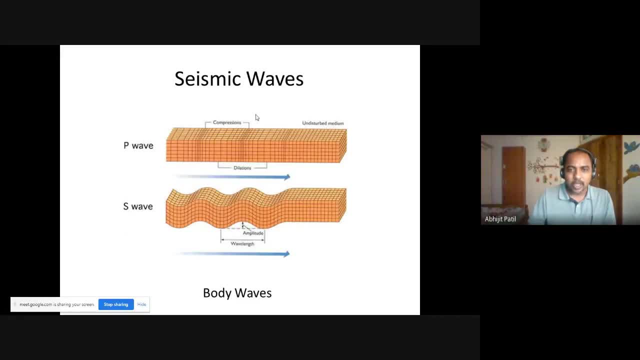 so there are two types of seismic waves after earthquake. so one type is body, where an another is surface value, so this one個 and another is surface value, so body wave, and this another is skin wave or surface waves. so the wave, so body wave. obviously, the waves which travel inside the earth's body are called as: 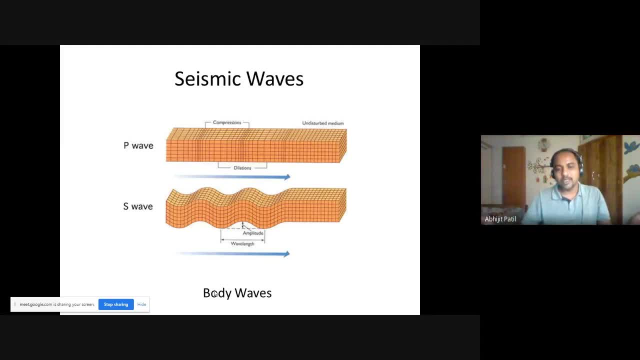 body waves and the waves which travel on the surface of the earth are called as surface waves. okay, so body waves are again of two types: p, that is primary wave, and s, that is secondary wave. so we'll just go through these small animations to understand what exactly is happening. 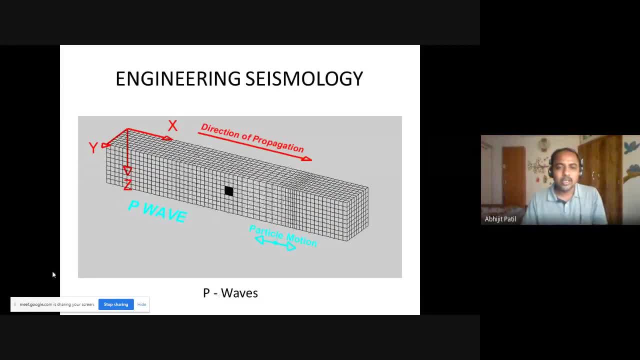 okay, so, uh, this is just uh, this, uh body of the earth, okay small. uh, just like in fluid mechanics, we consider a channel in the river to understand the properties of that whole channel. so we have taken a small mass of the earth inside the earth's body and we have divided that into 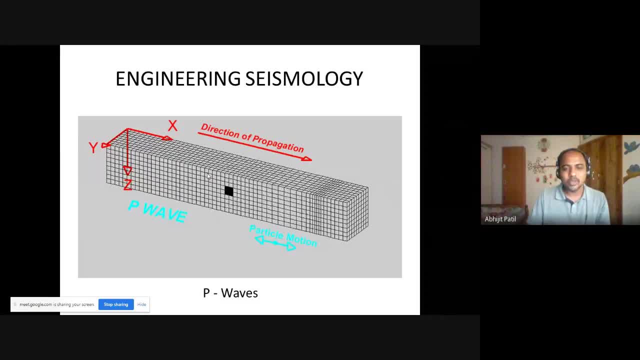 cubes or squares like this, and we are trying to observe what exactly is happening in case of p waves. so you just see, the p wave started from here, okay, and we will just observe this sample. so this is this black part is sample. so this will first compress and then get. this is the rarefaction it is called. 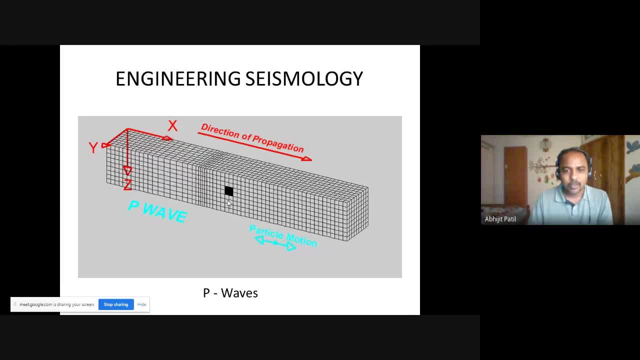 opposite to compression, rarefaction: compress and rarefaction. okay, similarly, what is the thing happening? this is moving forward, backward and original position. okay, so this is the particle motion forward, backward and coming back to original position. okay, so waves will pass, the remember, the body mass is not moving. 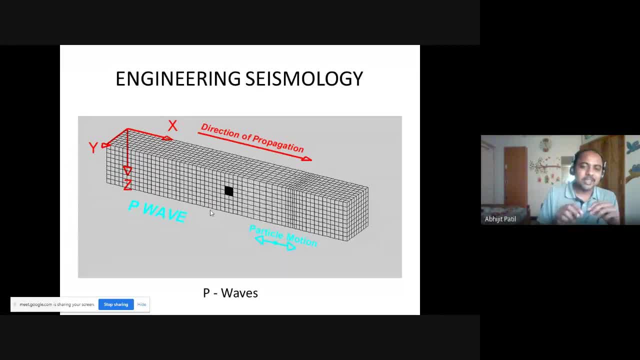 the body, body mass is present there itself, but it will vibrate. so what is vibration? moving? moving of any particle or body with respect to its mean position. so it will move forward, backward and come back to its mean position. forward, backward, mean position, parallely, it is getting. 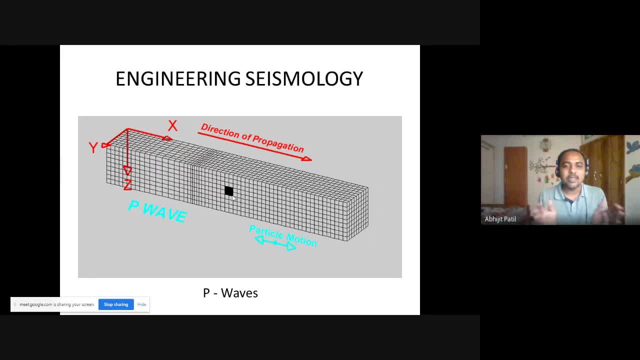 compressed, it is getting rare, reflected and again regaining its original size. okay, so this is what is happening. so the particle motion is in the direction of the wave, so wave is moving in this direction, so partially completed條 Universe in this direction will move forward. a rapidly visible for. 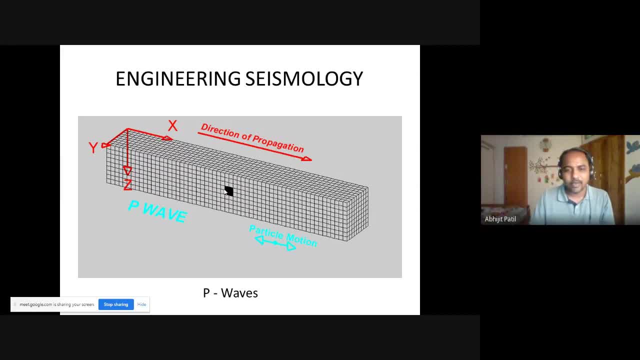 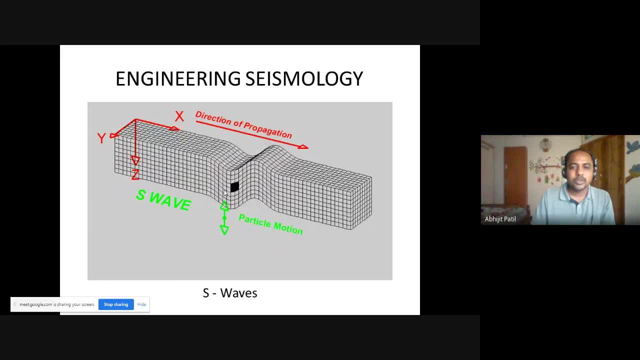 is also moving in this direction: backward and forward. so this is P wave. secondly, S wave. so you will be easily able to understand: the particle is moving in a direction perpendicular to the wave direction, moving upward, downward and coming back to its mean position. so this is called as secondary. 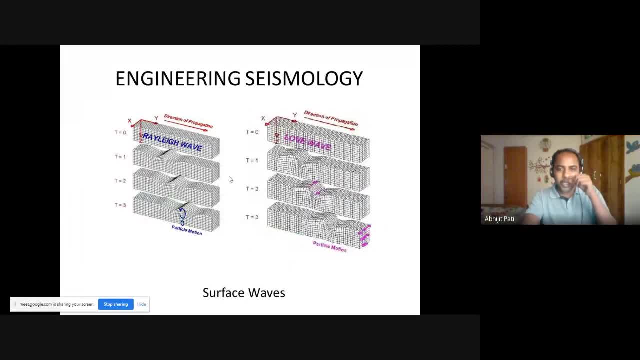 wave, then you have surface waves, so in that again there are two parts. left hand side, it is rally wave, so these are named against scientists rally and this is named against the scientists love. so these are two waves. okay, so this is the let me see. yes, yeah, I have animation, so rally will be just like a circular. 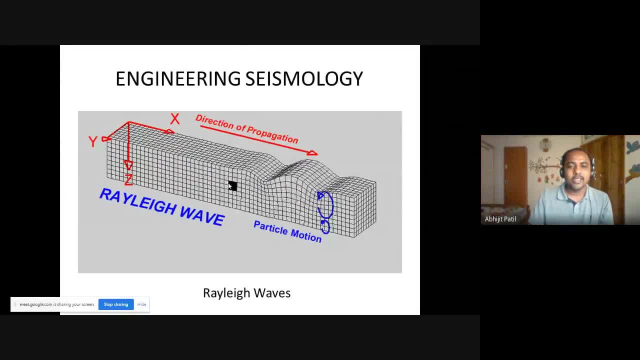 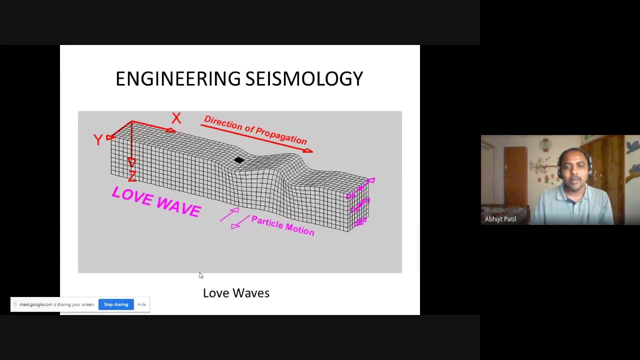 motion. okay, so the particle moves in a circular fashion and again come back to its original position. so this is the particle motion? no, circularly like this. so these are traveling along the surface of the earth and the love wave is like this. so the particle motion in a direction perpendicular, because this is 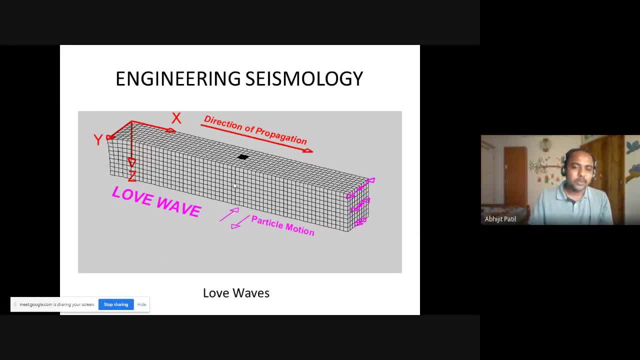 on surface. so what is the difference between s wave? so s wave was moving up and down and this is the lateral motion. okay, so these are traveling along the surface of the Earth, and the love wave is like this and the particle motion in a. this is moving side by side because it is on the surface of there, so it is just. 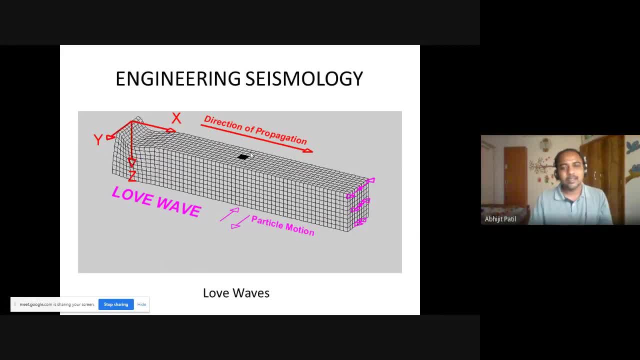 like the motion of the snake, okay. or if you tie one end of a rope and hold the other end in your hand and if you just give a horizontal flick, so the rope will show this kind of motion. so rope it's steady, rope is not moving, only the 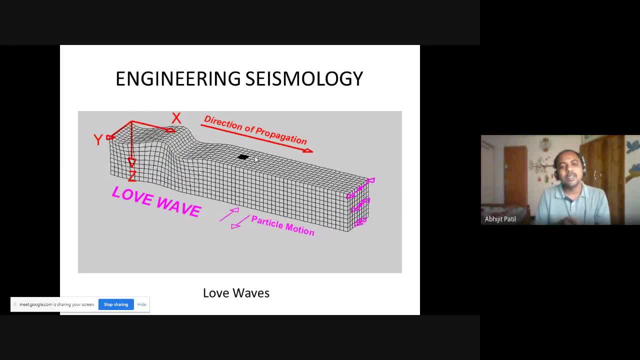 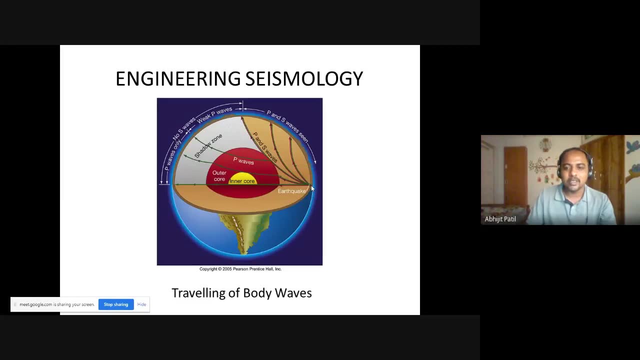 particles, a part of the wave, a part of the rope is moving left, right and again coming back to is or in position. okay, so these are the effects of earthquake. so this is how the waves travel. suppose the earthquake has happened here. okay, so the body various will travel inside the body of the earth's surface. so the P waves. 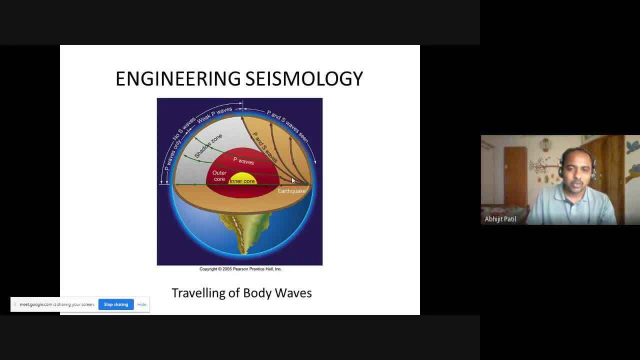 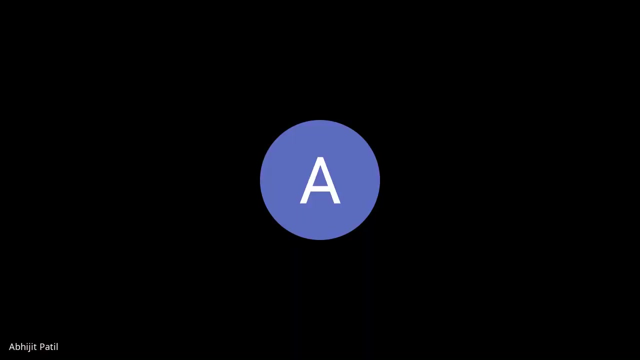 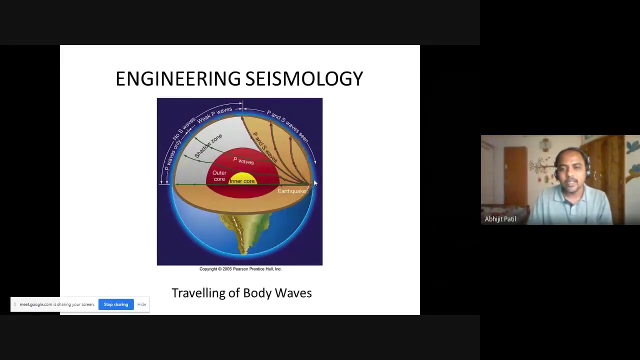 will travel like this, like this, like this. okay, they will also change the media. so just like refraction, so it will be having refraction like that. that means the angle will be changed and when the media again changes again the angle, when these waves reach the surface of the earth, so they will travel in the 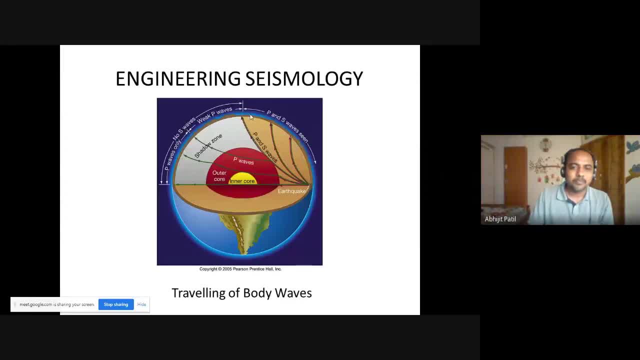 form of surface waves. okay, so you can see, the P waves will reach at any point on the earth. so if you see, this is the earthquake and it is exactly opposite of the point, opposite of the location of the earthquake, so there also P waves will also reach. but S waves will reach up to some point, the body waves, because 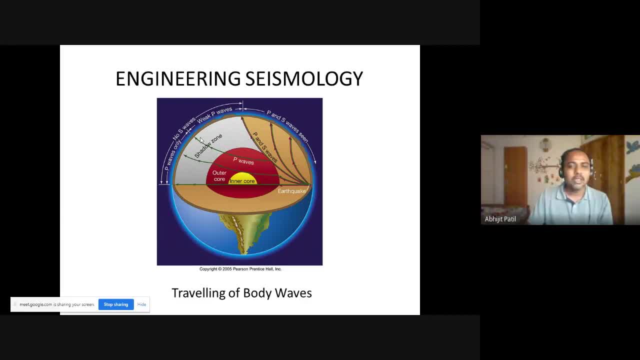 they travel through the body, so they will reach. P waves will reach. so anywhere earthquake has happened, the P waves will be received by all the parts of the earthquake. so earthquake happens at us, the P waves will be felt at the. of course, these waves are not felt by human beings, so these we have to have some. 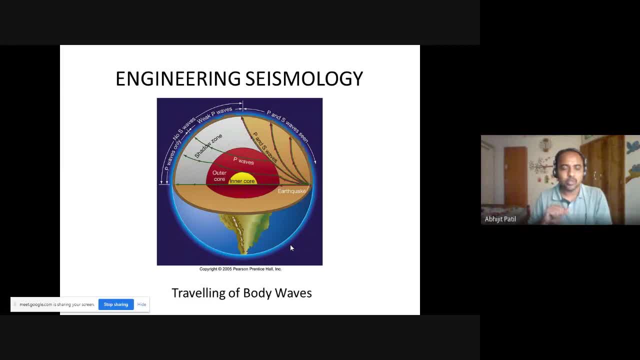 instruments to record those waves. so the instrument will record that, okay, but S waves will be recorded up to some part of the earth and the surface waves of also after some point. so, just like your, if you, if there is a steel lake, okay, no wind is there, it is still. and if you drop a stone inside that, so the S, the 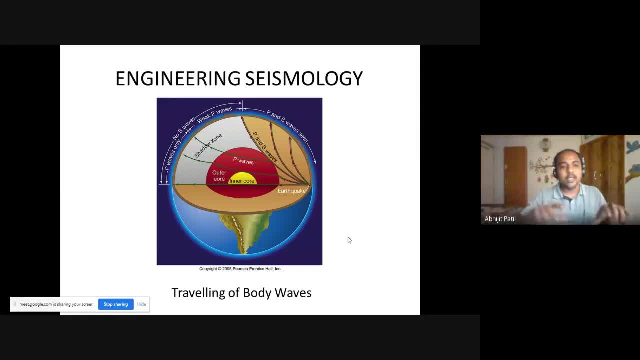 surface waves will travel along the surface and after some time, the amplitude. what is amplitude? amplitude is the amount by which the deformation is happening. so the amplitude will be more where you drop the stone and it will be less as you go away from the stone. so that is happening. what happening with? 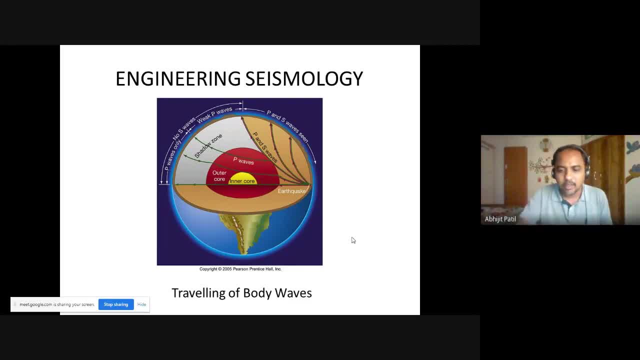 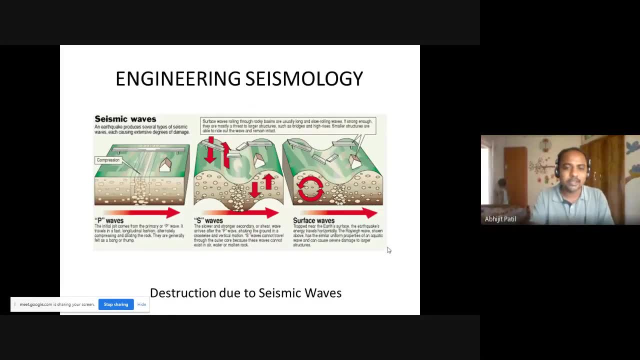 the surface waves. okay, so these are the effects of earthquake. so once we know these effects, we have to understand what exactly will be happening to our structures. so you see the P waves. so we are considering two types of structures: a small building and a long span bridge. okay, 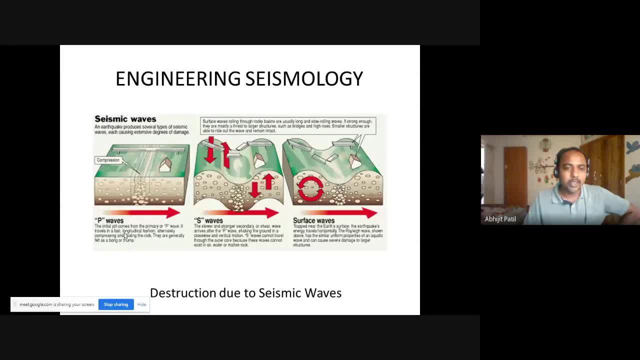 so the small waves, sorry, the P waves, we know they are moving like this compression, the refraction, so it will not have a very extensive damaging effect on the structures, whereas S waves though, it is a body wave, okay, some part will move up, some part will move down, so it will not affect building like 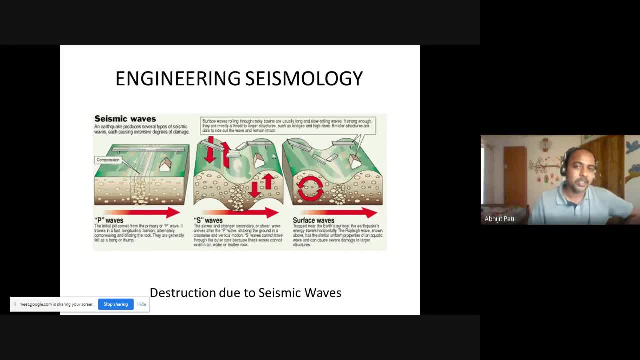 structures, but it will affect long span structures like bridge. okay, because this part is moving in this direction. this part is moving in this direction, so obviously the middle part will be under damage. so there will be. this is dangerous for our or this is affecting long span structures and the surface waves obviously are affecting 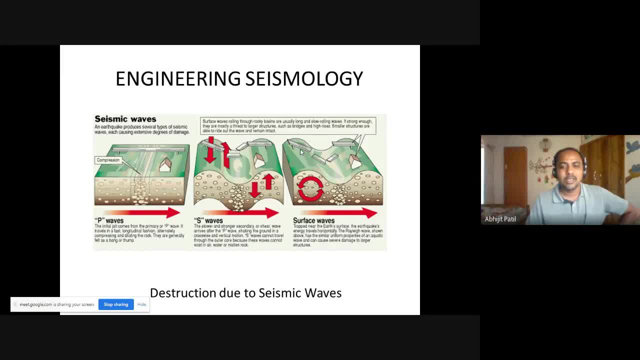 our buildings as well as long span structures. so if you see again in descending order, surface waves are more damage causing waves to structures and moderately damage causing waves are s waves and very low or literally no damage to because of the p waves. okay, so this is what is happening due to seismic waves. so we are more. 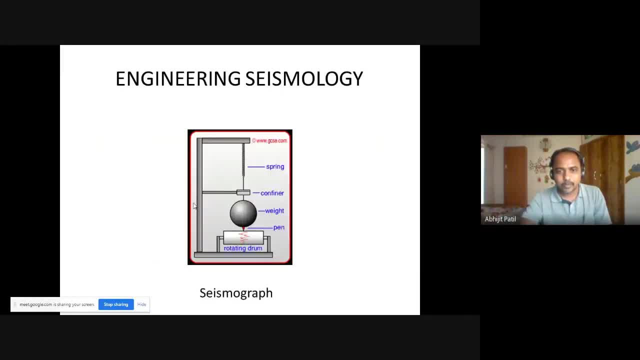 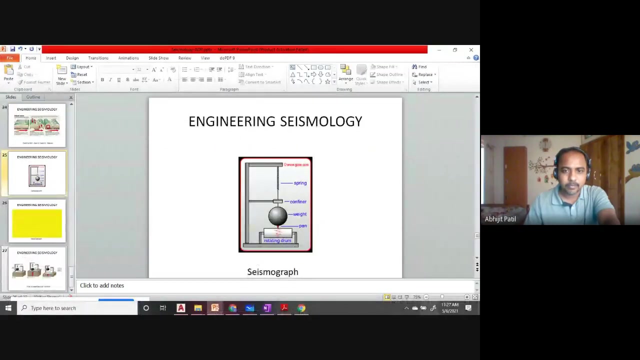 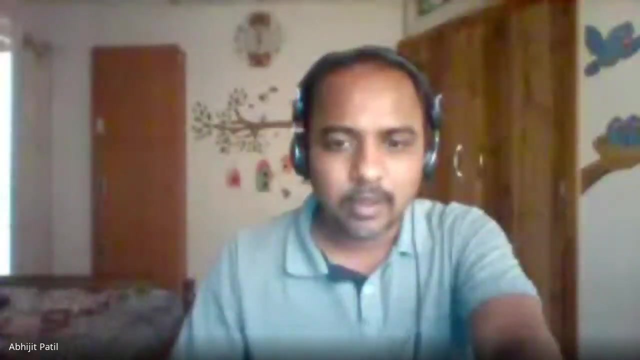 concerned about these effects now shortly, how the, as i said, how these earthquakes are measured. so we need amplitude for that, and then that amplitude is converted to some scale that is called as magnitude scale. so whenever you read in newspaper that this much magnitude, just a second you. 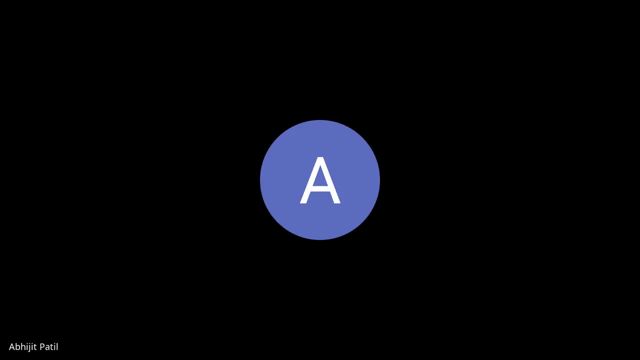 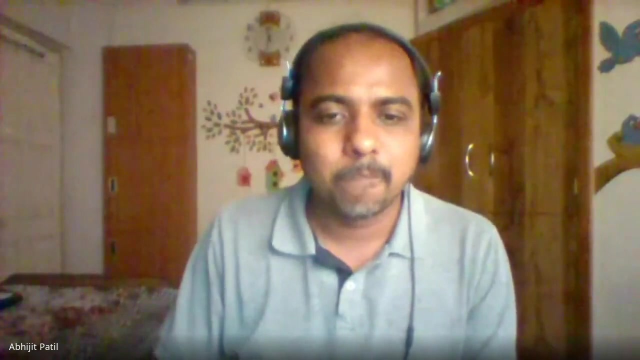 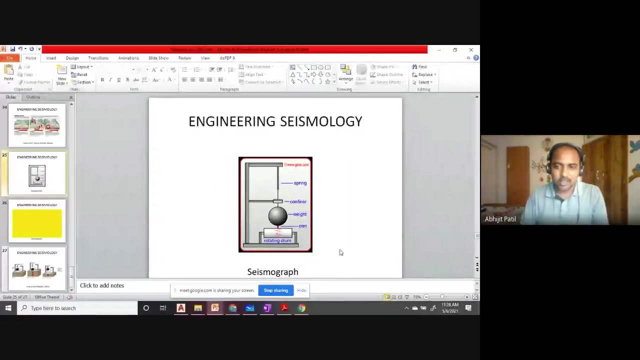 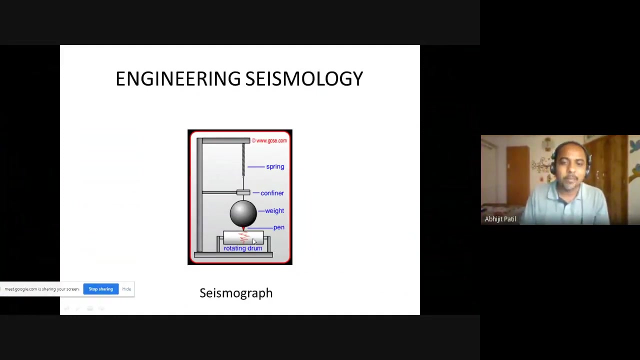 okay, sorry for the disturbance. uh, we will continue. okay, so we are discussing this. so, uh, the magnitude, the earthquakes are measured in terms of magnitude. okay, that is called a risk of magnitude and for that we need this amplitude. okay, so this is a simple mechanism which works on the 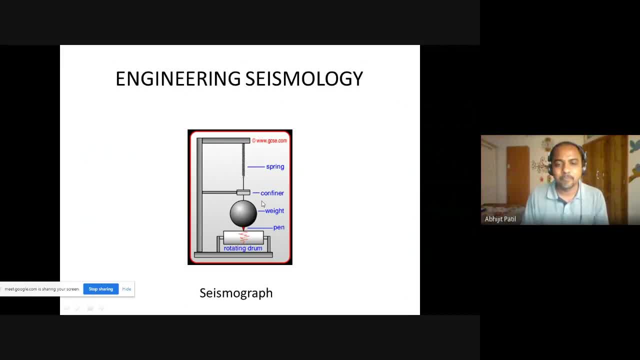 uh, principle of newton's second law. okay, so what is second law? the force f equal to ma, basically. so force is proportional to mass and acceleration. so what is done? this weight is very heavy weight is used. so this is conceptual. this is not actual instrument. this is conceptual. heavy weight is used, okay, and you have the other assembly. 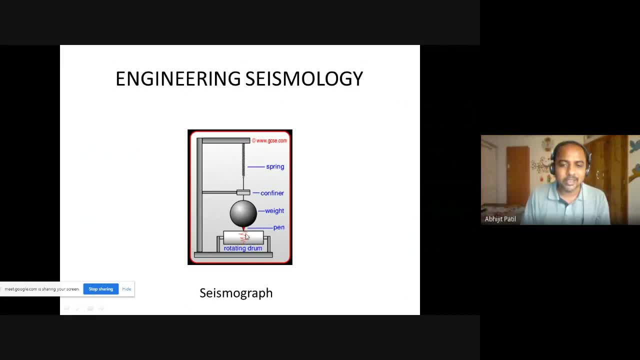 the rotating drum where it is. it is a recorder is attached here, the pen is attached here and the frame. and this frame is attached to the ground. so when earthquake comes, this weight is heavy. it is attached with a string or spring. okay, so this held assembly will vibrate with respect to ground during. 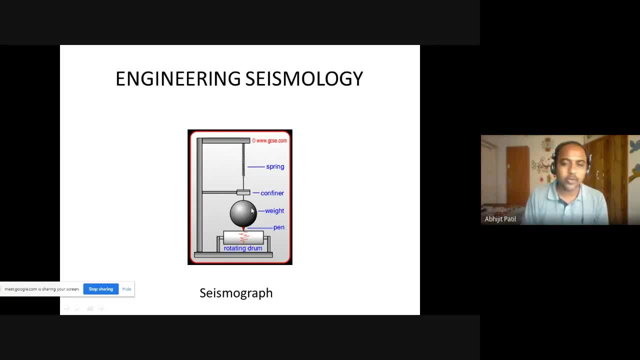 earthquake. but this heavy weight because of its heavy, because this will require heavy mass, sorry, heavy weight, sorry heavy force, f equal to ma. so since the mass is more, you will require more force to accelerate this mass. so literally there will be no vibration and this whole other assembly will. 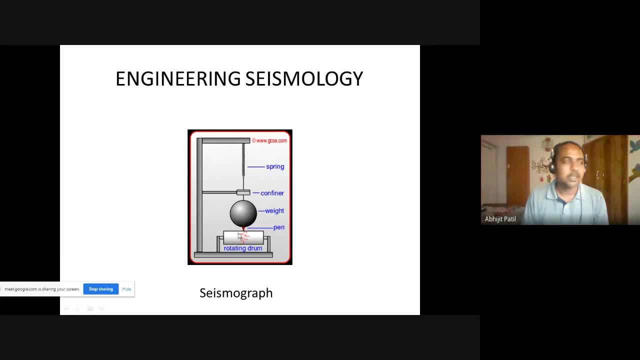 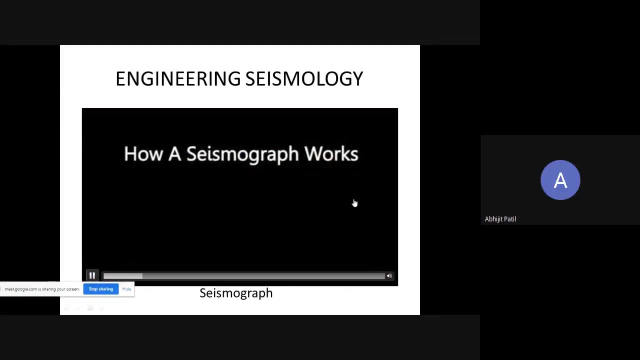 vibrate and you will record this on a recorder. so this is basic principle of a systemograph. so let me check if i have video. yes, a small video will explain this concept, how a seismograph works. a seismograph is an instrument used to measure the movement of earthquakes. 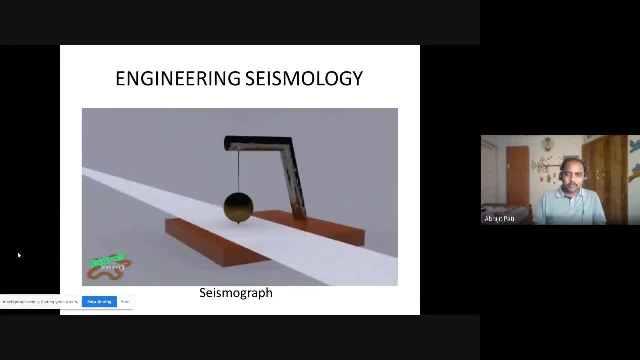 a weight is suspended in a way that allows it to remain still when the ground moves. most modern instruments use an electromagnetic mechanism for this. a writing instrument is attached to the weight, allowing it to record the movement. as it happens, the word graph refers to the writing action. most modern earthquake monitoring uses seismometers, not seismographs. okay, so this is. 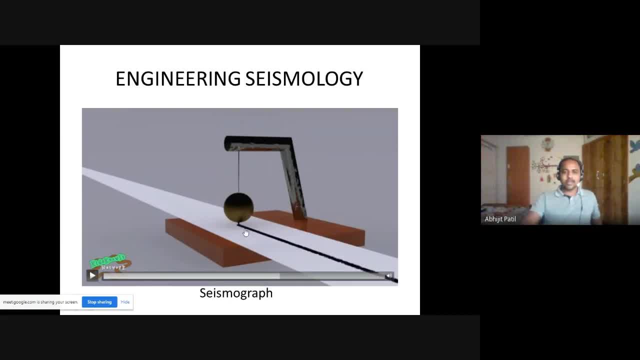 again conceptual this thing. so this paper is actually mounted on a rotating drum. okay, you have a plane attached here. so whenever earthquake comes, this whole assembly is having less mass so it moves with the ground. so this base is attached to the ground and this is very heavy mass attached. so it is basically 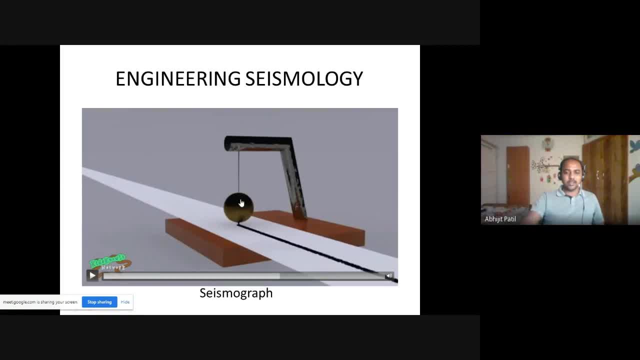 isolated from this frame, attached with a very small string so that this frame moves but this mass doesn't move and we get the record and record the movement of the earth. so this is just concept. but actually nowadays this electromagnetic seismometers are used and digitally or output the data to a seismogram. 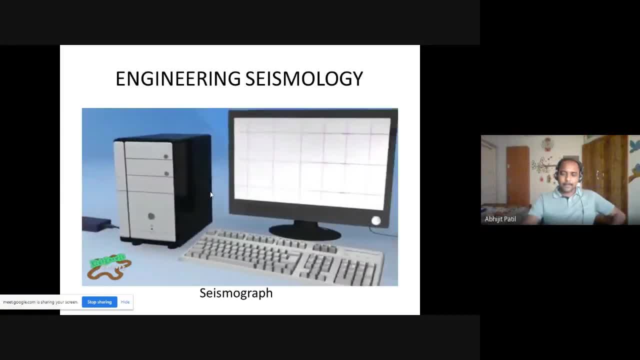 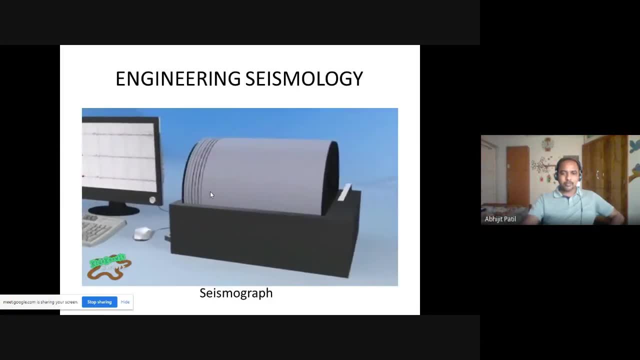 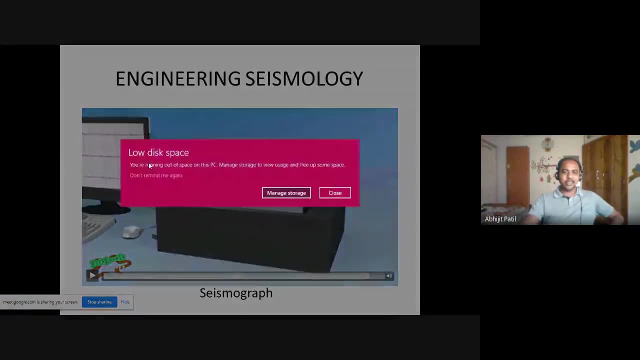 a printed version of the wavelengths on a large drum. these wavelengths that represent earth's movements are so small that in order for scientists to study them, they have to be amplified. okay, so this is how actual record. so this is a printer and this is monitor, where you get the record, so no need to store. 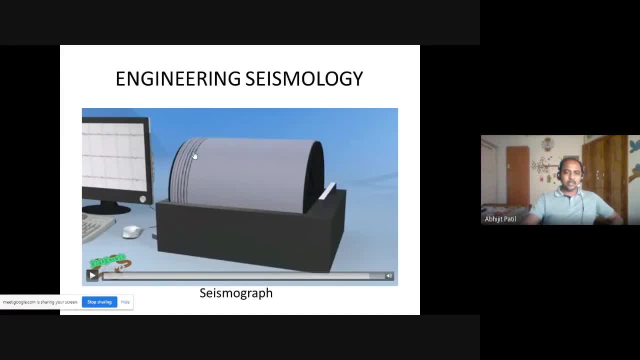 everything earlier days. you, we used to store the record paper first. we used to write Pennsylvania single data forき and there is a special certificate like these. so these data around primera méinity, holingbury visit, no to individual medical universities in all of these universities are like services, but basically, instead of 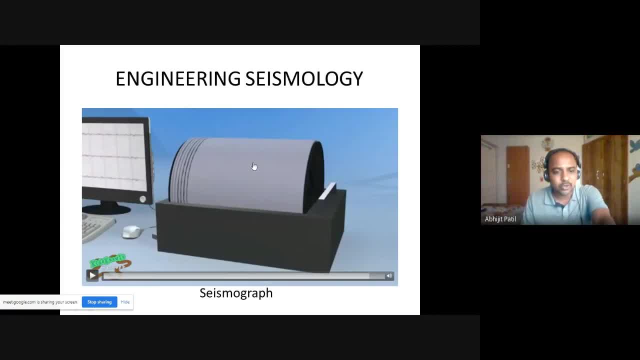 which there are every kind of closed customers like this. it is basically leveled 까�: sudden special Vaijit go to pregnancy, informs whether you have forks and i will see oashes. this study was field Cairo hospital and the device like this here is the. 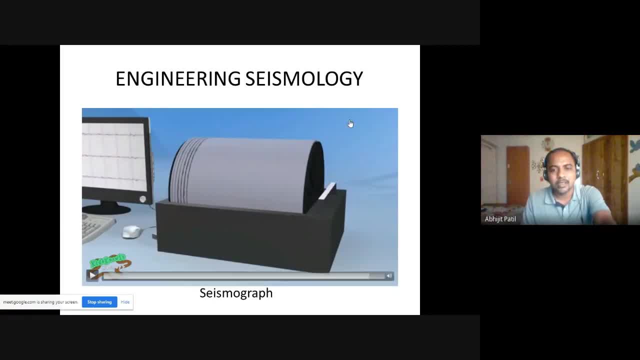 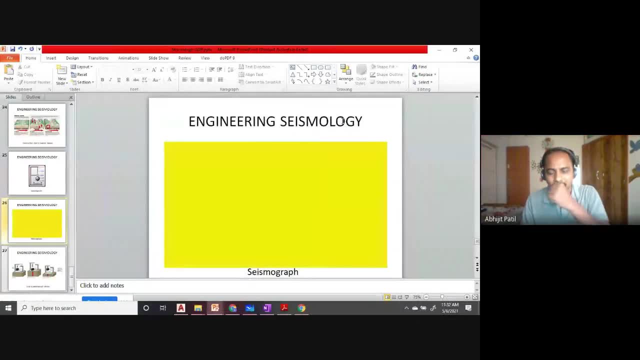 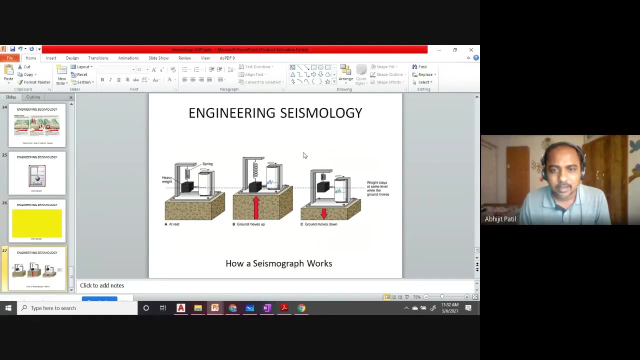 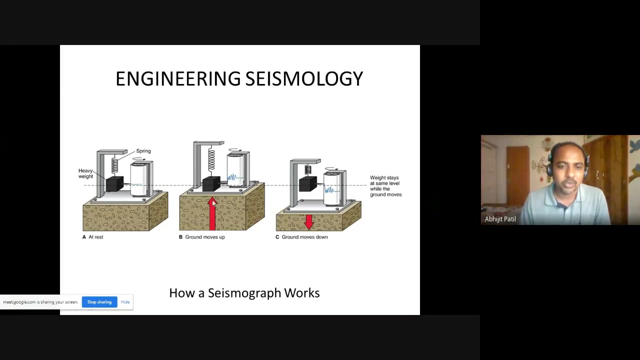 medical industry is theacia's question. first강 nächste 문제는, researchers- is that there is a when, an auto akkoron. so for research purpose, if you opt for mtech or phd, so there you will require this data and there you can get that earthquake records. so this is just for measuring the vertical motion. 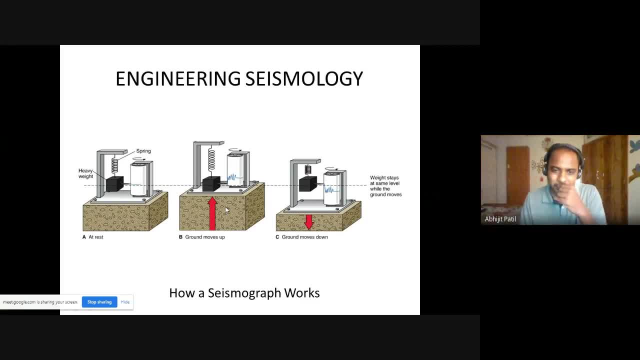 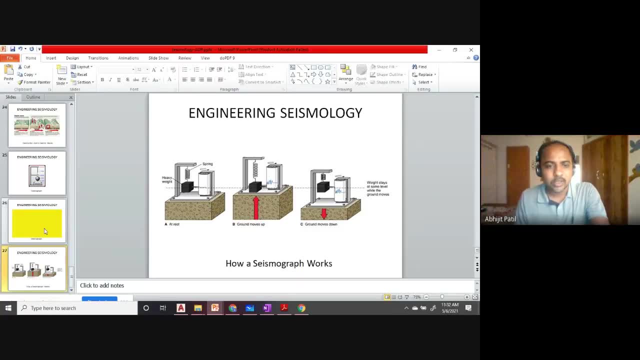 so only the assembly is somewhat changed. so there you can measure the vertical motion like this. okay, so this is all about seismology, the effects of cause of earthquake, effects of earthquake, the waves and how the earthquakes are recorded in very short, okay. in continuation with this, if you have any doubts, you can ask. it's just a small. 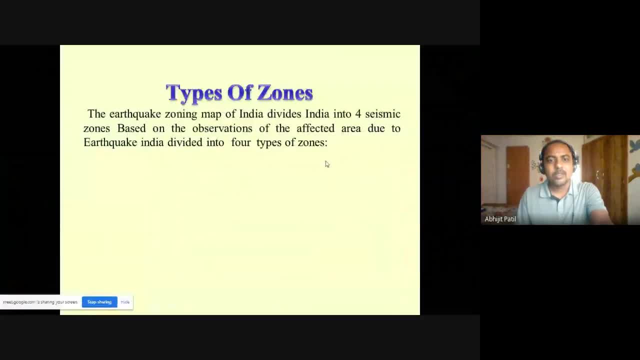 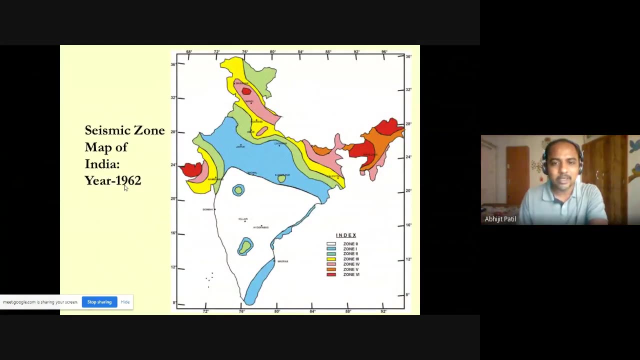 question. also, you can ask any question. okay, so you will. we are talking about india. so india is basically divided into four, uh, seismic zones. it's what is seismic zone. i will just go to the map. so this is very old map, 1962 map. so, uh, it was basically zero to six, so seven zones were there. 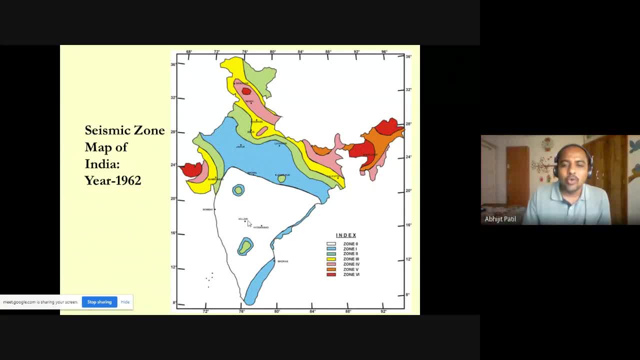 so what is this? uh, the lower the zone, the lower the probability of earthquake happening and the lower the probability of an earthquake happening. so let's talk about inside the air, into that zone. so, if you see, this is zero zone. this is old map, 1962 man. so that means the probability of happening of earthquake will be very. 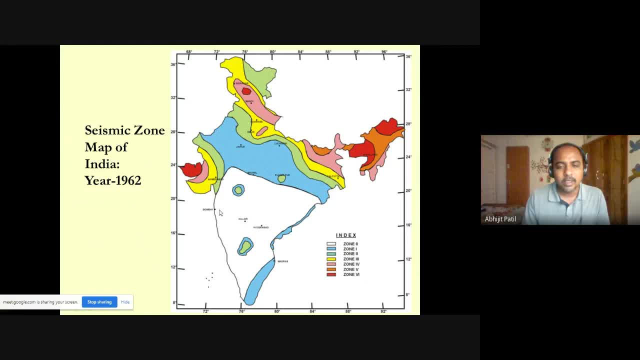 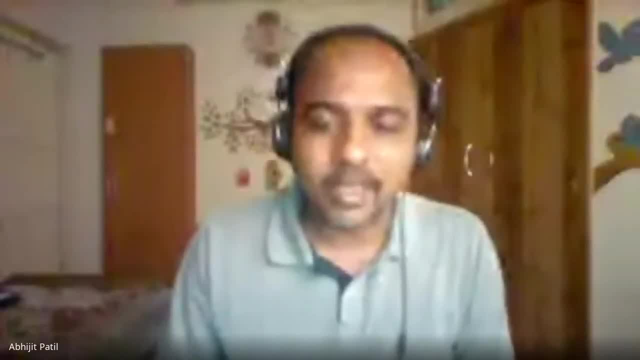 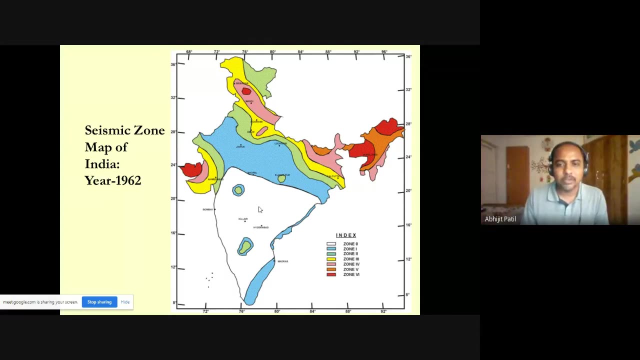 less, and that too will also be very, very, very less. and if you go to this red zone, so if you see, this is not history, so that means here the, if you remember, this is Nepal region, so this is all Himalayan range, so here you will see the higher. 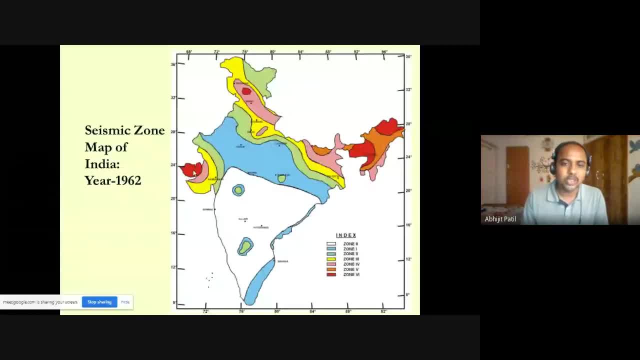 zones are present. here also, there is some higher zone, so the 2002 booze earthquake is from this location. okay, so here the probability of earthquake happening is more, and the magnitude of those earthquake will also be higher. so this seismic zoning map. earlier it was like this: 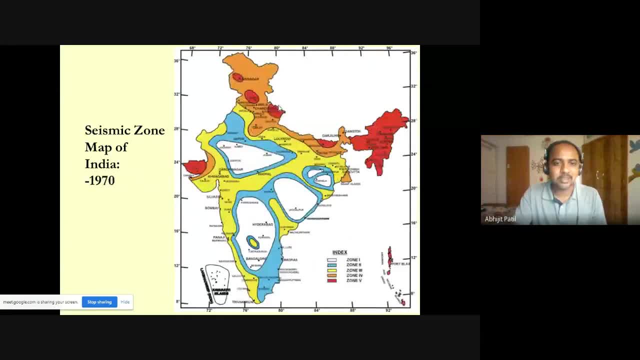 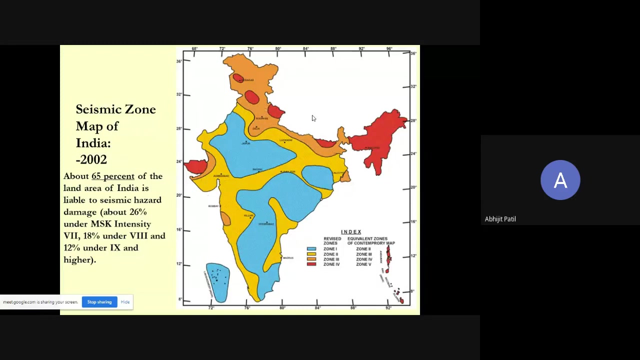 then the zones were revised in 1966, then 70. so why this division was happening? because earlier there were no records. so as the number of seismographs or seismometers were installed, we got more records and we modified the graphs. so in 2002 it was revised after the booze earthquake. so if you see, there was. you zone 1, 2, 3, 4, and now 1 is merged into 2, so we have zone 2, 3, 4, 5. so no zone 1 is present and again in 2016, after the Nepal earthquake, the graph is revised: it. 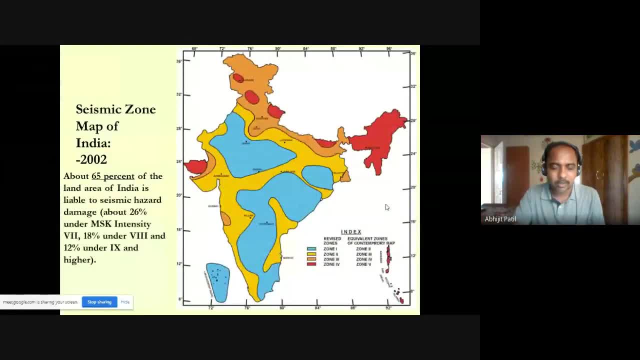 is like this. so basically the if you see the zone maps are not revised, almost same map is present. so if you see this, okay, I just wanted to focus here. so in 1970 I have received this audio infrastructure and I make it as the ev估 2b overexposed. 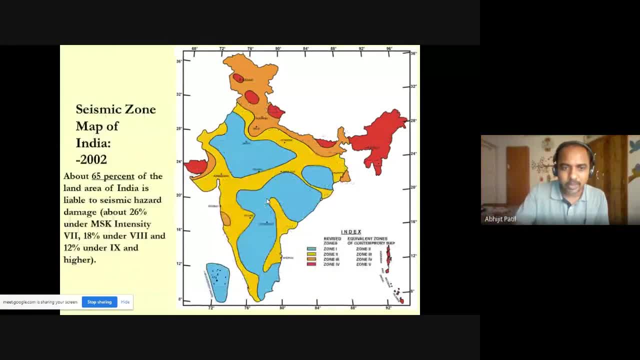 a question about that and it just appeared something that happened. we see soon that the flashing lights will be lit up when top downtr Spa Bridge light up, so we can see that the changing current, while the fifth shit is burning, which is the Devon hills vide you will see already. so this is PV 48. you happened. 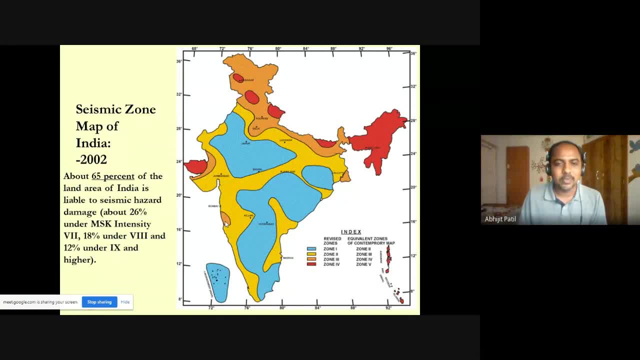 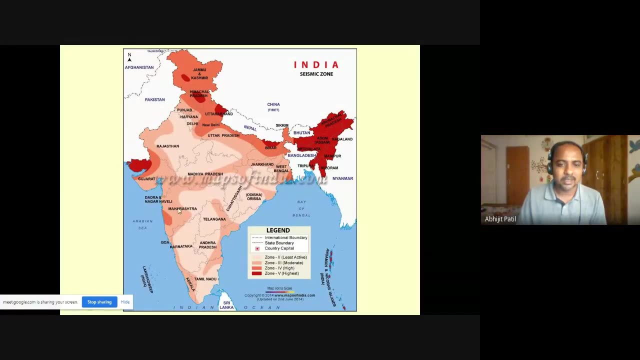 to look more photo. lemme quickly where fruit line: 32 nautical days, 21g, commander land in 2016. otherwise whole of the Maharashtra is in zone 3 or 2. only this thing is in zone 4. okay, so I am showing this, so this is available. in is 1893 the. 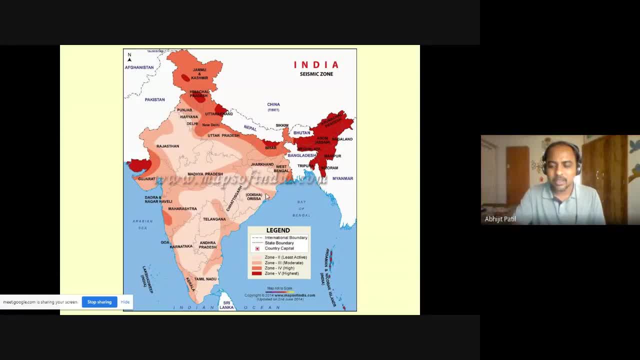 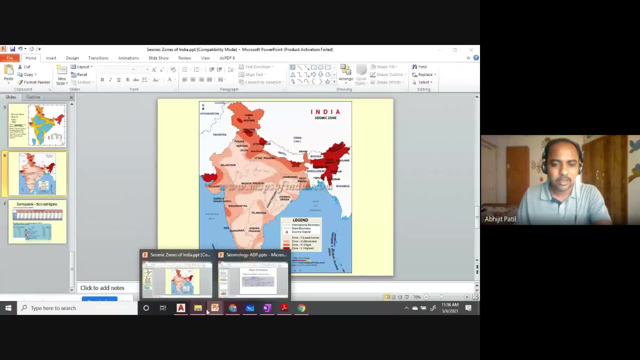 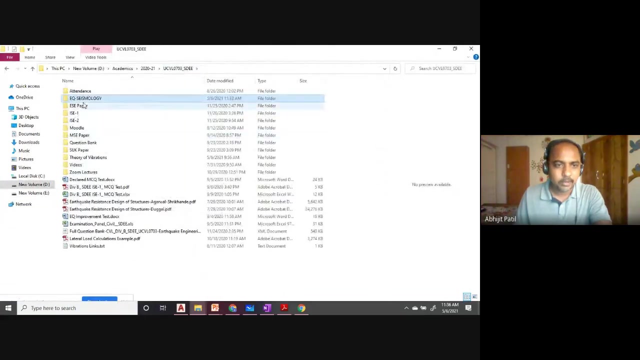 ice code, from where we will be referring to calculate the earthquake force. so this is not required. so this is the seismic zoning of India. so we will make use of this map when we are solving the numerical, so moving further. so, although theory of vibrations is not a part of your syllabus, but I will just explain. 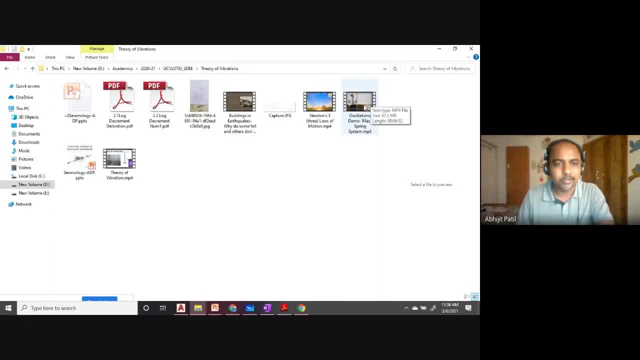 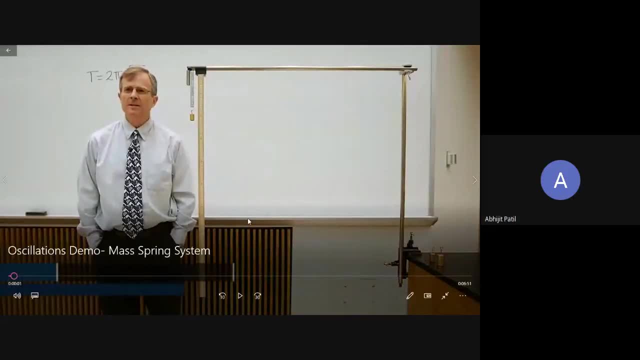 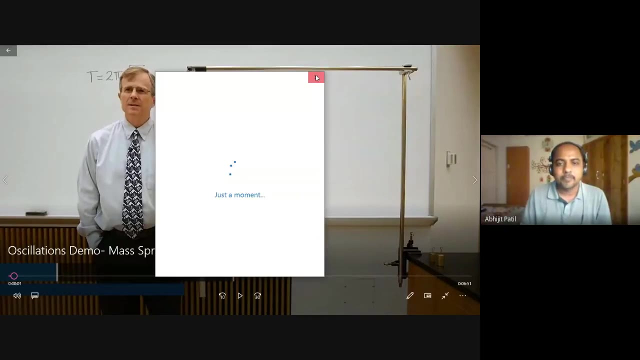 shortly the concept in 10-15 minutes I want to illustrate. so this is this: these videos are available on YouTube, so you can also see this. so basically, what to see from this video? the mass and spring model. so I will explain the analogy of this or application of this. 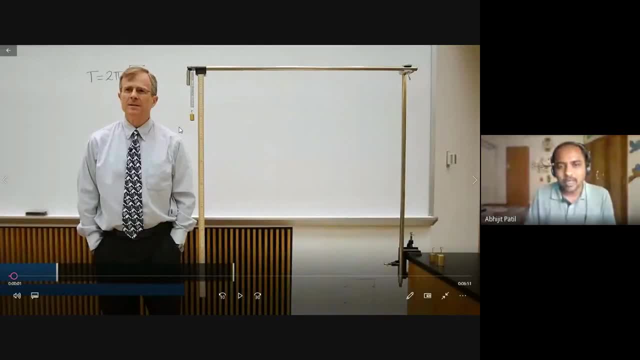 inbuilt thing later on. okay, but try to understand this mass and spring. what exactly is happening? the time period below this board. he will discuss the time period also. so this is very good demo to understand the dynamics. structural dynamics, so basic soft structural dynamics, so I'll just not. 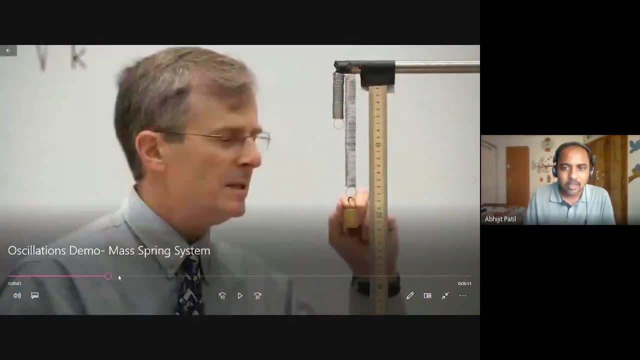 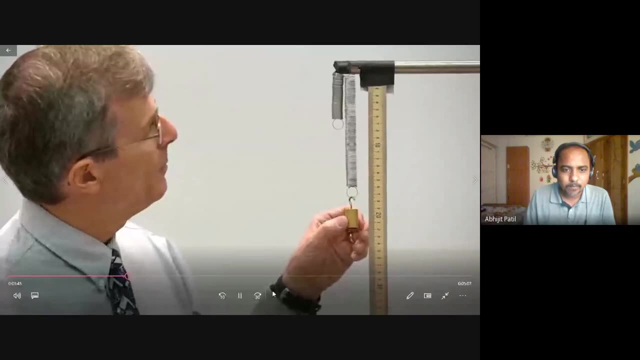 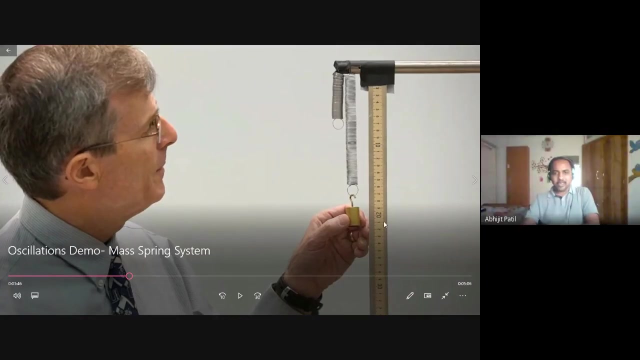 show you full video. you just of excursion from with an amplitude of 1 centimeter. I'm gonna want to move this, okay. so this is a spring and this is a mass and there is a small scale attached here. so how the vibrations. oscillations mean vibrations, so how these vibrations. 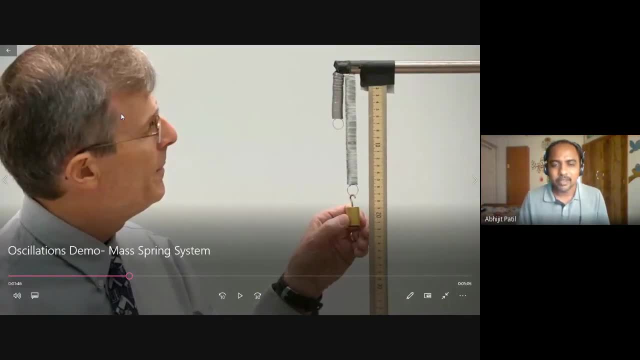 are happening and what is the relation of this vibration with the time period? okay, so we will understand what is time period. so time period is nothing. but when a body moves in a, just like what we have seen in p waves or s waves, the particles move in. 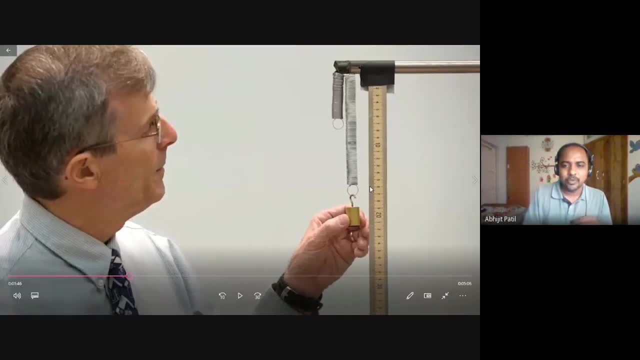 one particular direction repeatedly. okay, so when this repetition is there, we call it as vibration or oscillation. so there is a particular time period for that vibration. so to complete one cycle, that means the particle is at stationary position. so just like this mass, so this mass will move. 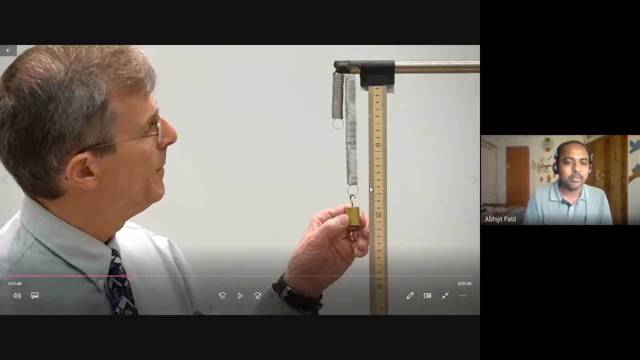 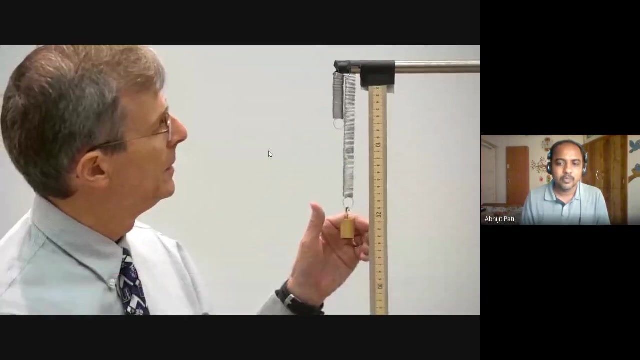 below, then above and again come back to its minimum position, so that one cycle, uh time required to complete that one cycle, is called as time period. so we'll just understand that concept here: mass one centimeter up and release it, and so now it's oscillating roughly between 18 centimeters and. 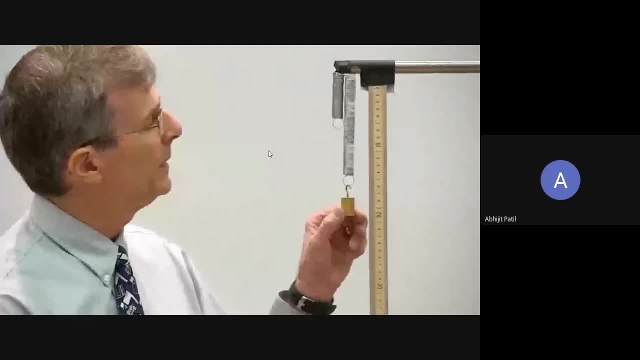 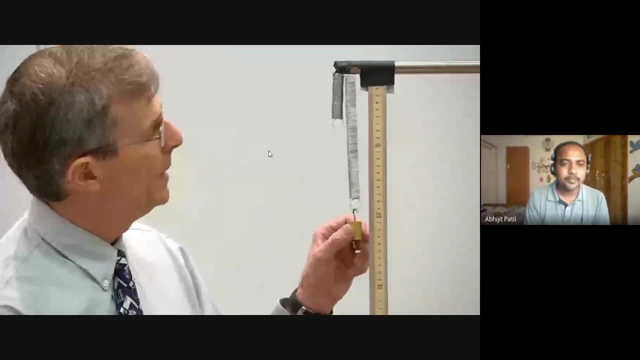 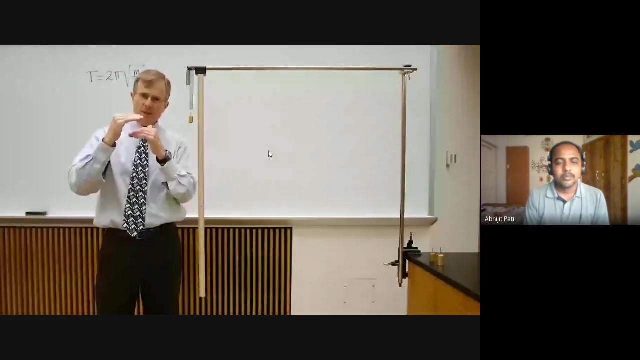 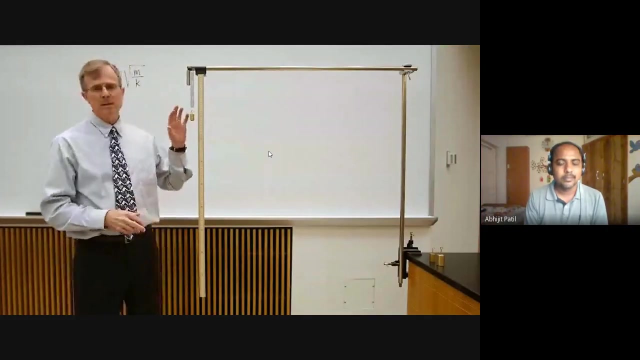 i could have done the same thing by moving it down to 20 centimeters, and then the overall motion is still two centimeters from top to bottom, but only one centimeter between the equilibrium position and one of the maximum positions. so now we want to look at the dependence of the period. 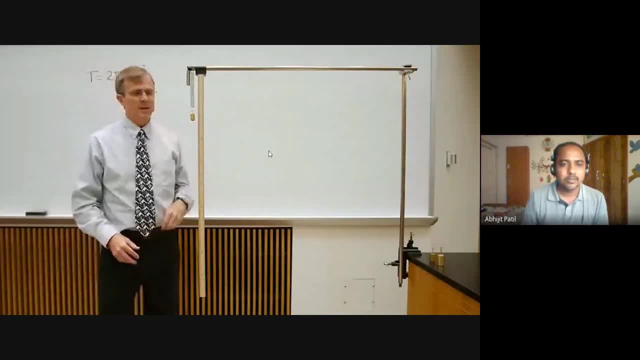 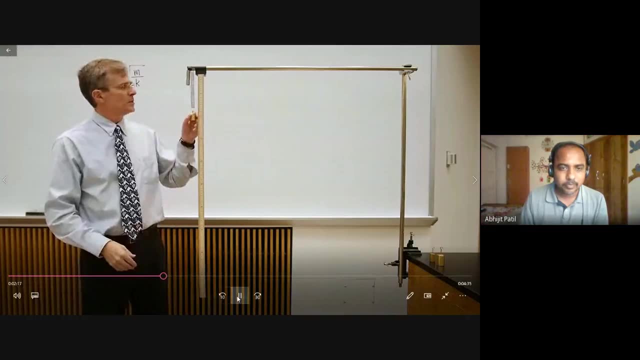 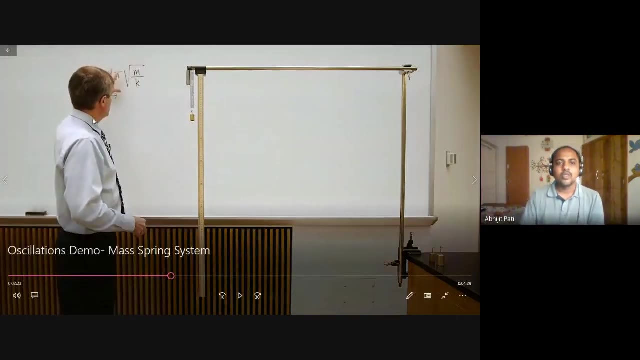 on the mass and the spring constant and also the amplitude. first uh, first the amplitude screen, constant positions. so now we want to look at the dependence of the period on the mass. okay, so you see, this uh t is nothing but time period. two pi under root, m by k. so this is the way we calculate the time period of any system. so let it. 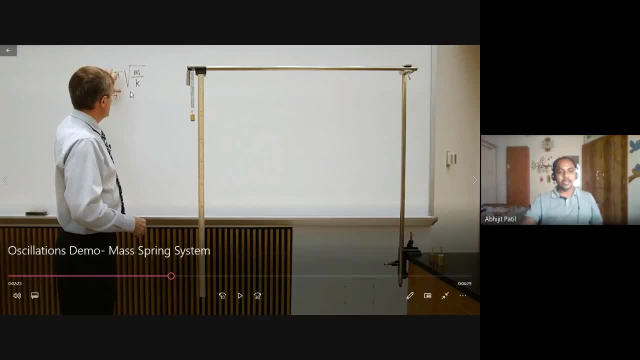 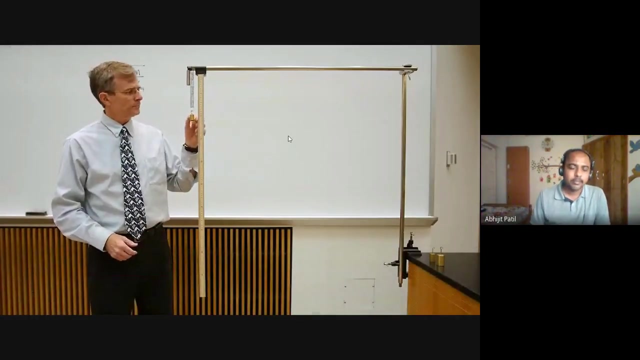 be a mechanical system like this: mass and spring. or let it be a building- okay, so this is universal formula. or let it be a pendulum, so this, uh, is an Lydia looks like. so you can see that the on amplitude and let me look at a couple of different amplitudes. here's a fairly 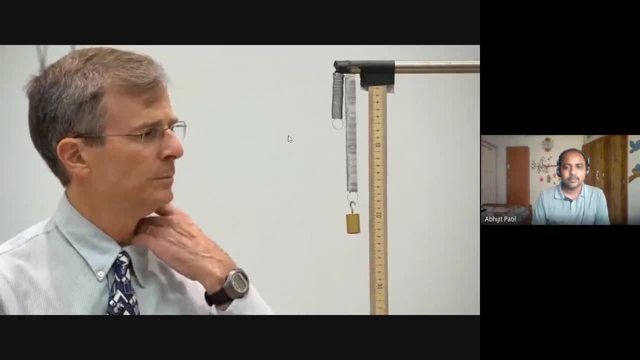 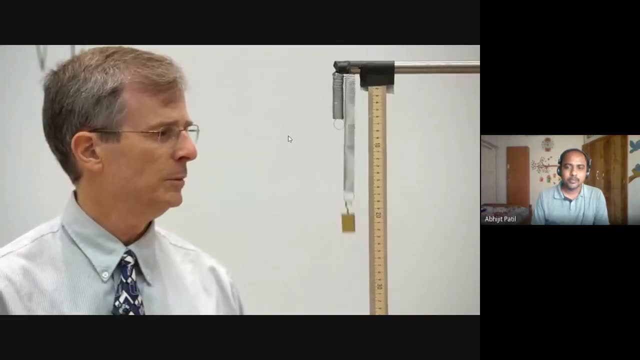 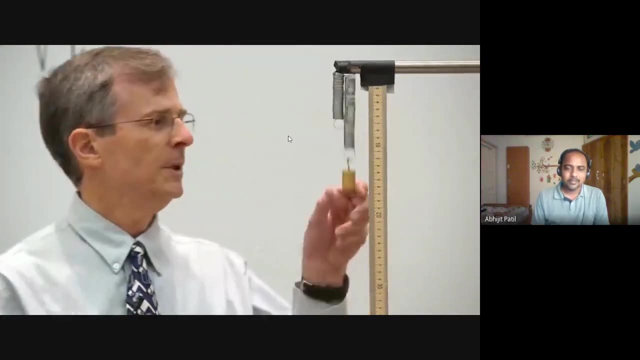 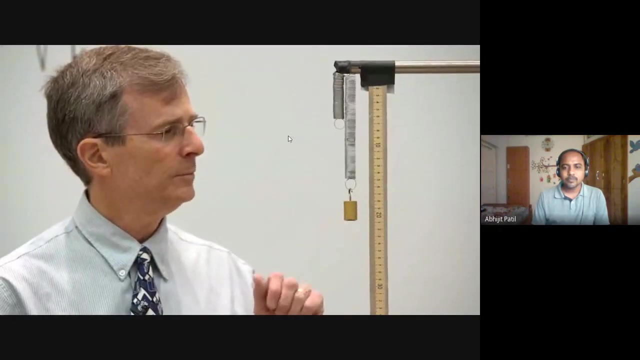 small amplitude: boom, boom, boom, boom, boom, boom. here's a medium amplitude: boom, boom, boom, boom, boom. and here's a large one: boom, boom, boom, boom, boom. and back to the small one again, and we're just getting a rough measurement here: boom, boom, boom. I think you can tell the the amplitude or that the period doesn't. 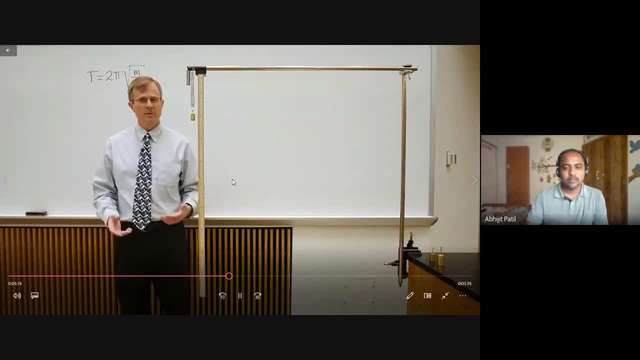 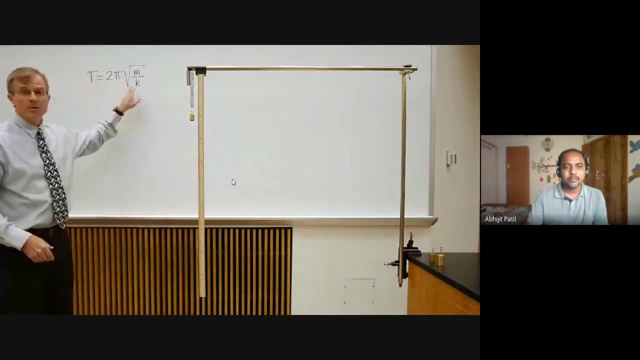 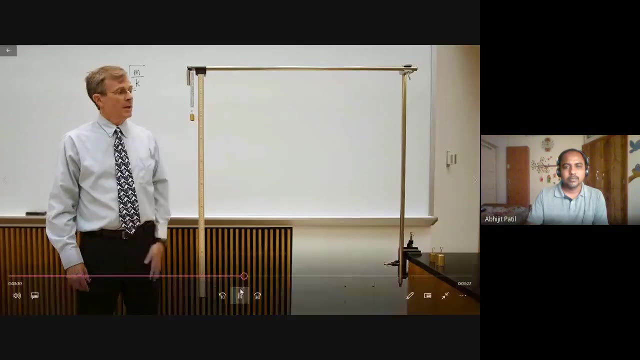 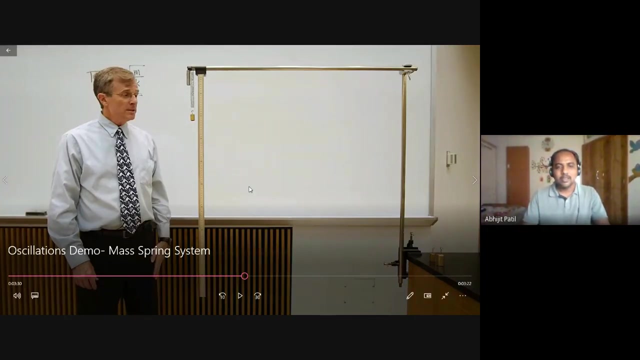 seem to be depending much, if at all, on the amplitude, and in fact the mathematics bears this out. the period T has no dependence on the amplitude of the motion, but it okay. so that is the thing. the amplitude of the motion. that means how you start the vibration. the time period will not depend on that. yes, if you start with one. 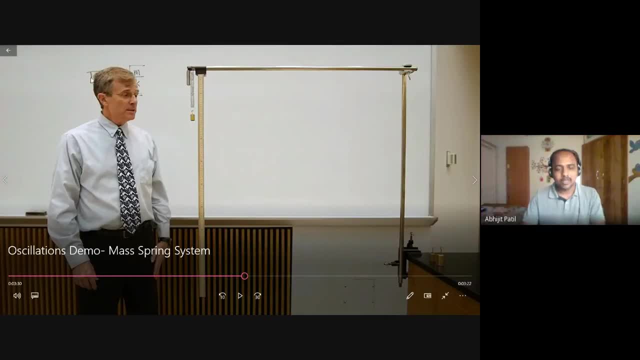 centimeter, same time period required to complete one cycle. if you start with larger, like 10 centimeter, amplitude again, the time period required will be same. does depend on the mass. so let's look at. so. in this formula you have mass included, so he will now replace this mass with. 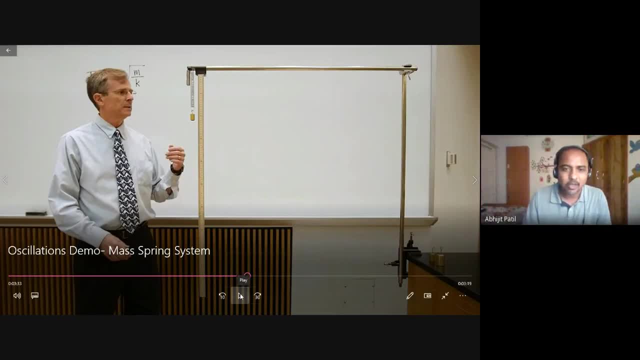 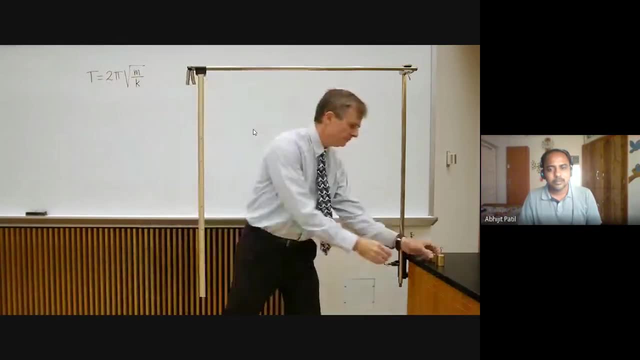 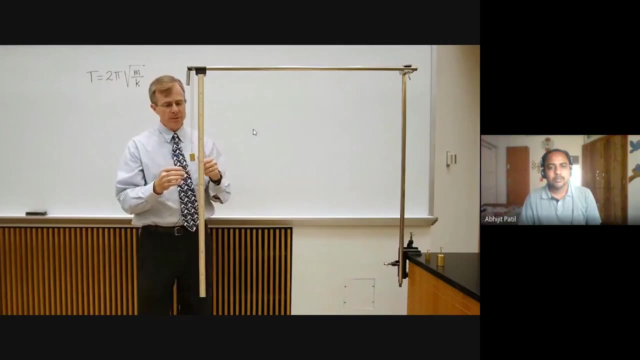 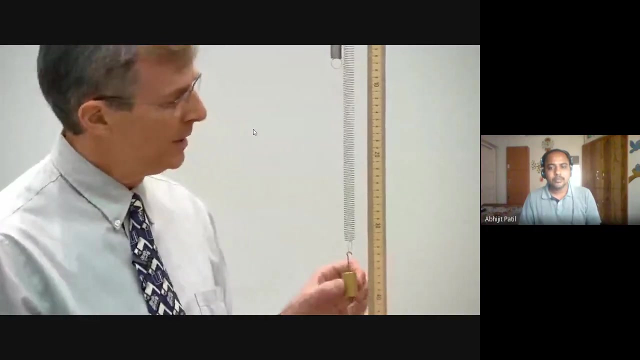 pi, pi. it must, and we'll see how. what happens at the period is a function of the mass. by adding a bigger mass, remember how fast the last one is going. first thing to notice is that our equilibrium position is no longer at 19 centimeters, it's down at around 36 centimeters, and then, if I give it some, 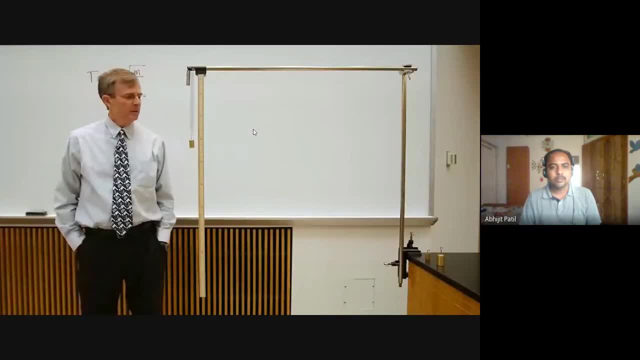 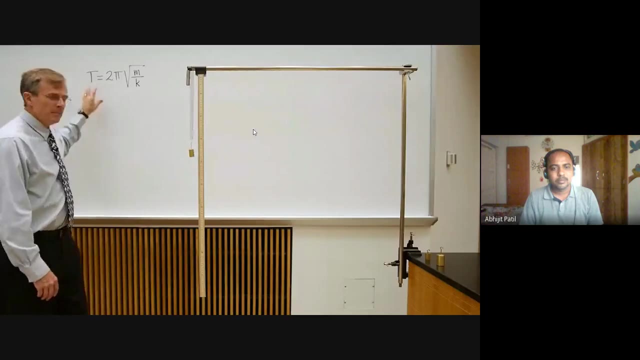 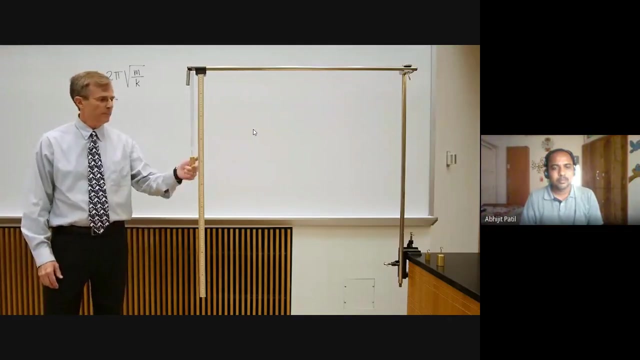 motion and look at the period. the period is now boom, boom, boom, boom, boom. it's slower, takes longer. so that means the period is the time between uh, a time for one complete oscillation. so that's from here back down to here again. that time is now longer, with a bigger mass, exactly as predicted by the 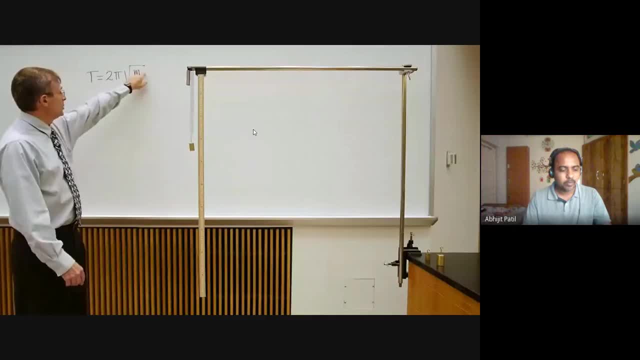 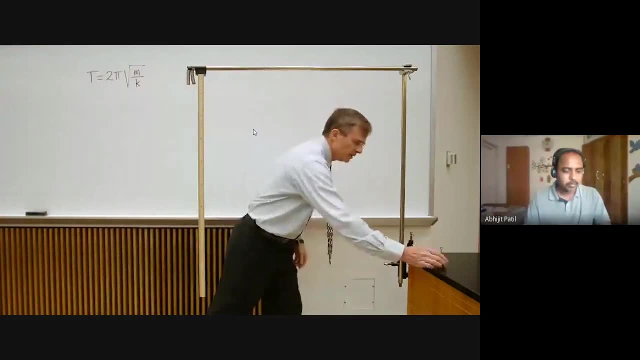 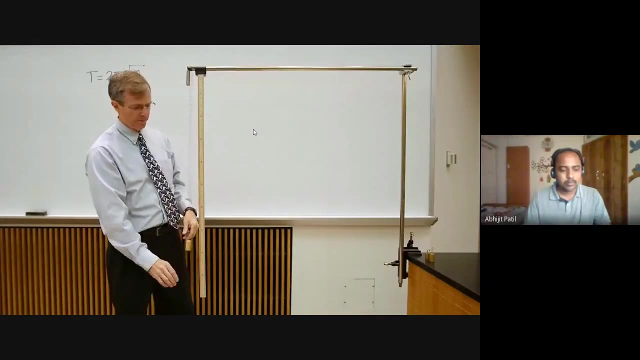 equation: if you increase the mass, it's in the numerator here- that will increase the period or the time for one complete oscillation. and then bringing this to the extreme, even longer period equilibrium position: much lower: boom, boom, boom, boom. very, very long period motion. so how does this depend on the spring? 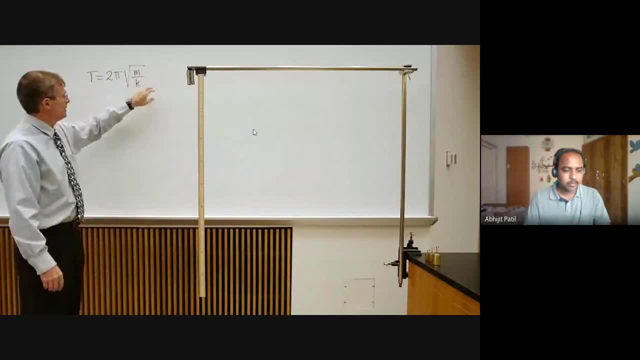 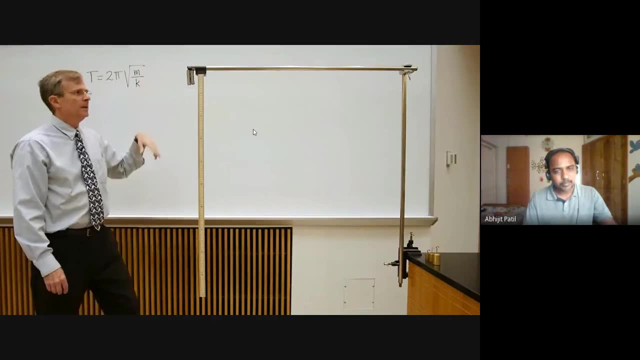 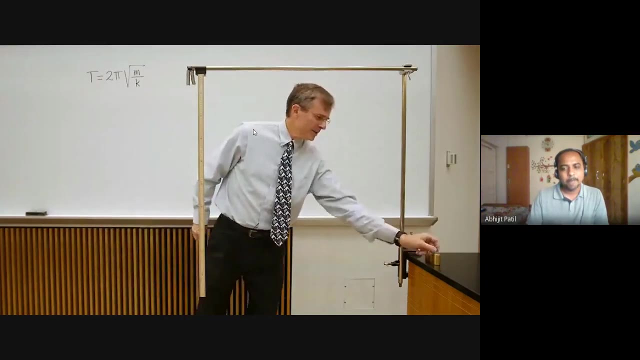 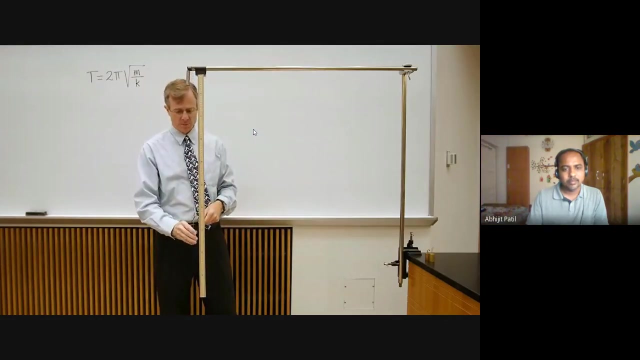 constant k get the dependence on the mass down. the period depends on one over the square root of the spring constant. if i use two springs instead of one, i thereby doubled the spring constant. so let's compare the period with just one, one spring and this large mass boom. 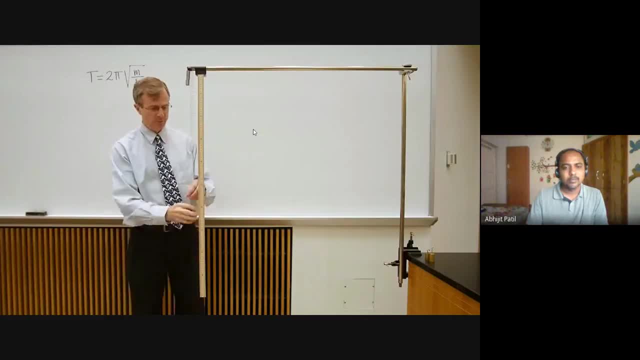 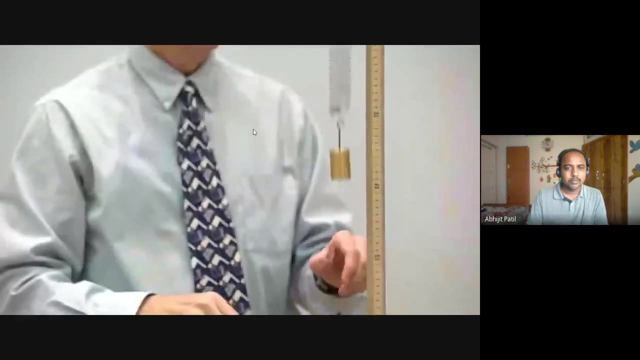 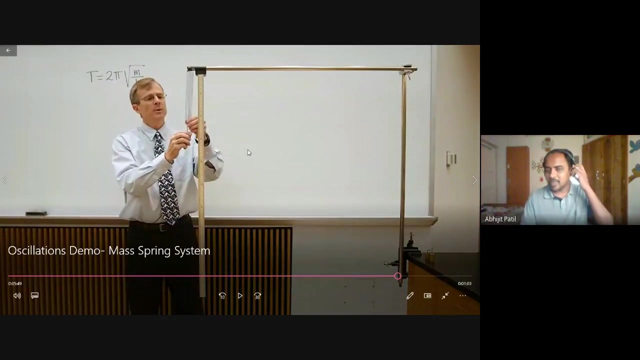 boom, boom, boom and the same mass with two springs. you know, first, that the equilibrium position is higher because we got more force pulling it up to counteract gravity. boom, boom, boom. a little bit faster, faster, okay. so, uh, the takeaway from this video, the time period, if you see the as he was. 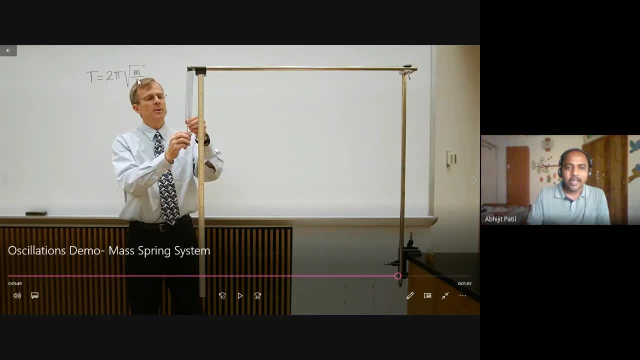 increasing the mass, the time period was increasing and as he increased the stiffness which represent, which is represented by these springs. so, instead of one spring, when you attach two springs, that means the stiffness is increased, the time period decreased. so this is the mathematical equation and this is how practically we can see the actual things happening. okay, now we will see. 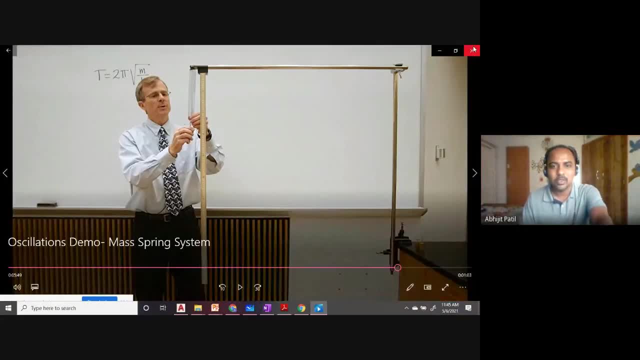 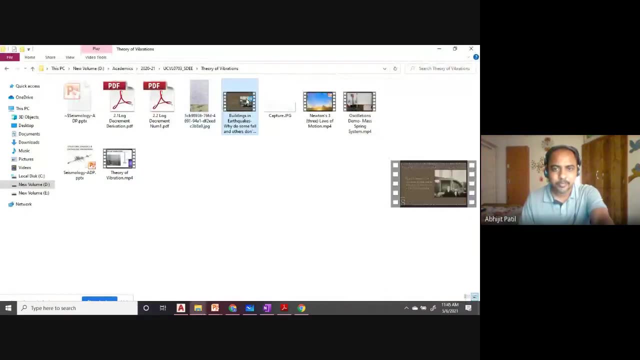 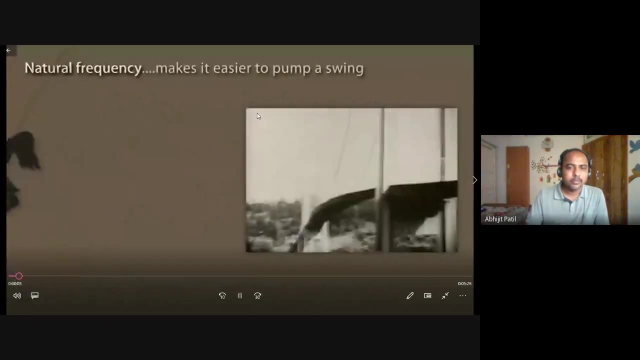 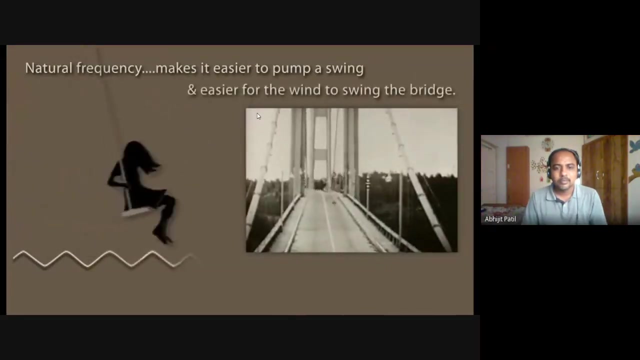 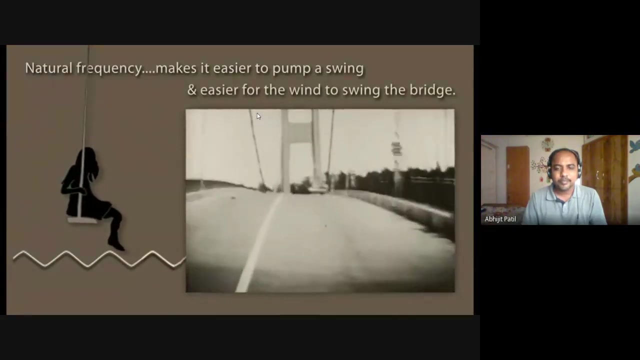 another video to understand what is the relation of this video or this time period- mass and spring- with our structure. to understand the resonance of buildings during earthquakes. we will look at other resonances. the natural frequency of a swing makes it easy to maintain the motion using little energy. a prolonged wind swung the bridge on the right at its natural frequency. 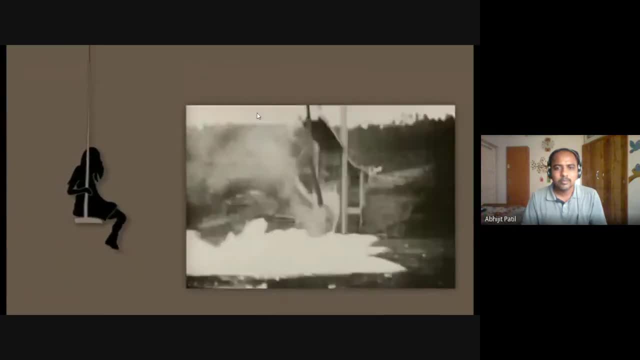 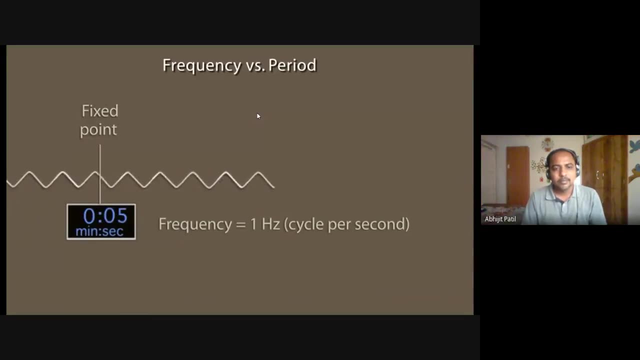 until it exceeded its structural integrity and tore apart. the frequency of a wave refers to the number of waves that pass through a point from one second. a period is the amount of time that it takes one wave cycle to pass the given point. a frequency of one cycle per second has a one second period if the frequency doubles to two cycles per second. 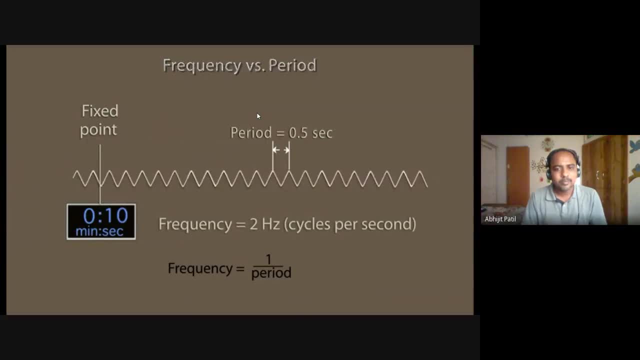 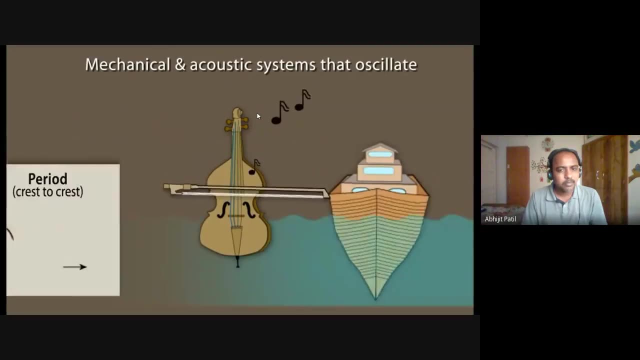 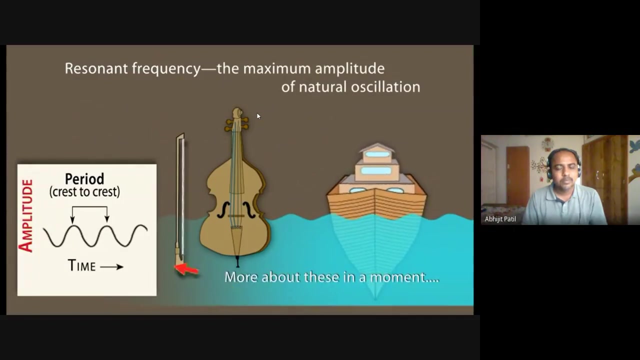 the period is only half of a second. resonance is a tendency of a system to oscillate with greater amplitude at some frequencies than at others. the resonant frequency of any given system is the frequency at which the maximum amplitude oscillation occurs. for example, the resonant 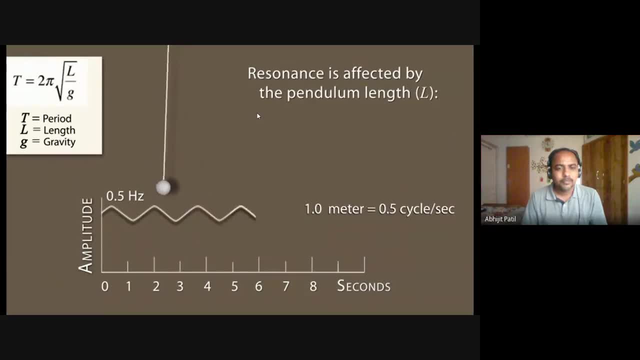 frequency of the one meter long pendulum is one half of a hertz. if the string were one quarter of the length, it would vibrate at twice the frequency. small amplitudes can be approximated by this equation using length in the gravity constant. in Resonant systems can be used to generate vibrations of a specific frequency to create 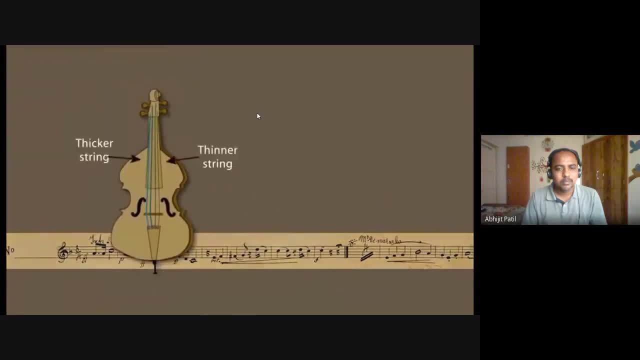 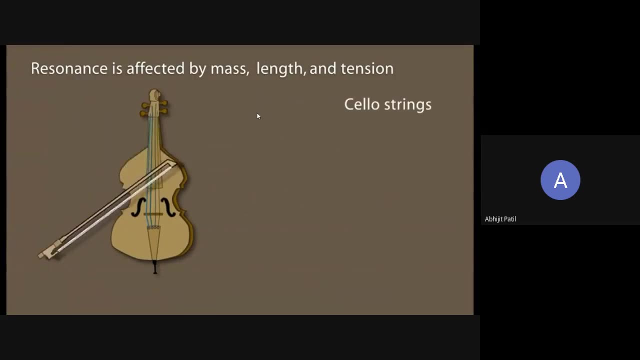 music Strings under tension, such as with this cello, have resonant frequencies directly related to the material of the string as well as the mass, length and tension of the string. The mass of the slow C string resonates at 264 hertz, whereas the thinner A string of a different. 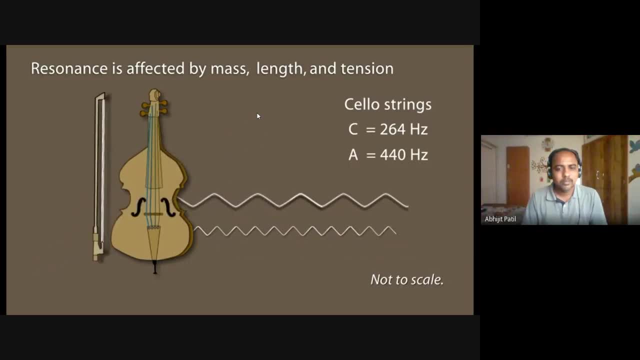 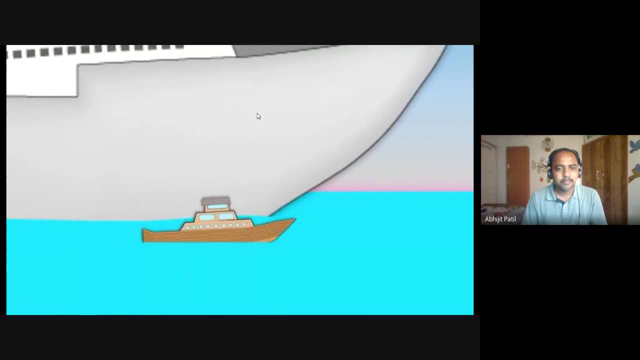 material resonates at 440 hertz. Now we use a simplified analogy of boats at sea. A series of waves, particularly when they hit broadside, can initiate rolling behavior. The smaller boat is affected by short-period low-amplitude waves that slap against the ocean. 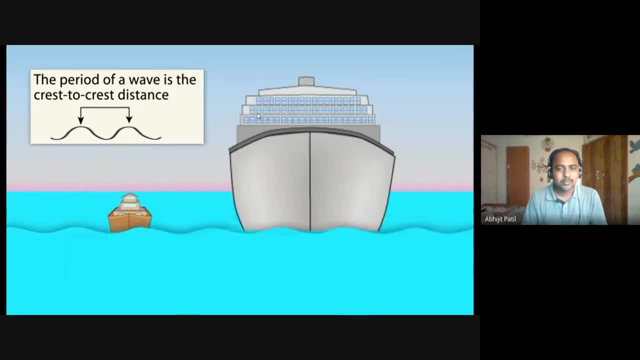 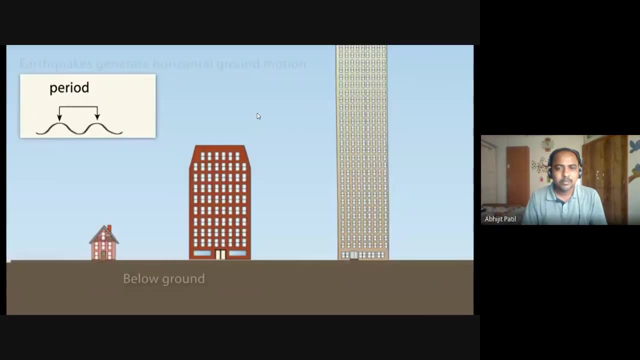 liner with no effect. Small boats, on the other hand, will ride up and over long-period high-amplitude waves As a larger boat begin a long slow rock. Now let's look at how buildings are affected by earthquake-induced seismic waves. All buildings have a natural period, a resonance, which is a. 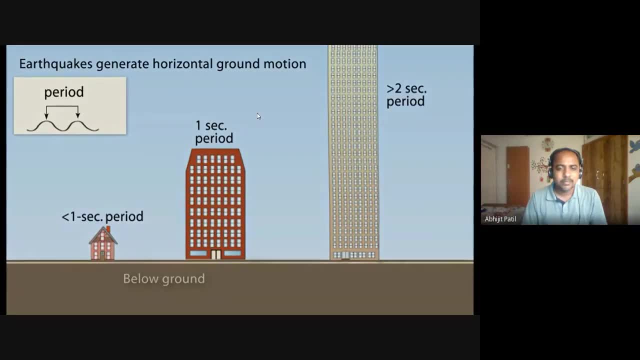 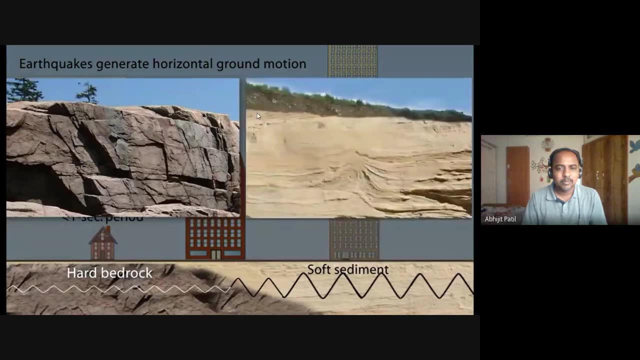 number of seconds it takes for the building to naturally vibrate back and forth. The ground also has specific resonant frequency. Hard bedrock has higher frequencies than softer sediments. If the period of ground motion matches a natural resonance of a building, it will undergo the 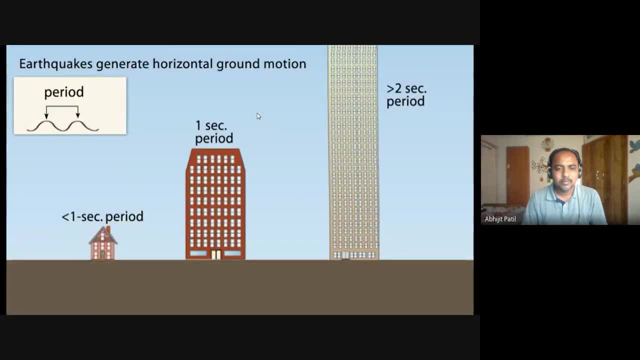 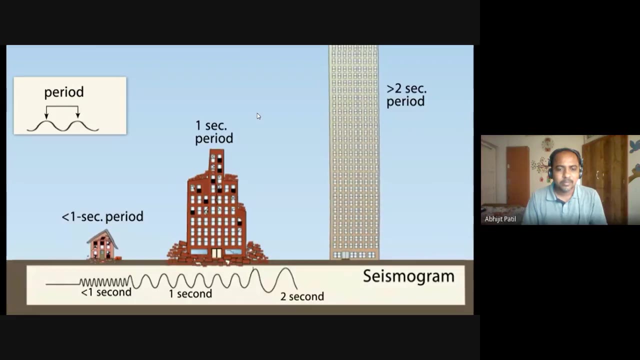 largest oscillations possible and suffer the greatest damage. Small buildings of one or two stories resonate naturally at much less than one-second periods. One-second period will affect buildings about 10 stories. For example, a 30-story building resonates at a period of three. 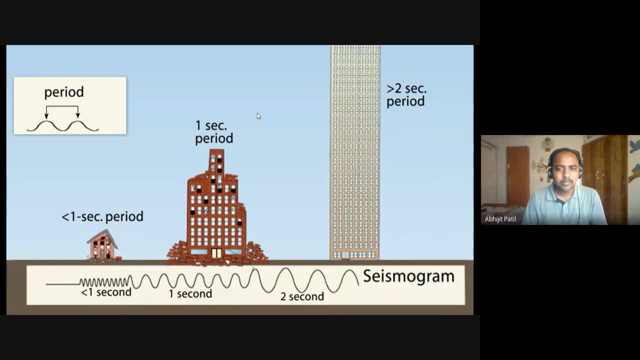 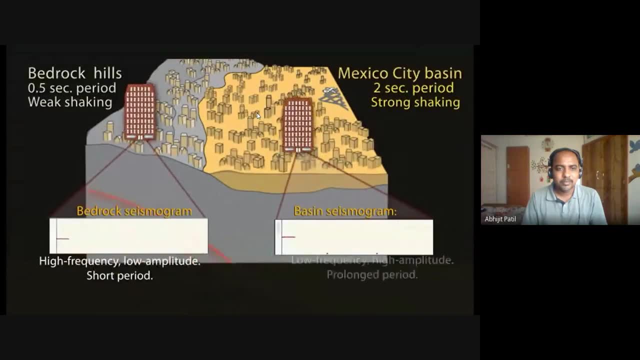 seconds and a 50-story building resonates at a period of five seconds. During the 1985 Mexico City earthquake, the ground beneath the city resonated with a two-second period for over a minute. Thus medium-height buildings with similar natural periods. 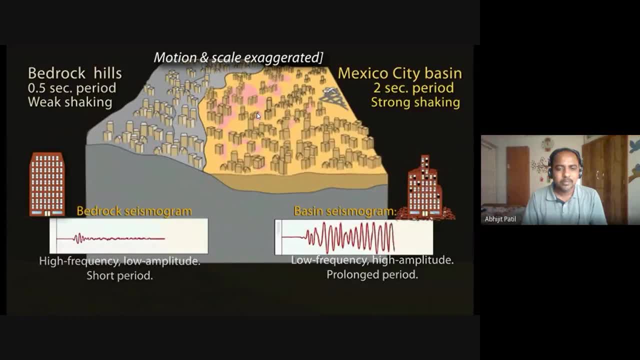 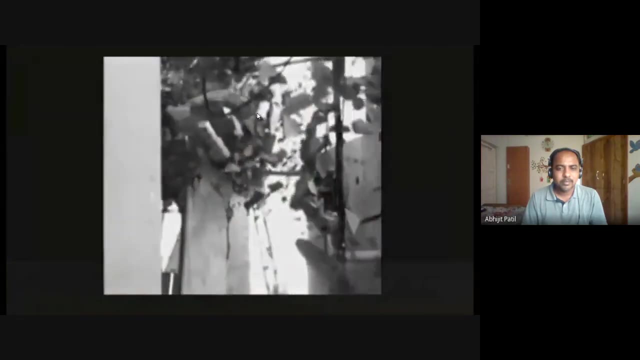 suffered the most damage, while short, old, weak stone buildings and skyscrapers were relatively undamaged. That proved to be what is called a resonance disaster, which is how engineers describe the destruction of a building by seismic vibrations at a system's resonant frequency. It is because of prolonged energy input that the system swings more, and 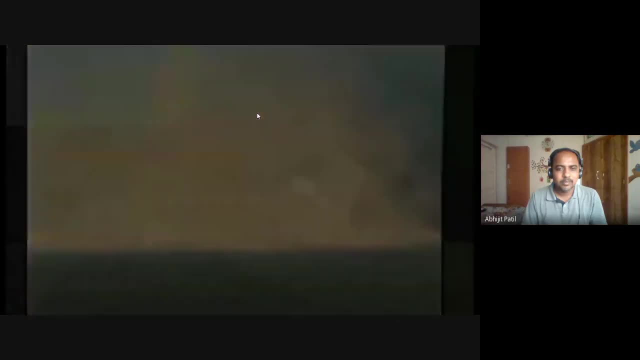 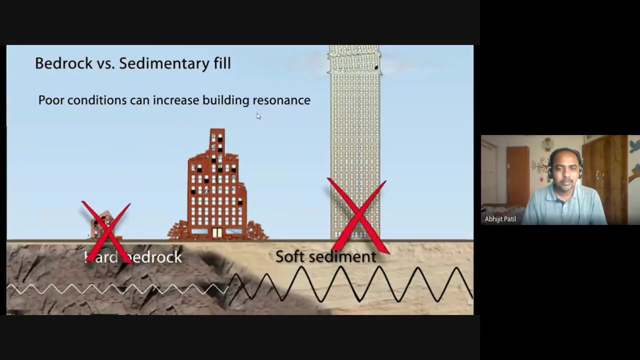 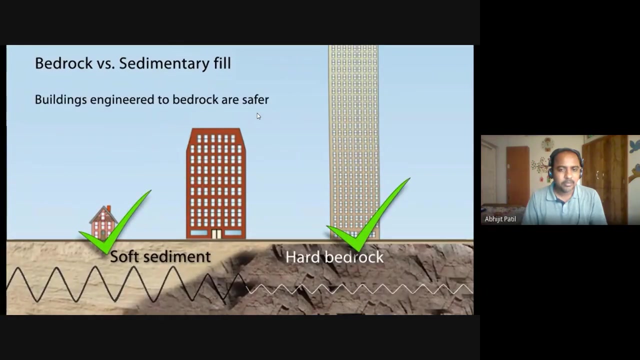 more strongly until a structural load limit is exceeded. A key point here is that the small buildings on hard rock and large buildings on soft sediments may suffer more damage and ground motion effects from an earthquake than small buildings on soft sediments and large buildings on hard rock. Resonance is one factor that contributes to earthquake damage Of. 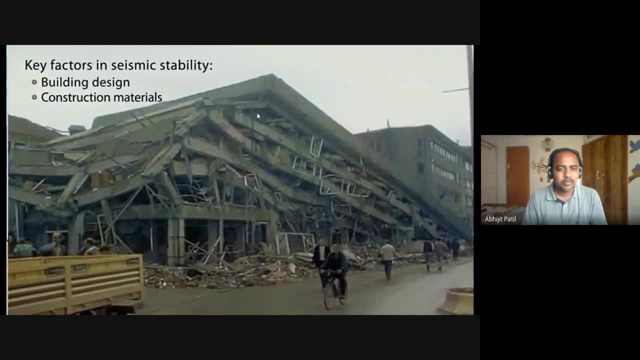 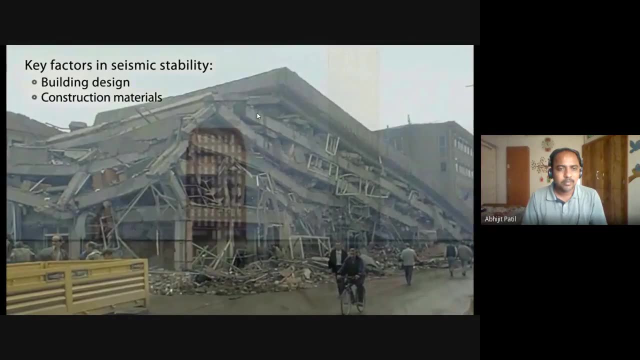 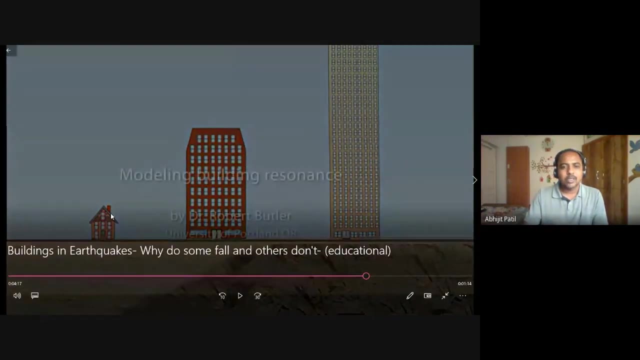 equal or greater importance are building design and the quality of construction materials. By determining the resonant frequency of the ground beneath the building site, the building design can be modified so that a resonance disaster does not occur. The following demonstration is just an example of how a building can vibrate and have their own. 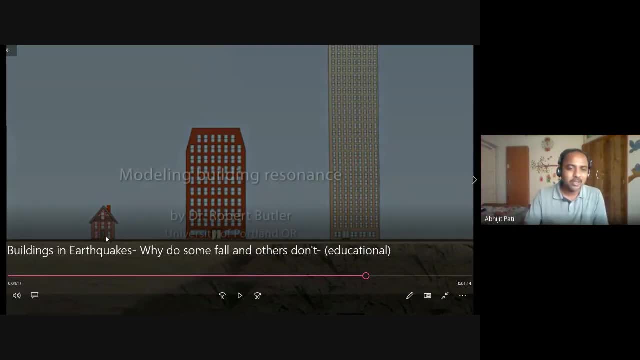 time period, because the time period depends on mass and stiffness. So stiffness is here. I will, after this video, I will just shortly explain how the stiffnesses are derived. So a particular building has a particular time period and when the earthquake waves pass. 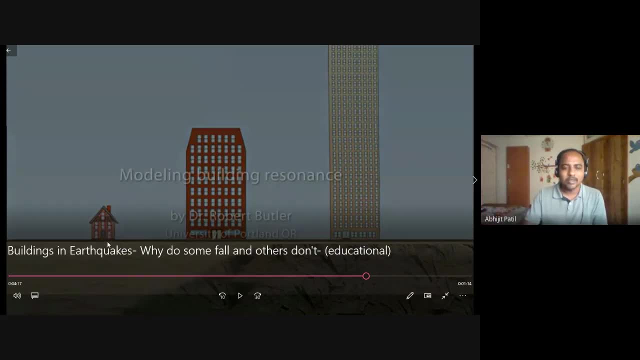 if that matches with the time period of the building, the chances of damage are more So the small building, medium building and large buildings. So if this time period generally in soft soil is longer and the time period on the bedrock or hard rock is shorter. So what is suggested here is this time period of small building is 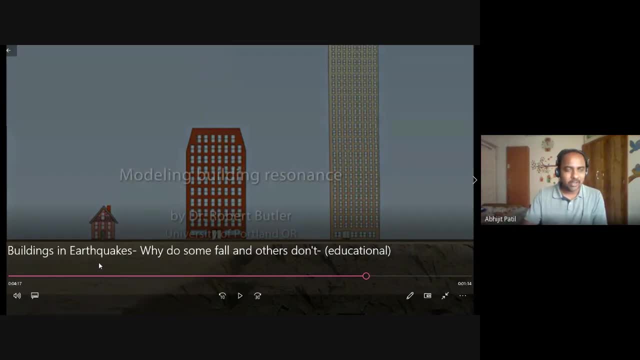 smaller, So this can be registered on soft soil and the tall buildings can be rested on bedrock. But so this is a theoretical suggestion. but practically you live nearby Mumbai. So if you have visited the South Mumbai and we already know that whole the Mumbai, 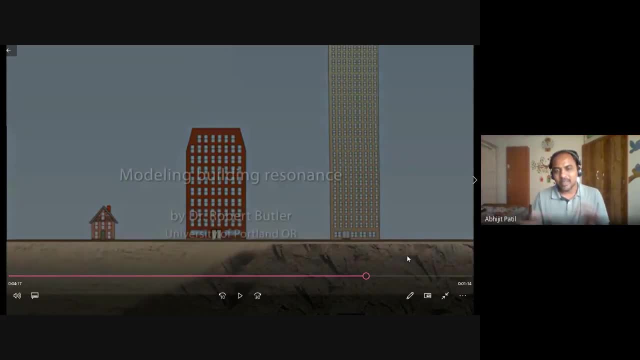 it was actually seven, I guess I'm not wrong, seven islands, and then they were connected together by pouring soil. So basically, all the tall structures in India, most of the tall structures in india, are in mumbai and it is resting on soft soil. so how that is happening. so if you see that, 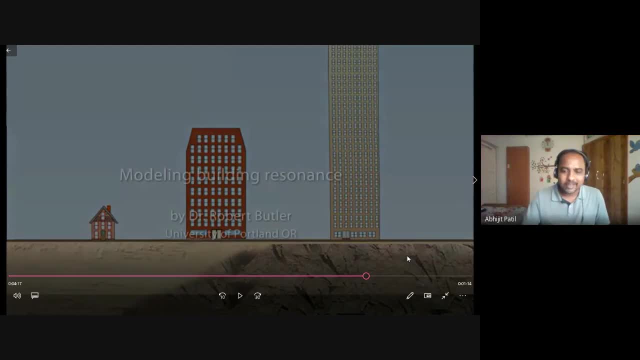 it is not resting directly on soft soil. they drive piles. okay, until the hard strata is available, and on that hard strata these buildings are rest. so that is why these buildings can survive the earthquakes. okay, so these technological solutions need to be done by civil engineers or structural engineers. okay, so generally, this is happening. so 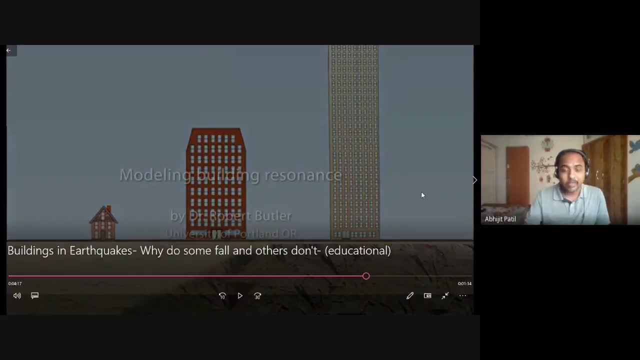 even if you see the bush earthquake, so this basin effect which was shown here. so same thing. that example was for mexico, but same thing was happened in case of bush earthquake. so the earthquake location which is called as focus, so that was nearby, or epicenter, that was nearby the 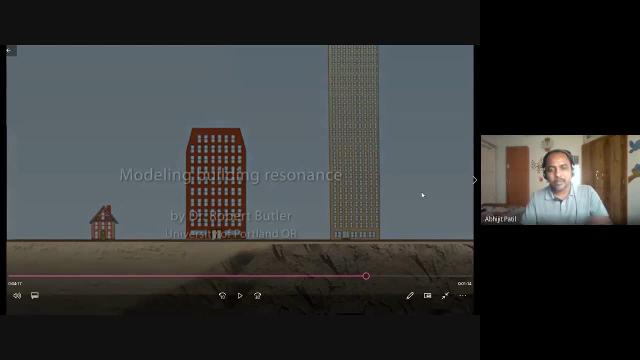 uh, bush, okay, but amdabad, i don't remember why- i think 200 plus kilometers away from the. so the damages near bush were less, but the damages in damages to buildings in amdabad was devastating. okay, two reasons. one: nearby there were small buildings and in the hard it was. 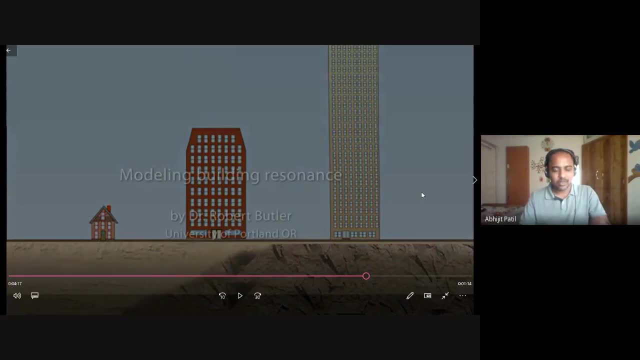 not on very soft soil, it was a medium soil. the amdabad is located in the basin of river and it is basically soft soil and there were buildings of five to seven storage located and that the time period of vibrations was more in the amdabad and that matched with the 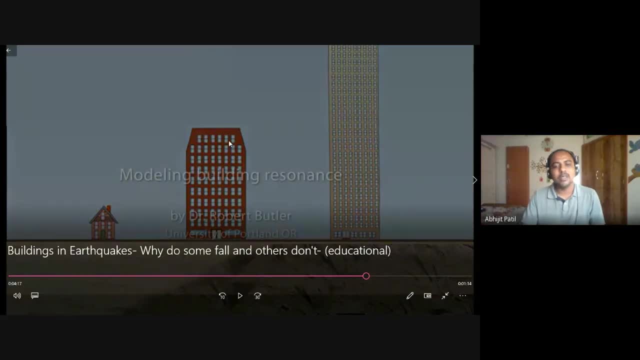 medium height buildings and because of that, the damages were amplified in amdabad. okay, so that is another takeaway from this video, another demo just like this. this is we have seen in animation, so one professor. that video is also very famous and it is available on youtube. so that will be. 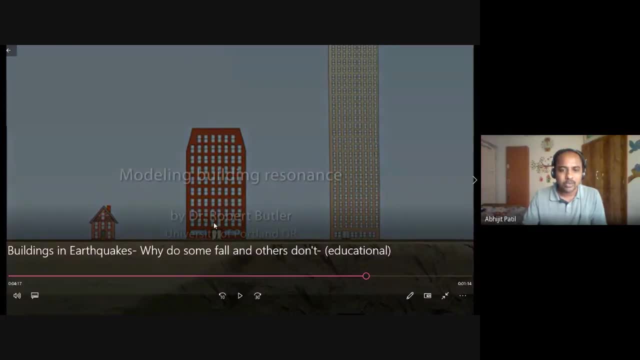 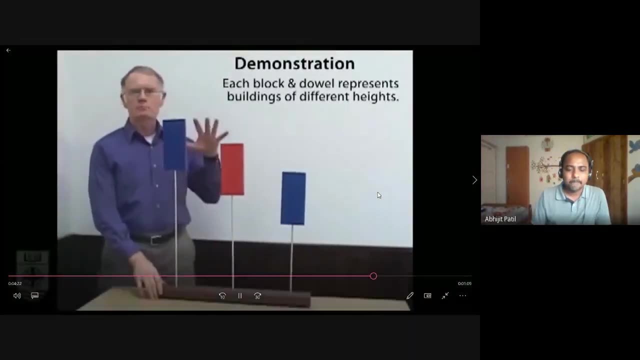 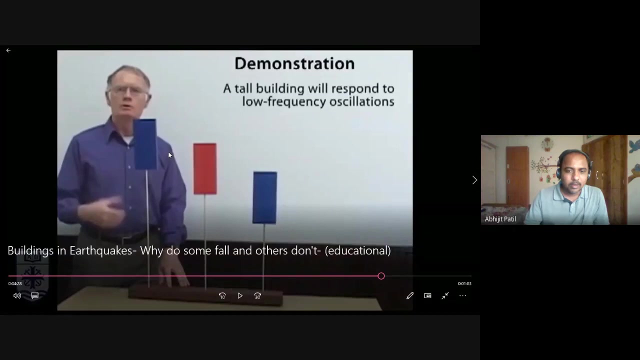 followed. so modeling building resonance by dr robert butler, that are model resonance in the classroom. the idea of the boss model is that different height buildings will respond to different frequencies of horizontal ground motion. so the building is a tall building, okay, so, uh, before we proceed, so this is represented, uh. 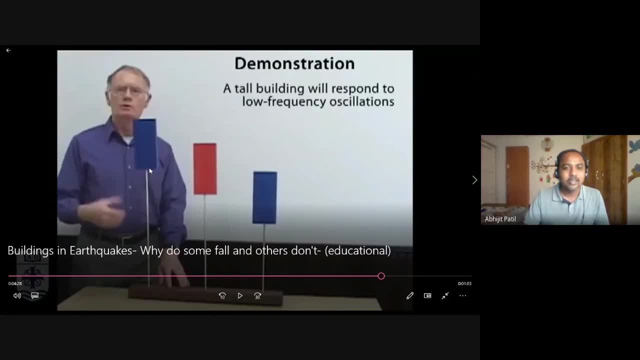 representing the mass of the building. okay, and this string is representing the stiffness of the building. so stiffness is resistance to force, and that is nothing but our columns. okay, so every building is resting on columns, so those columns can be modeled as a single line representing the same stiffness. okay, so this is a tall building. 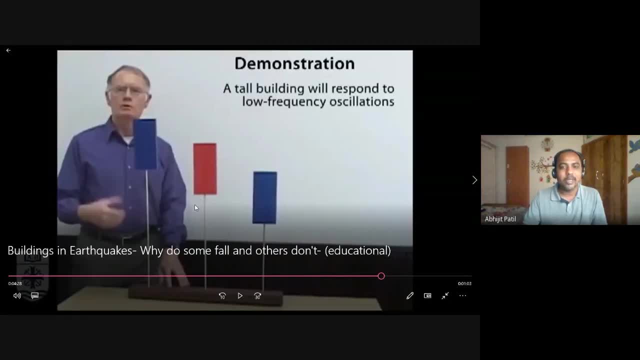 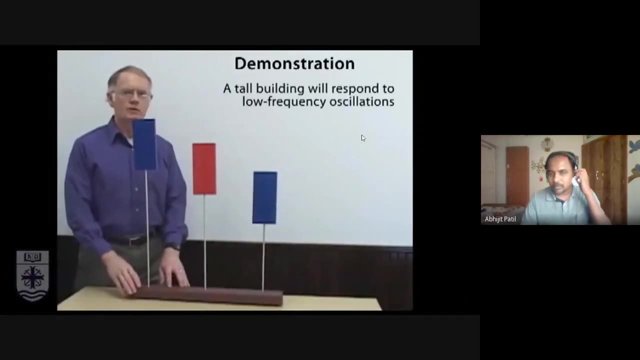 this is a short, medium height building and this is a short building. now what he will do? he will just uh, try to vibrate this with different frequencies and see which uh building will respond. more building will respond to very slow or low frequency oscillations of the ground. so if i move, 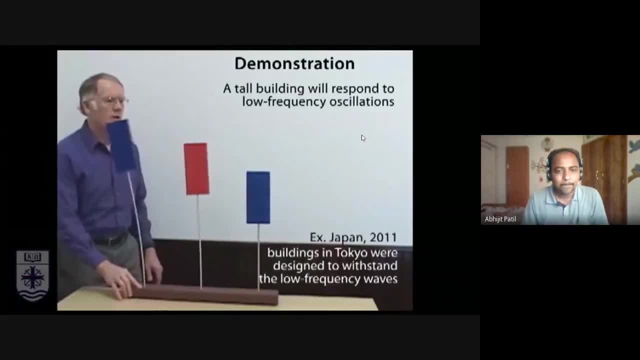 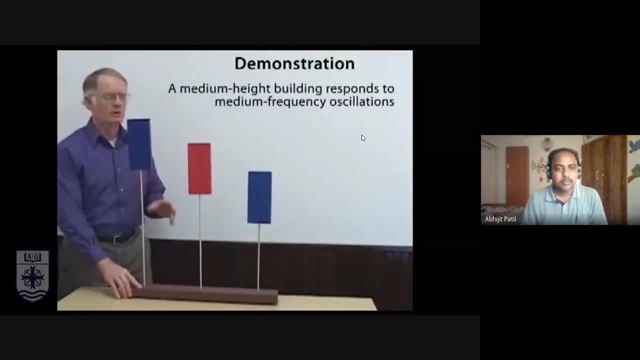 the base slowly back and forth, i can get the tall building to oscillate, where the intermediate and short building will respond to the oscillation of the ground and the short buildings are not moving. if i move it more briskly, i can dial in the rate of horizontal oscillation so that i move the center building, the 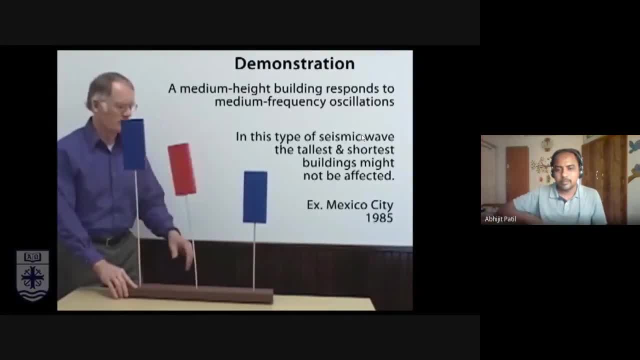 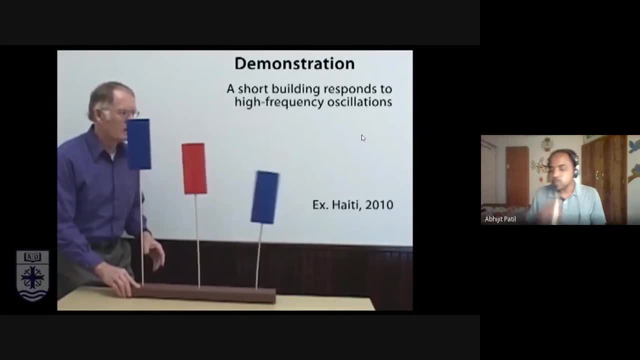 intermediate height building and the short and the tall ones are barely moving. to get the short building to oscillate you need to move the base very briskly back and forth and dial in to the natural frequency of the short building and we can see that the intermediate and 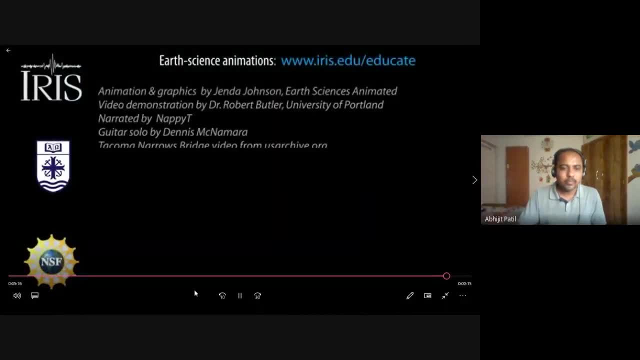 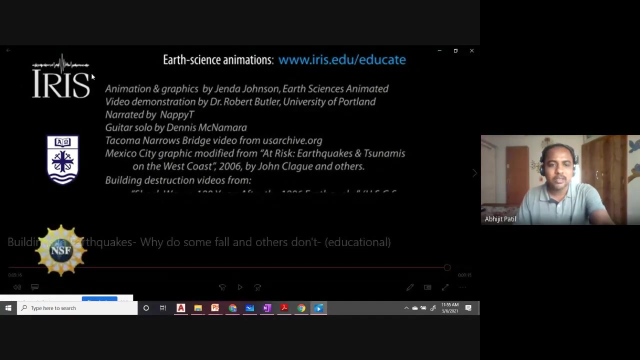 short buildings are fairly moving. okay, so these videos are available. if you are more interested on this website, iria, so this is one institute which keeps on researching on earthquakes, so a lot of videos are available there so you can go through that if you are curious. okay, so this is what we have seen, that the buildings. 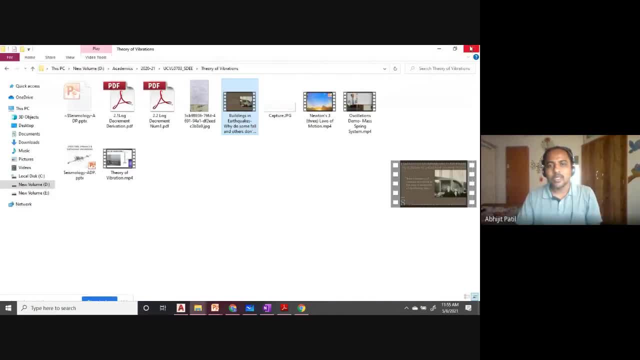 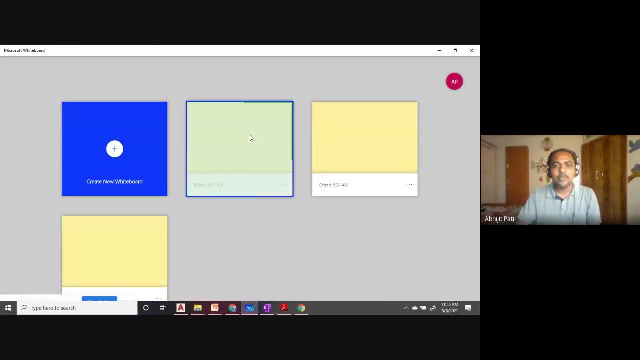 are having their own time period. okay, and depending upon the uh time period of the building, the building will response to earthquake. so basically, as i was mentioning, we just try to get so any tall building or uh single solid. also, any building plane can actually be represented, so it has its internal design. 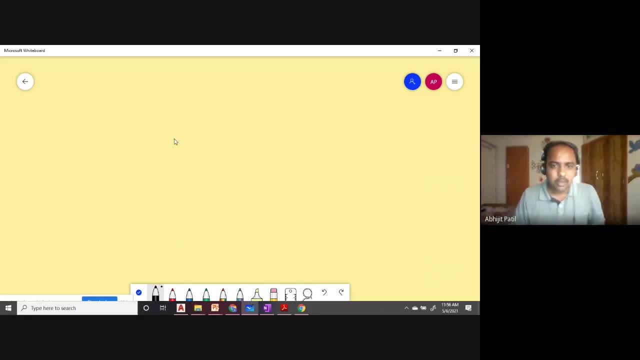 so let's see which block primarily line level project it is, but this one is point function. so what do you do? this is the position of the height of that wonders w. i'm sorry for defeating you. sorry, i'll change the color of the pain. and this is nothing but floor level. so this represents the mass of slabs and beams. okay, as. 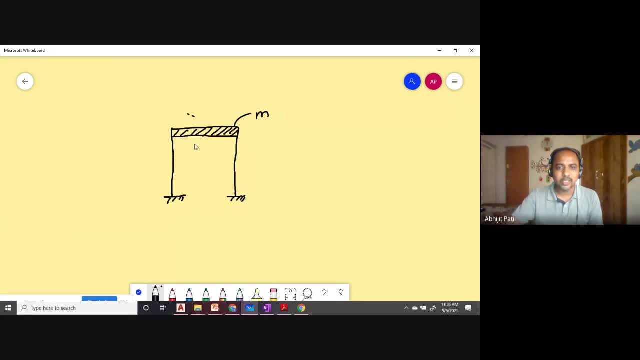 well as walls. so whatever load of wall is there that is included here, and 50 percent of column weight is also considered to be acting at this floor level. okay, so we are assuming that there are some whatever mass is there that is concentrated at this slab level. okay, these two indicate: 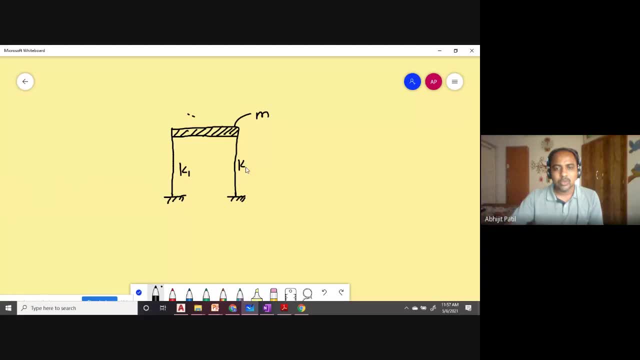 columns with stiffnesses k1 and k2. so what is stiffness? it is resistance to force. so if you just go by this equation, force is equal to stiffness into deformation, right? so so, mathematically, if you see, i think i am telling you something wrong. just let me. 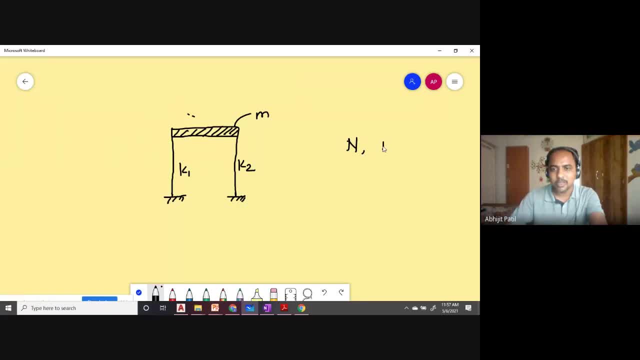 so the unit of the force is newton, the unit of the displacement is meter and the unit of this is s. i was right. in perm versions X actually stiffness is defined as force required to displace any task, in this case the portal frame, by a unit displacement. 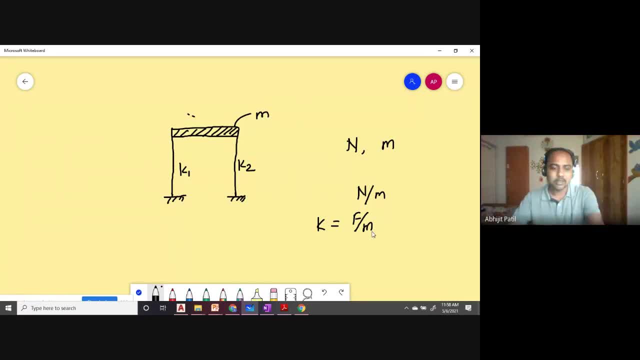 sorry or okay. so force required to displace any takes any structure by one unit. so if we have six, four, let's have six, two, three stitr stretch. oh, five, three, one, six. it is a newton per meter, so suppose one newton per meter is the stiffness that means this structure. 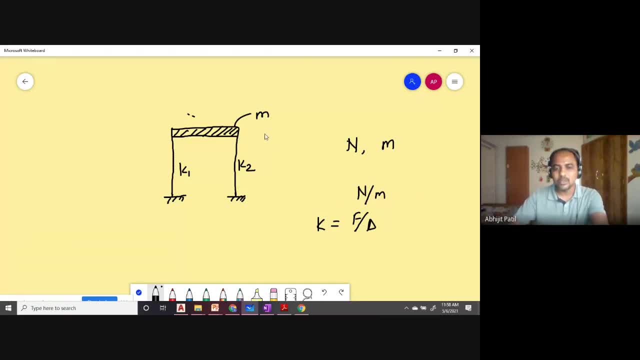 is required to apply one newton force to displace this by one meter, like that. okay, so this is the basic uh idea of stiffness and this stiffness is, uh, suppose a cantilever column is there, okay, for lateral deflection. so, uh, if you remember, this is calculated: the deformation here. 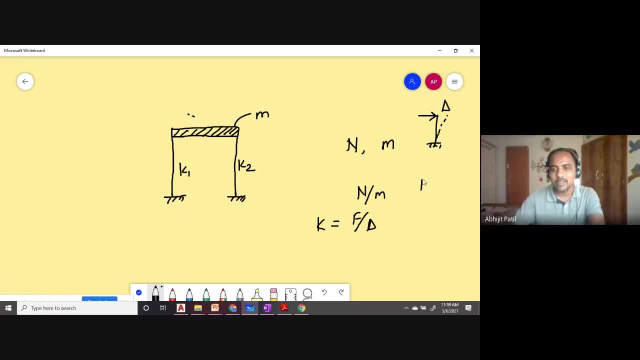 will be like this. so this delta is calculated as if this is the force: p, p, e, i. e is the modulus of elasticity, i is the moment of inertia. 12 l cube l is the length of the cantilever. so if you remember this from structural mechanics, 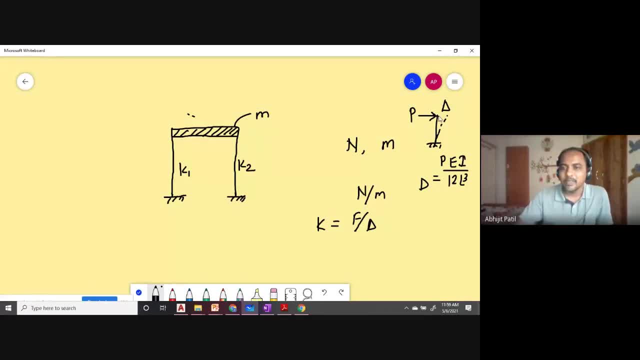 the displacement of a cantilever beam or column, whatever you say, of length, l, modulus of elasticity, e, which will depend on the material, and this i will depend on the cross section, whether it is circular, rectangular orientation, etc. so p? e i by 12 l cube, and if i just 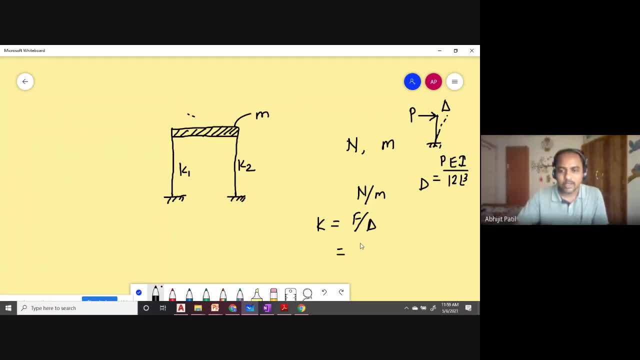 want the stiffness of this column, so what i will here. f is equal to p, in this case divided by p e i upon 12 l cube. so if we just simplify this, it will become 12 e i by l cube. so this is the stiffness of a typical column. okay, so how to calculate stiffness? 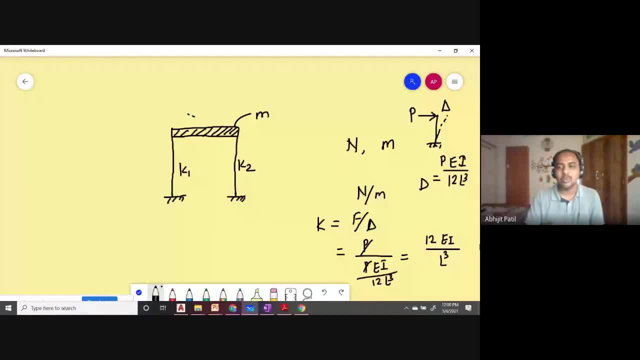 simply, You can refer to any structural analysis book. So there you will find these standard deformation formulas, Or the stiffness is also given. But how is that calculated? So this is how it is calculated: Force required per unit displacement is nothing but stiffness. 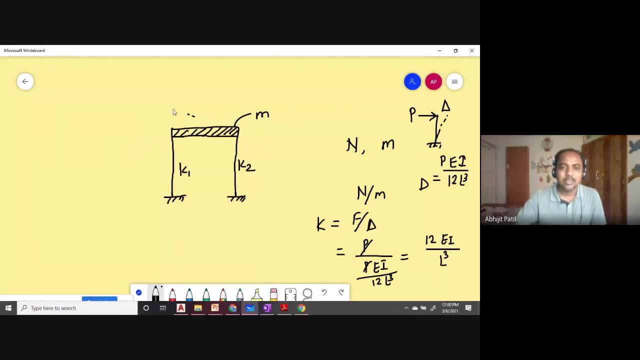 So, coming back to this, our buildings can represent as like this: Suppose, this is multi-storeyed, two-storeyed. You can assume it like this: So this is one-storey, M1.. This is another storey, M2.. 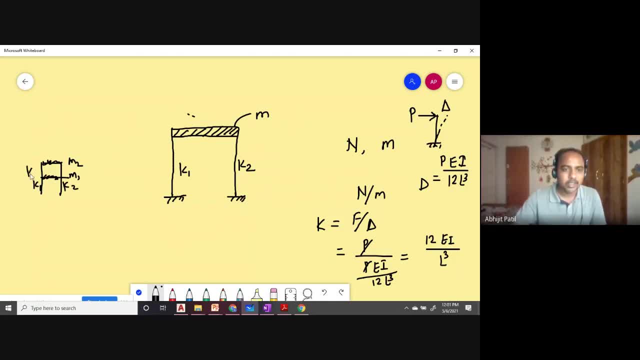 This is K1, K2.. Again here, it is K3, K4, like that. So if 10-storeyed, again this thing will increase like that. So we'll focus on single-storeyed. We'll focus on single-storeyed building. 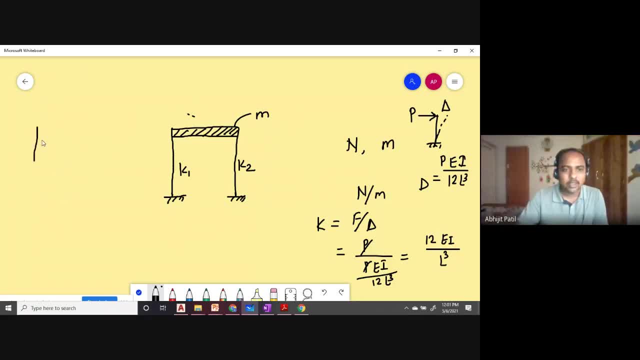 This can be represented with the help of a model called a spring model, spring and dashpot model. So I will just explain what is this: spring and dashpot? So this is representing K. So this is the combined stiffness of these columns. What is C? 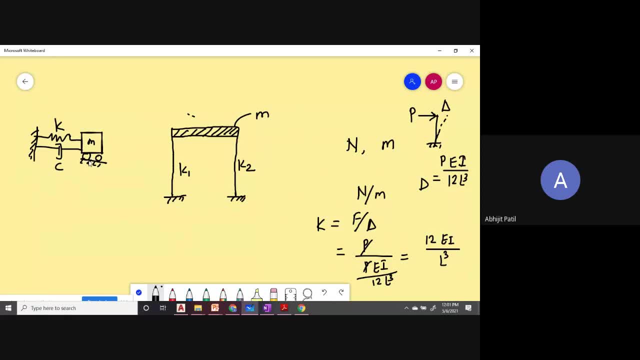 I will explain What is M. I will explain What are these rollers. So these rollers indicate that this is a mechanical model, If you see spring. So whatever we had seen in that demo video, in that, only this dashpot. this is called a dashpot. 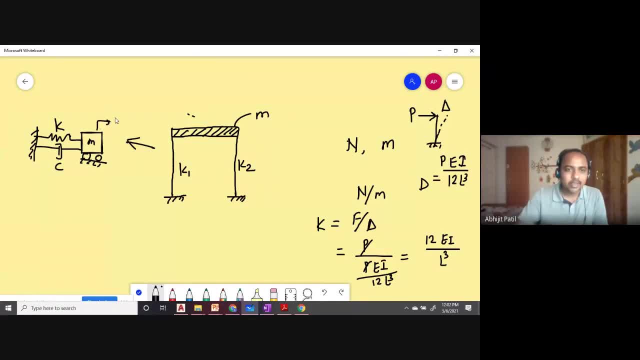 this is added And this is vibrating in this direction, So x, let us say, time-dependent. So if I just pull this mass and leave, it will start vibrating like this, Like this. So this model and this model are same. 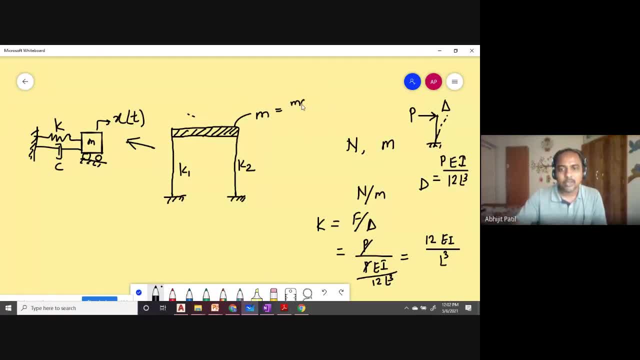 So here, mass is what Mass of M is what Mass of slab beams, et cetera, K1, K2, these are stiffness. From here, the stiffness will be offered by columns. okay, then, where? what is c? what is c? so this c is nothing but resistance. 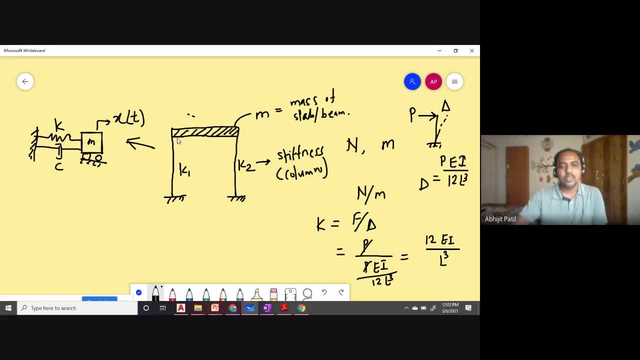 okay. so if you see, this is concrete. so whenever this is moving in this direction, what will happen? the concrete: we know it is not homogeneous material. it is made up of aggregates, coarse aggregates, fine aggregates, cements. so there will be internal friction between these materials and these materials. internal friction is represented by: 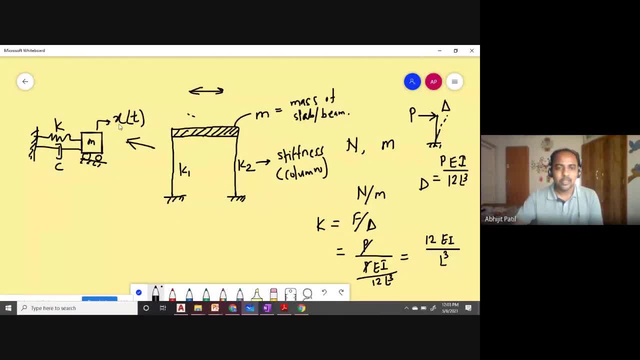 this c. okay, so this is the spring mass, that spot model. this can also be represented like this. so if i ignore this, this is negligible generally. so we can ignore this for time being. so this can be represented like this. so this is mass, this is stiffness, and whatever second video, or in the last of the video, what whatever we have seen. 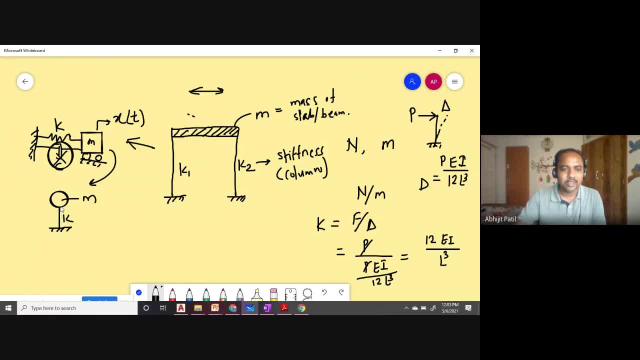 is this model. okay, so that vertical string is nothing but this stiffness of the columns and this mass attached above is the mass of the structure. okay, so this is how this is represented. and the equation of motion from newton's second law is like this: mx double dot plus kx. 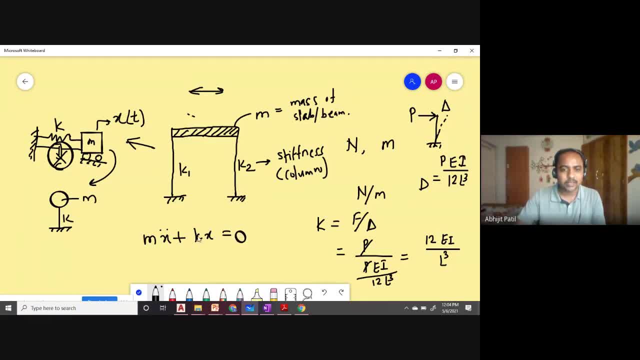 equal to zero. so k is here, stiffness, x is the displacement. x double dot is nothing but acceleration rate of change of velocity. okay, so just it is just for information. it is not included in your syllabus, but this is how our building is related to that mass and stiffness model. 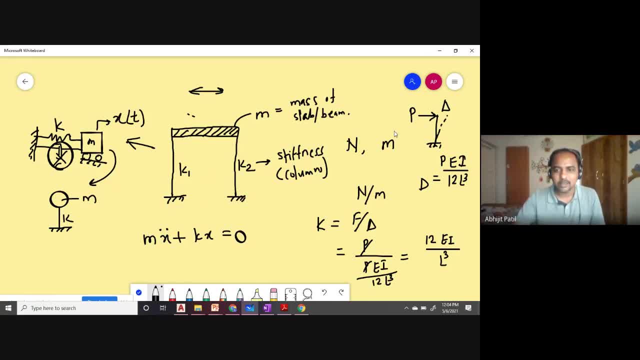 okay, so just try to remember this. so i hope uh, something is uh clear related to dynamics. so this is just a start of dynamic or very basic thing of dynamics. so from this mass and stiffness we can calculate the time period of the building. two pi square root of m by k. 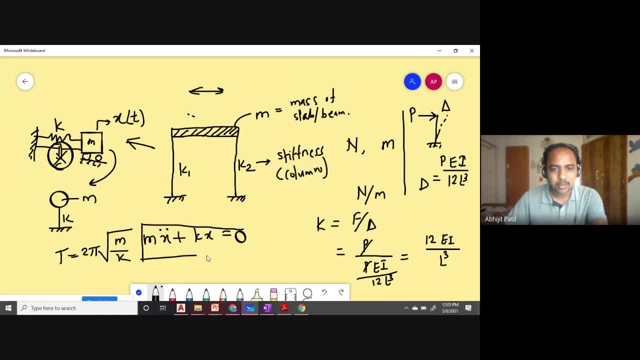 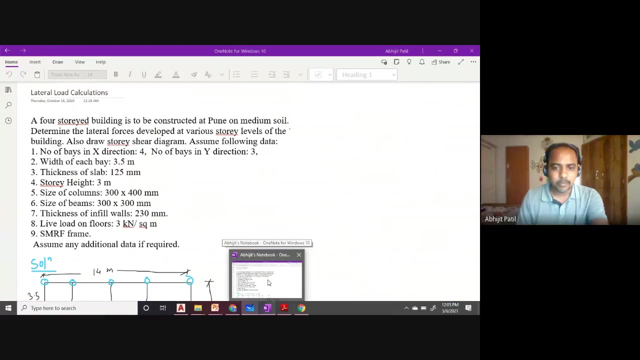 this is time period and this is called as equation of motion. okay, so from this equation of motion actually we get- i will not go into that derivation- so from this equation of motion we get this time period, uh expression. okay, so coming back to more information'll help you, so okay, 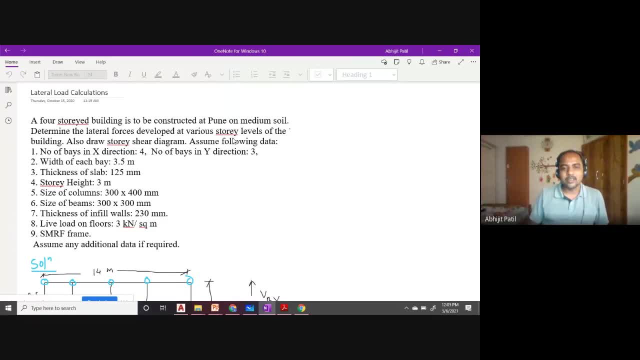 so this because fo across u, due to this, moving to menyur to these now. so, uh, the three step, thiscil one here that, according to the, that all right, or all right in your mind, you can't do it, that's it. you cannot go, so you have. 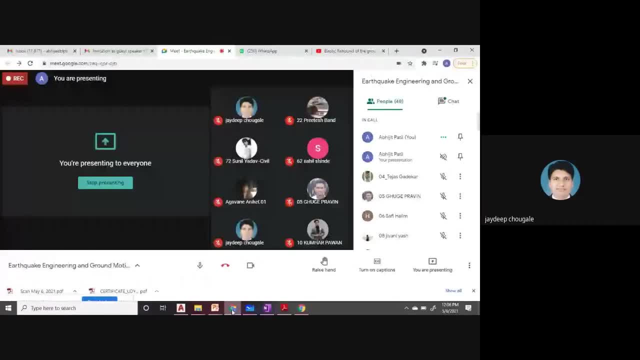 Yes, sir, The student. what do you do? Can you continue for one hour, or you can wait for tomorrow. Sir, continue, OK, OK, we will continue. I will continue for some period. I will just explain the basics of 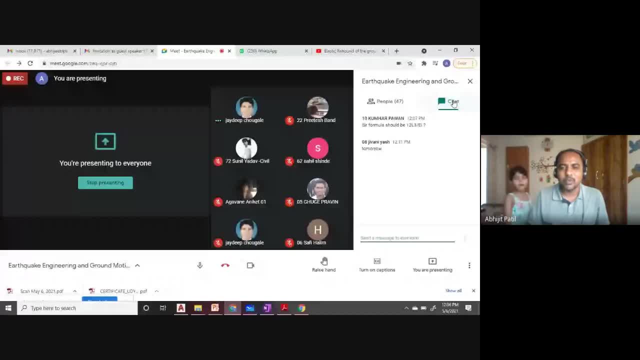 or I will just explain the numerical and actual solution. We will start tomorrow because it will be obviously hectic to digest so many new things. OK, Pawan is Pawan there. He had some doubt in the chat box. Yes, sir. 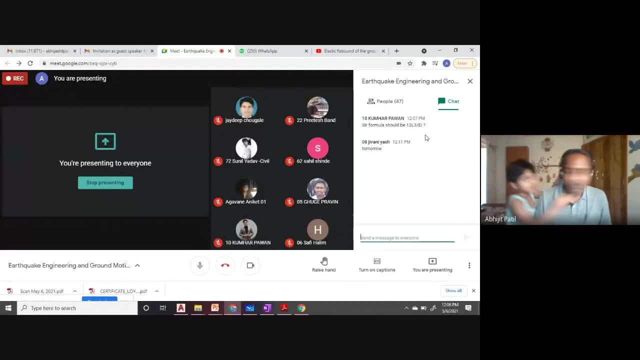 OK, Pawan. Pawan, are you there? Yes sir, I'm there. Yes sir, Is your doubt clear or you were saying something about formula? Sir, you have written the formula for K. that Well, EI by L cube. 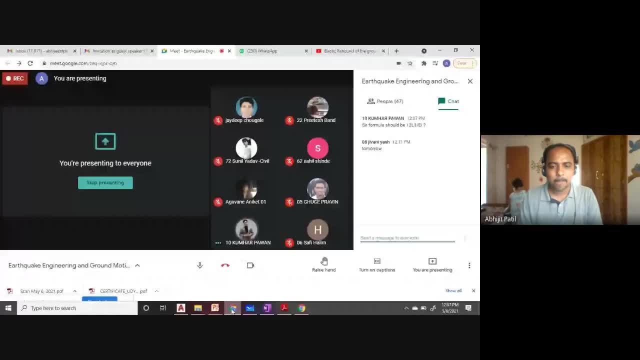 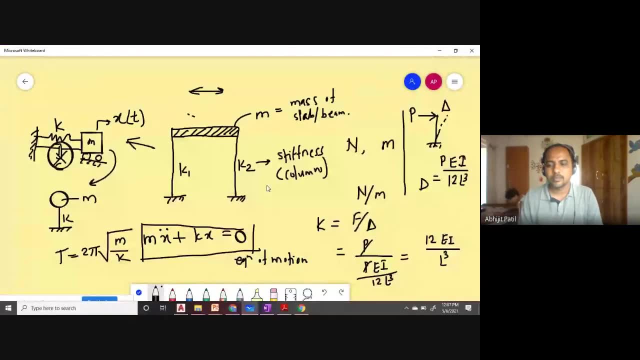 Right, Yes, sir, Just a second. Yes, yes, yes, It's wrongly written. It should be 12 EI by L cube And the K formula will become: I will just correct this. Thanks, Kumar, And this is not D. This is sorry. this is delta. 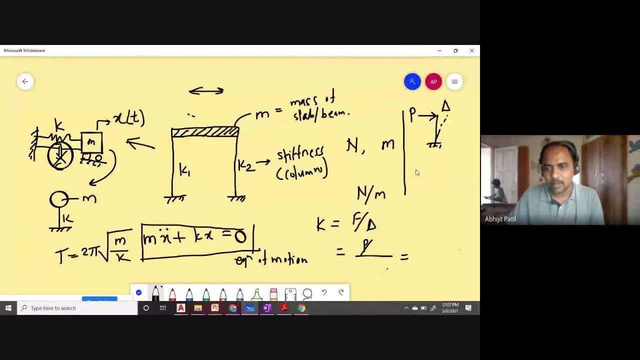 It looks like D: Yes, So it is 12 EI by L cube. Yes, youtubecom. All right, The K should be actually 12 EI by L cube. So here it is actually PL cube by 12 EI. I hope I'm correct this time. 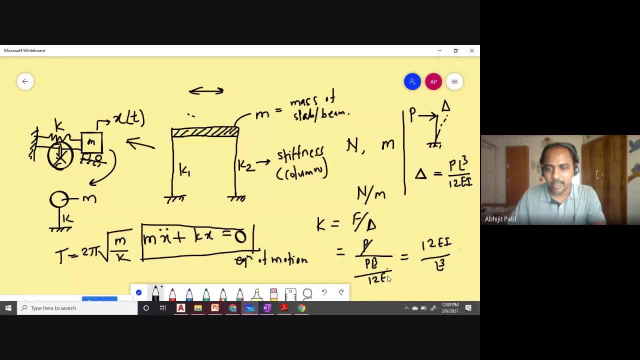 This is PL cube by 12 EI. And if you simplify it will become the stiffness of the dummy uh column and this numerical uh, this cantilever column, will become 12 e high by lq. okay, so if you have written uh, can we make this correction? 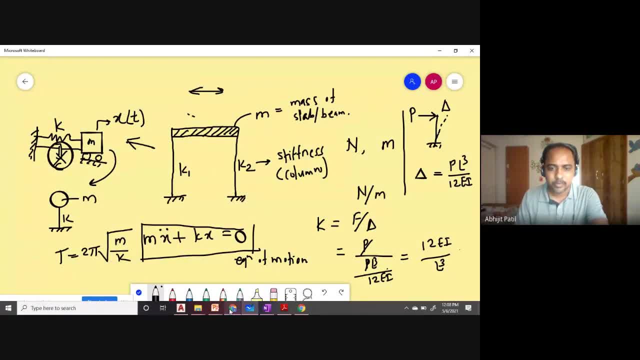 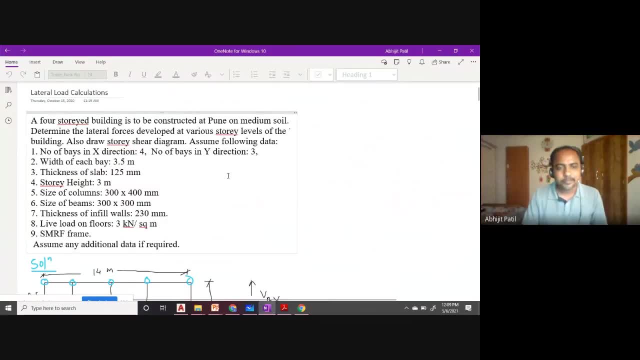 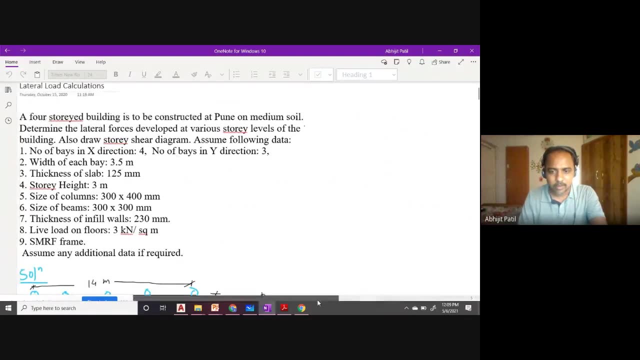 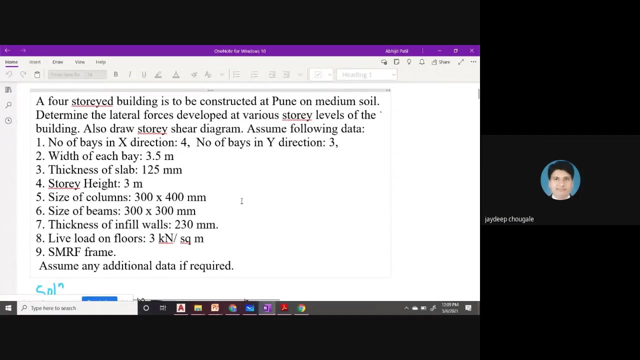 okay, so, uh, what we will do, we will just, uh, we will just write down this numerical. okay, i hope it is visible. we will. okay, i will write down this question. okay, i will just dictate slowly, uh, paddling, you can write, because, whatever we have learned, now it is time to apply this, because what is our ultimate? 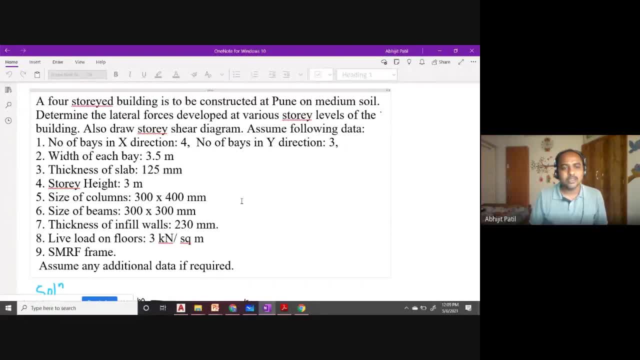 aim. we had to estimate the force coming on the structure. that is what is ultimate aim of this unit. okay, so this background was for that. again, in addition to this you will refer is 1893. i have shared that soft copy with chau glacier and requested him to share the same with you. it is. i will also share the link because, if you require, 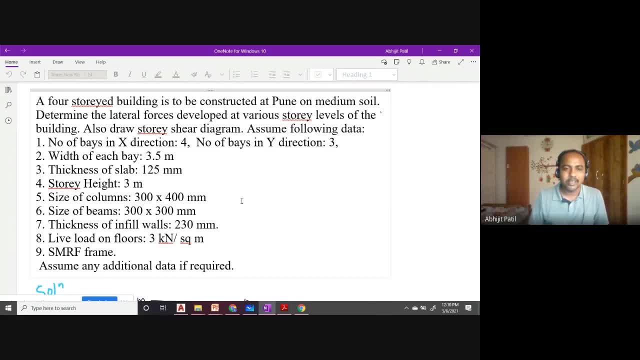 any other ice codes. those are available on that link free of cost. only thing is you have to register there. okay, so we will. with the help of this example and with the help of is 1893 guidelines, we will try to uh see how earthquake forces are calculated coming on a structure. okay, so this is. 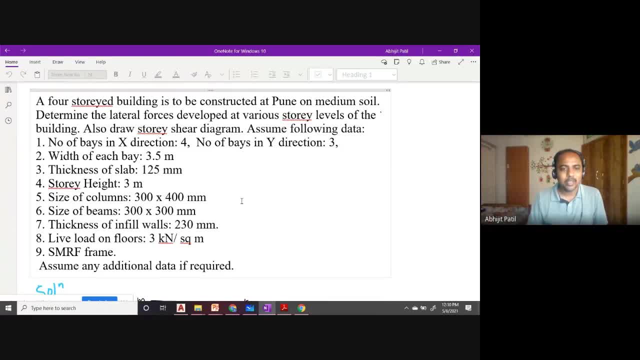 a typical example. you can write this example. i will just detect slowly a four storage building. four storage building is to be constructed. is to be constructed at pune on medium soil. at pune, on medium. determine the lateral forces developed. at pune, on medium. determine the lateral forces developed. 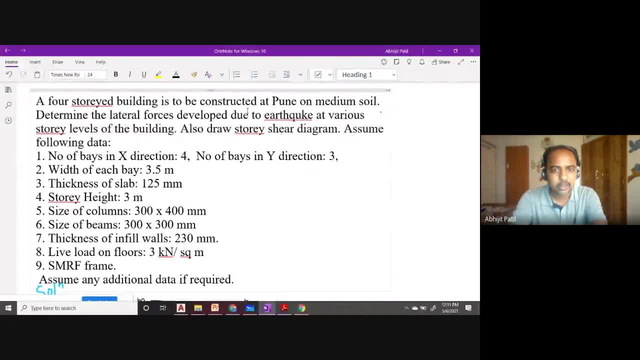 due to earthquake is to be mentioned, due to earthquake at various story levels of the building, at various story levels of the building. also draw story shear diagram. also draw story shear diagram. assume, assume following data. assume following data: so one to nine, few points are given. so number of bays in x direction: 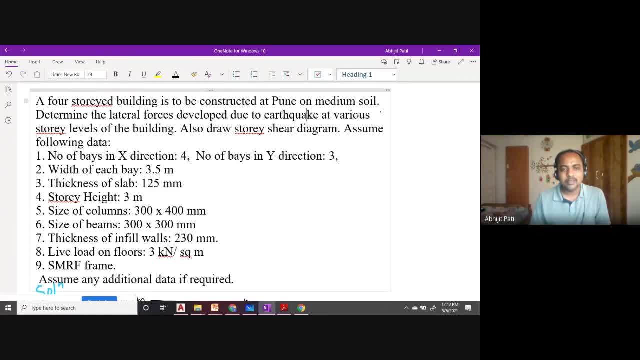 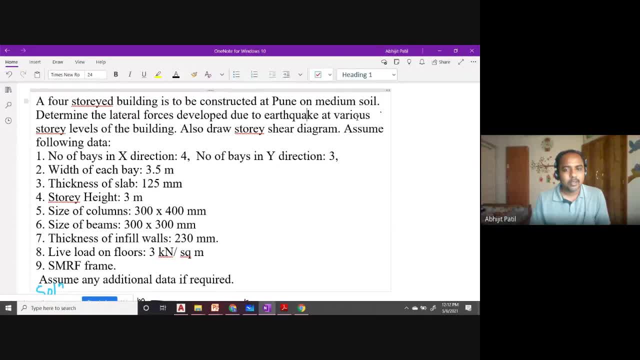 number of bays in y direction: three. width of each bay: 3.5 meter. thickness of slab: 125 mm. width of each bay: 3.5 meter. thickness of slab: 125 mm. wrote of slab thickness of slab 125 mm, Then story height: three meter. 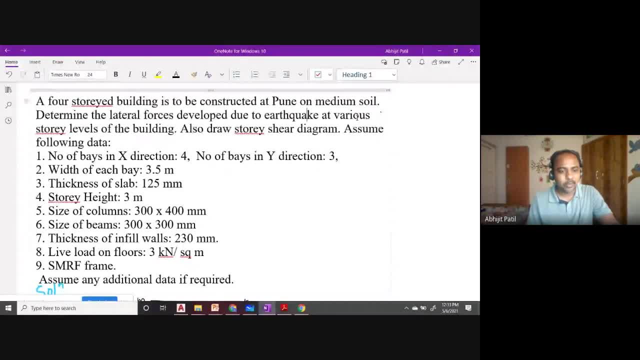 Size of columns: 300 by 400 mm. Size of beams: 300 by 300 mm. Then thickness of infill walls: 230 mm. Infill means partition walls. Okay, Live load on floors: three kilonewton per square meter. 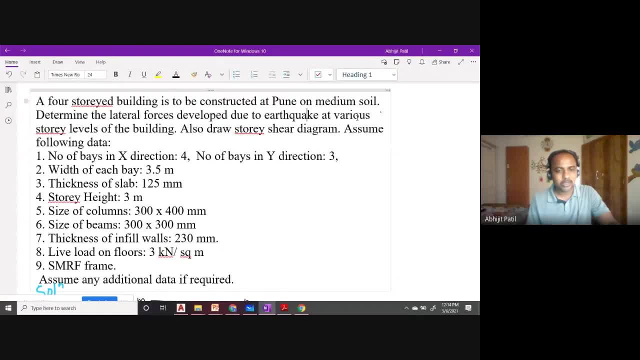 And SMRF frame. What is SMRF? That you will see when we are solving the problem. Assume any additional data if required, Okay, Okay, So number of stories is not mentioned here, but a figure is given, So sometimes number of stories will be mentioned. 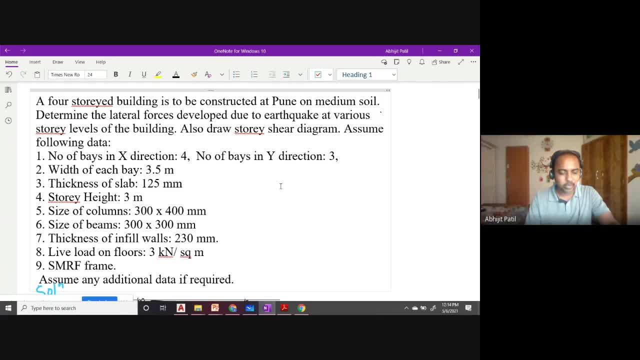 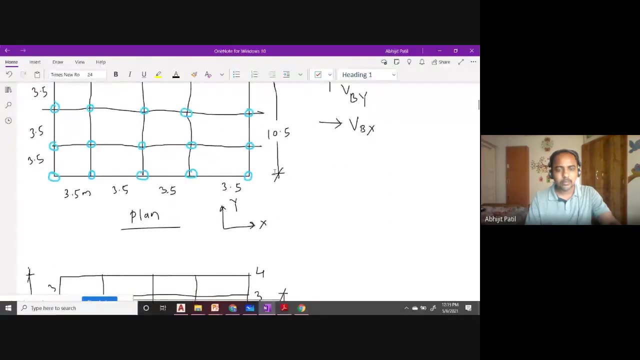 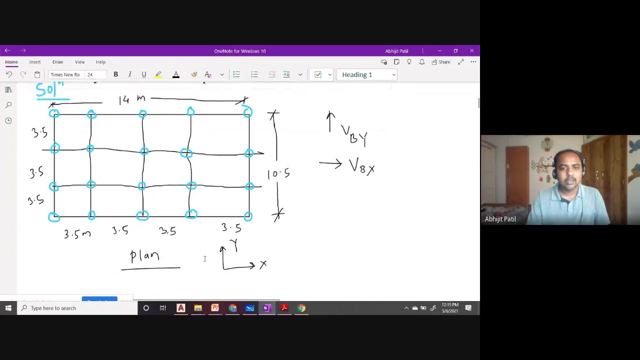 Sometimes, with the help of figure, we will get the input data. Okay, So in plan this building looks like this: In X direction four: base one, two, three, four. In Y direction three: base one, two, three. 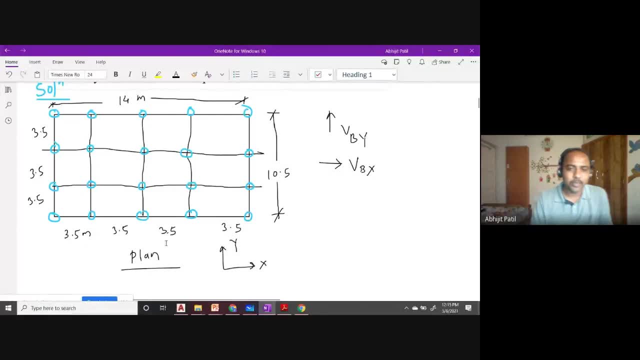 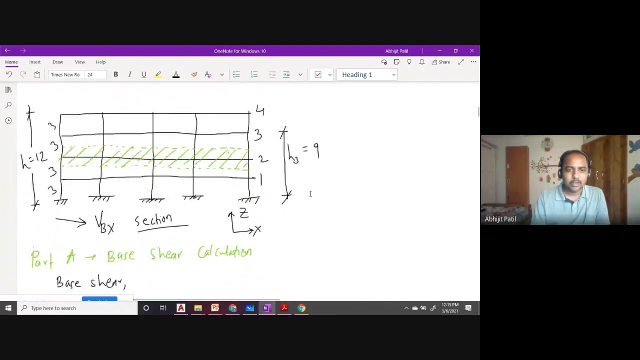 Width of each base: 3.5 meter. So total length is 14 meter. Total here length is 10.5 meter. So center of, at center of each junction, we have our columns placed And this is sectional elevation. 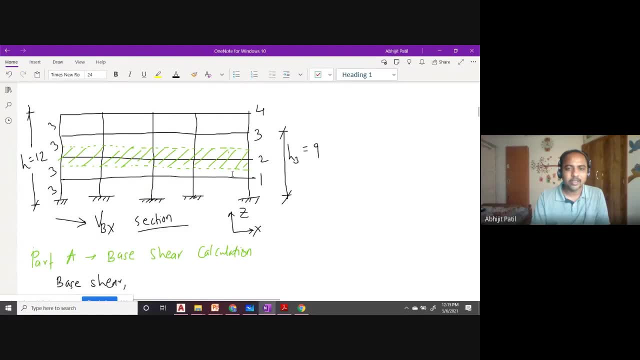 So don't just write the hatch part, Just show the number of base, because this is in X direction. So total: 14 meter And number of stories: one, two, three, four. So total height is 12 meter. 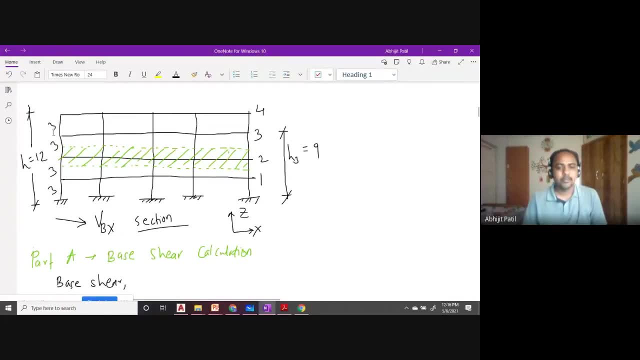 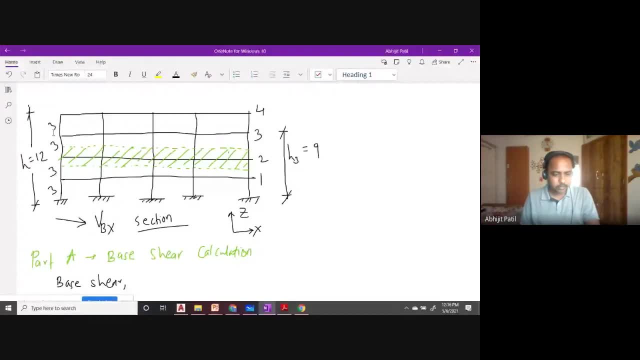 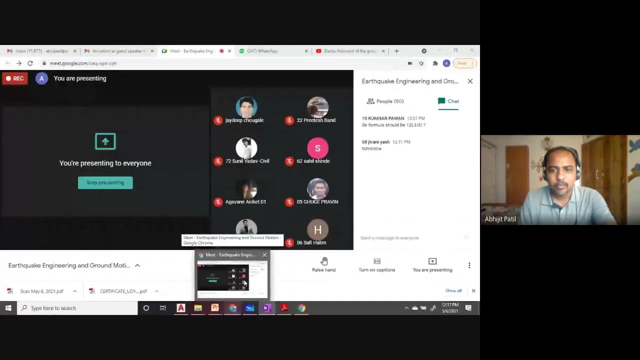 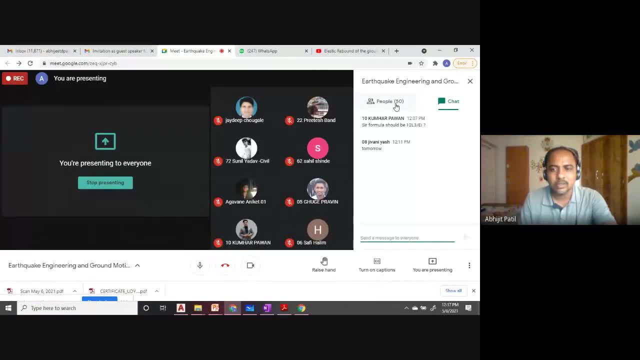 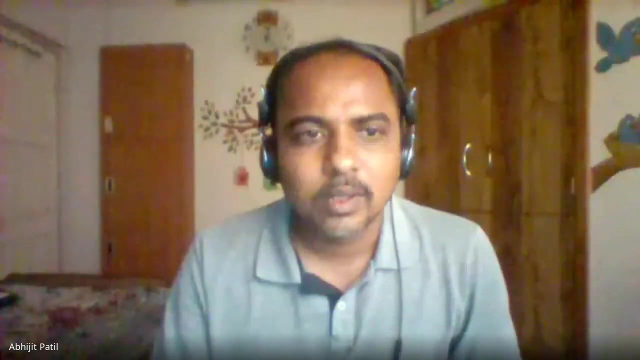 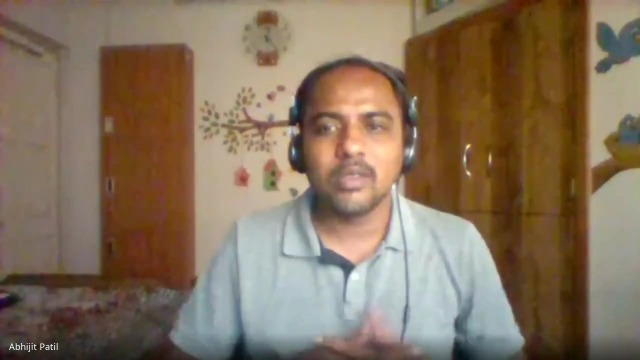 Or you can convey your questions later on. If you find something that you have not understood, you can convey your questions to Chowklesa. We will address it tomorrow. Shall we stop Chowklesa? Yes, sir, Okay, so tomorrow a few instructions for students. 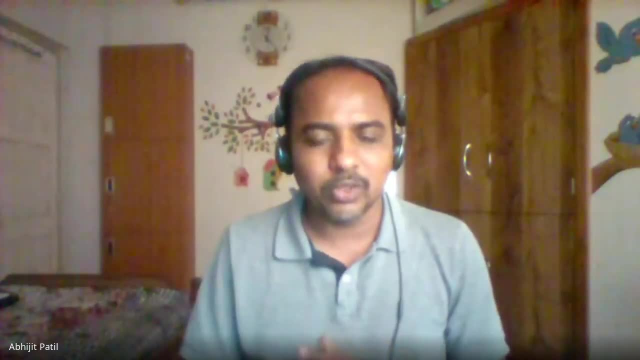 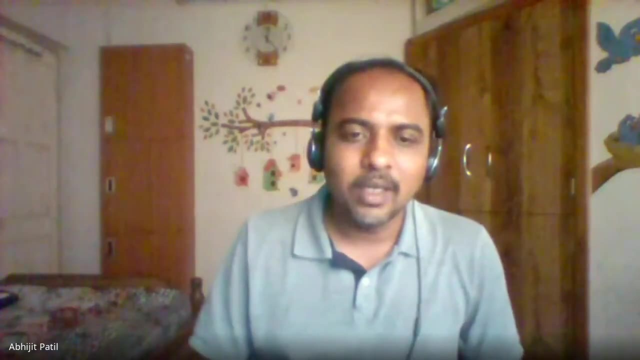 That 1893, which sir will share with you. Be ready with that Hard copy or soft copy, in whatever form you have. And another thing: Calc. So we will require a calculator also, So that we can you do it hands-on. 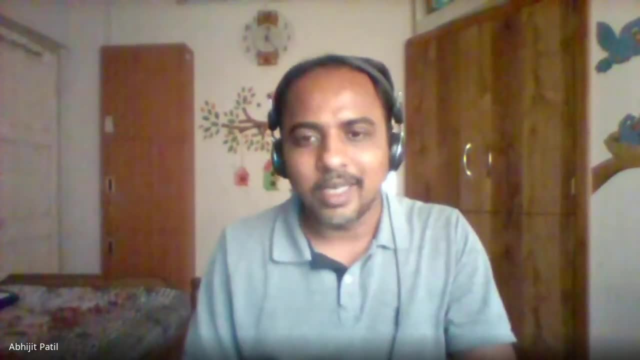 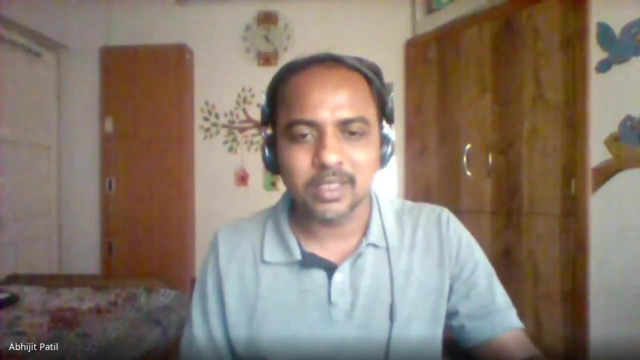 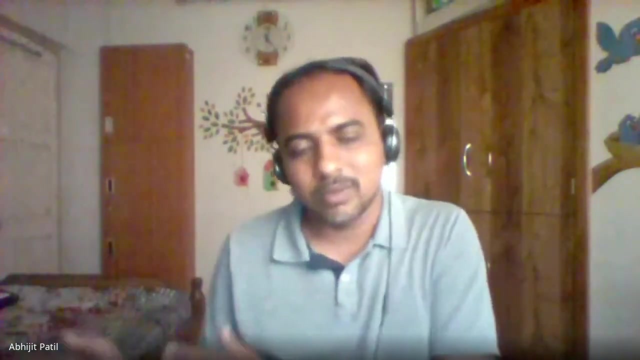 Okay, then only you will be able to understand what exact steps are to be followed. You should do it on your own. So we will be discussing step by step, And there will be a few more concepts that also we will discuss whenever that concept comes, when we are solving the numerical. 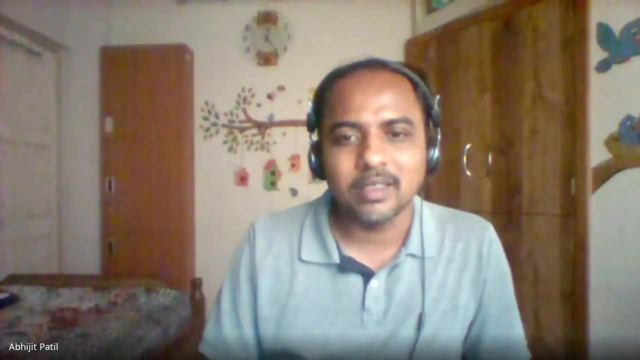 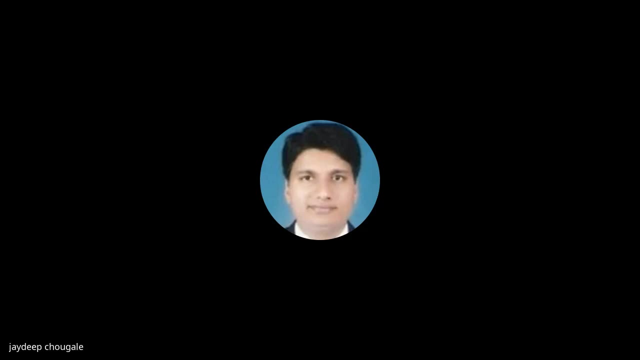 Okay, so we will stop now. Students can leave the class. Bye. Okay, thank you, sir, for your sharing your vast knowledge of earth engineering with our students. Tomorrow also, we will continue this topic. Okay, at 10.30, sir.